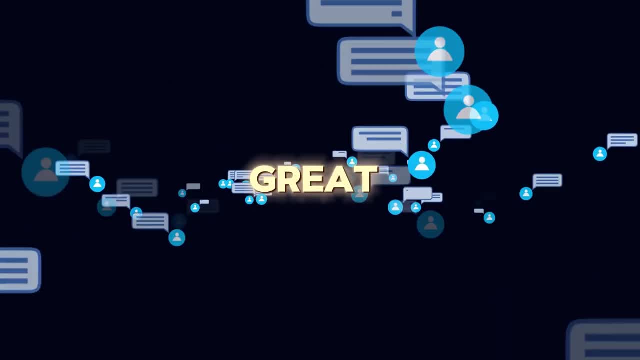 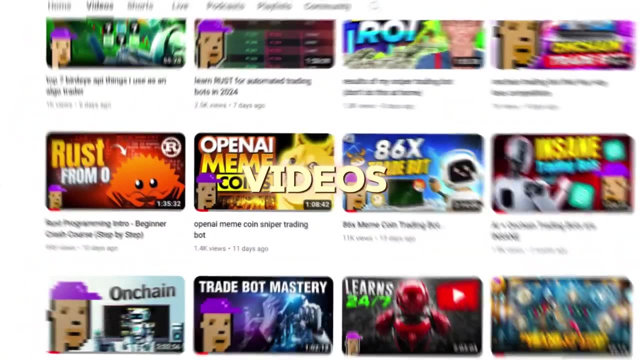 that review and I think this is gonna be great. I think it's gonna be great because now, once these videos are released, or once you're watching this, I guess there should be videos in the past that show the whole journey. and I'm learning Rust because I have this Solana. 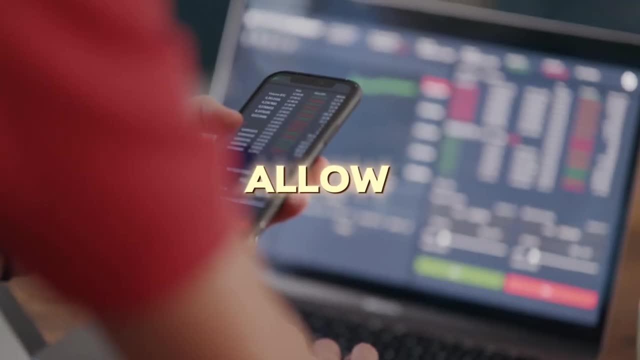 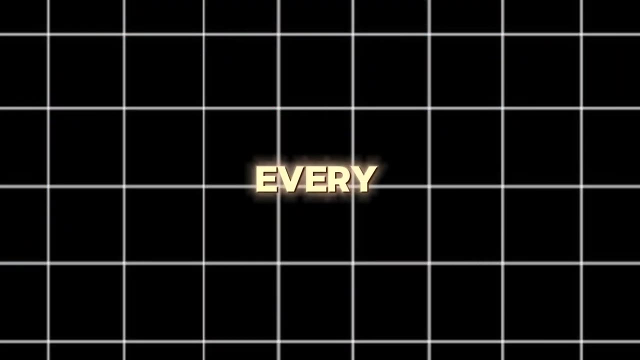 Sniper that's doing fairly well for me and this is gonna allow me to essentially sort through the Solana blockchain. on top of that, you know I'm an algorithmic trader. every single day, I automate new trading systems or update old trading systems or backtest trading systems, and I think it's gonna 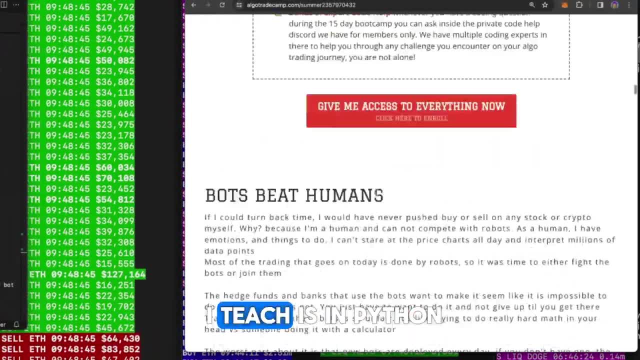 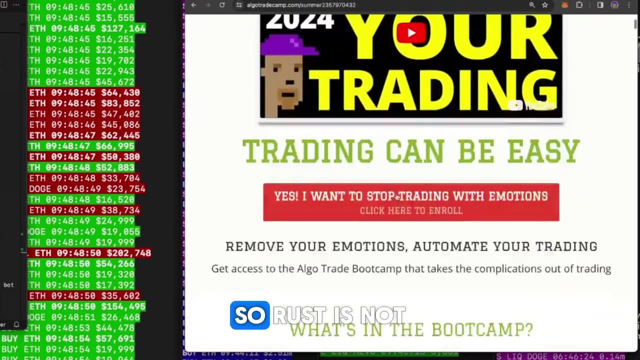 be super nice to have a faster language. that being said, everything I teach is in Python and I think Python is going to be- or I know Python is gonna be- my go-to language for the rest of the time here. so Rust is not a requirement by any means, so don't worry about it. the bootcamp still shows how to. 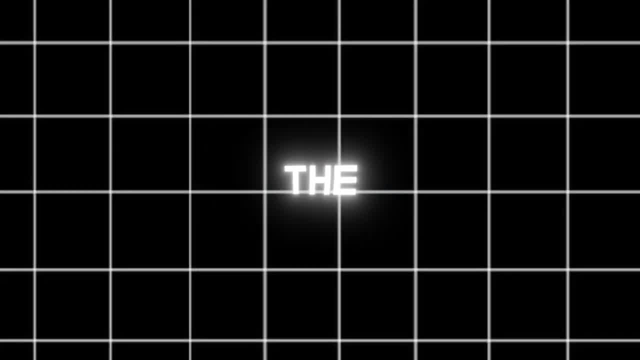 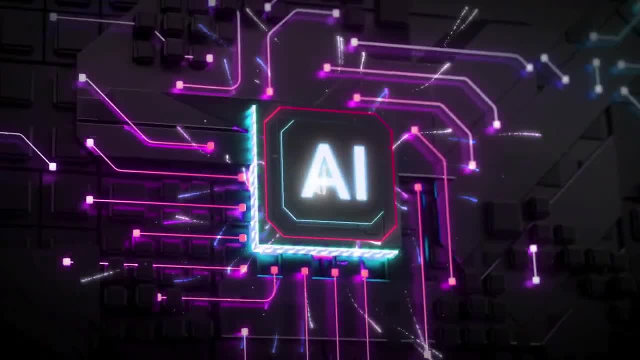 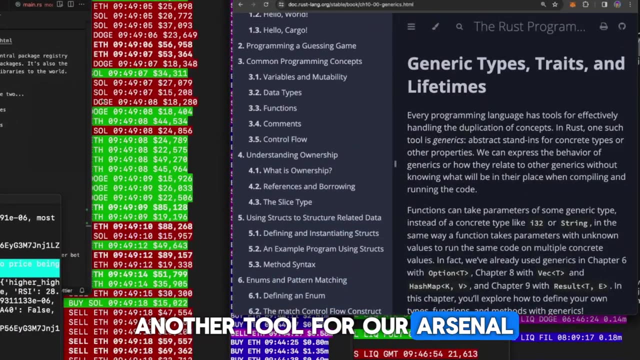 code in Python, because I believe Python is the way to go when you want to algorithmic trade, automate your trading, build trading bots, be able to back test, use AI. it's like the best language in my opinion, but we're here on Rust and we're just learning another tool for our arsenal, so 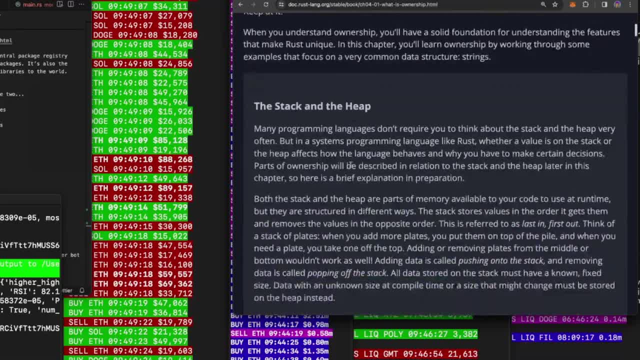 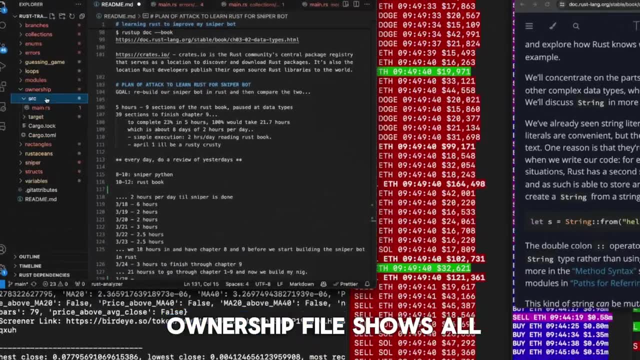 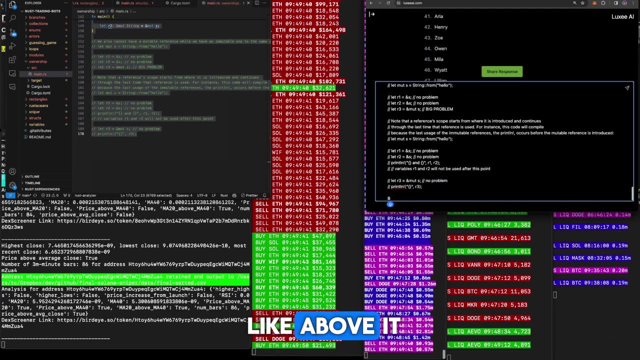 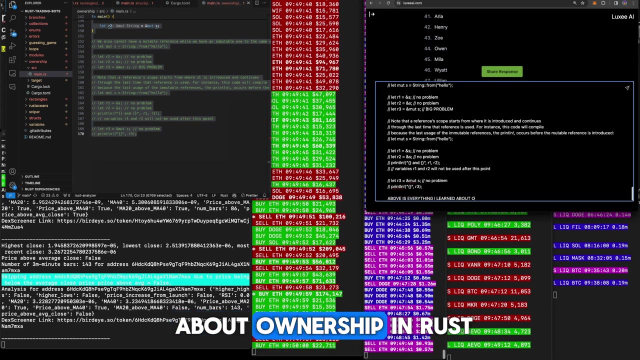 understanding ownership. this was a tricky topic, so what I want to do here is: if I have a ownership file, I do, and this ownership file shows all of the things that we learned. it's 171, so let's go ahead on Luxy and be like above it. oh my god, I can't type. above is everything I learned about ownership. 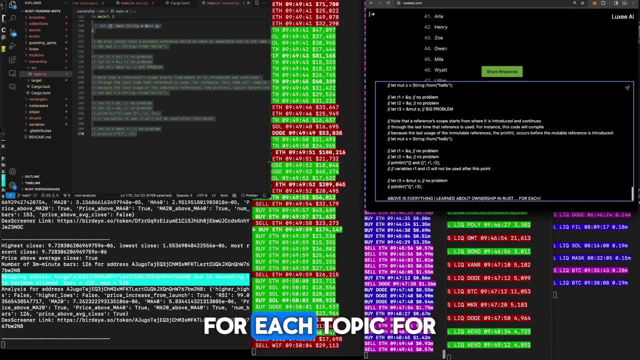 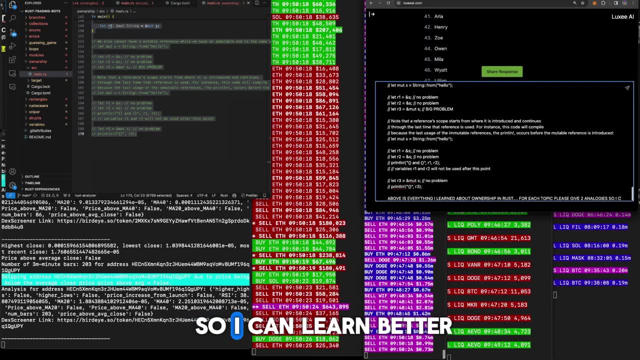 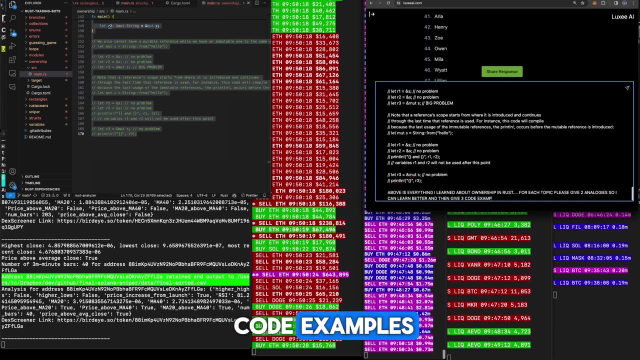 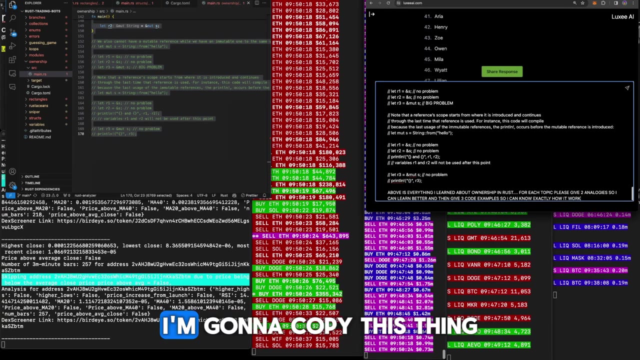 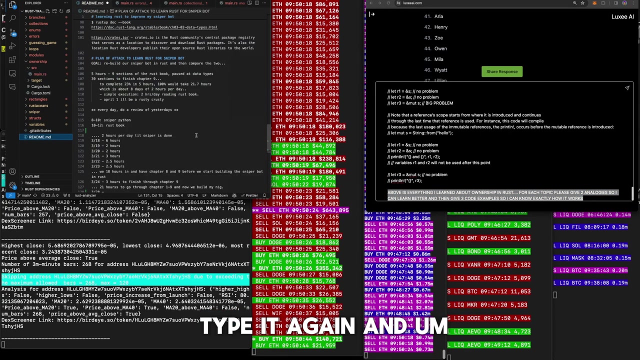 in Rust for each topic. for each topic, please give two analogies so I can learn better, and then give three code examples so I can learn and know exactly how it works. I'm going to copy this thing because then I can just use it. I won't have to type it again and um, this is going to be awesome. 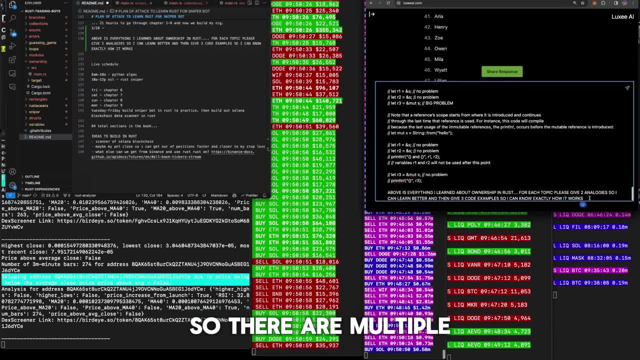 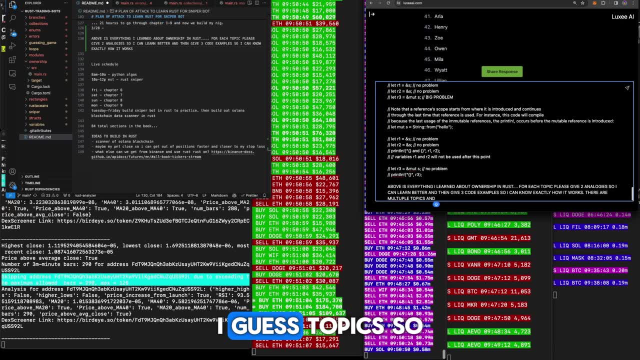 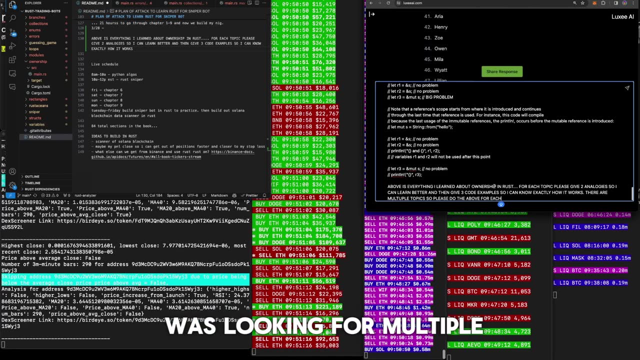 because we're gonna really have a great review. so there our, there are multiple topics and and- um, what would you call it? yeah, I guess topics. so please do the above for each. it's concepts, that's the word. I was looking for multiple concepts for each. I'll copy this over, and then Luxy, our little shorty over here, will go ahead and tell us exactly what we need to do. scenario: 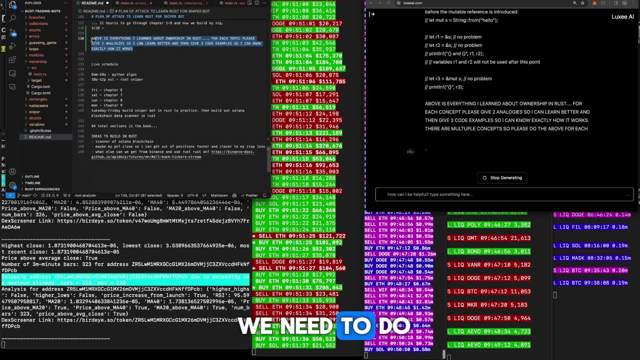 to do what we need to learn: troubleshooting, bait東西, the ownership in rust and excuse my point, but I'm gonna sit down and get into this and learn how to run this business itself literally every time. you know how important that thing is. you're entering something when you move to the software and you're constantly leaving the company. you're getting a want to work with a new. 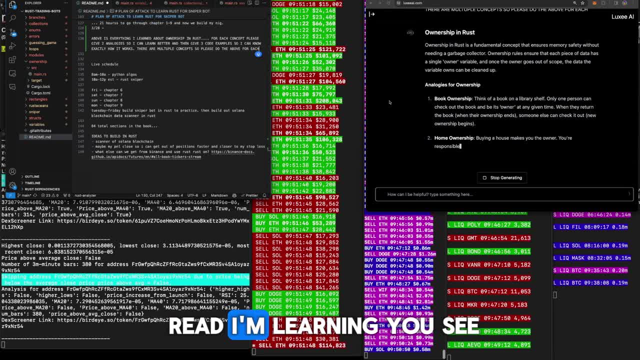 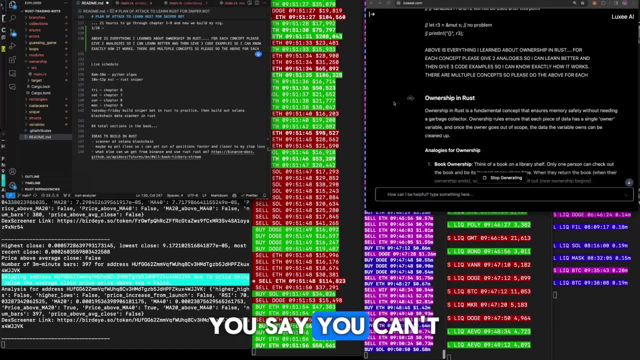 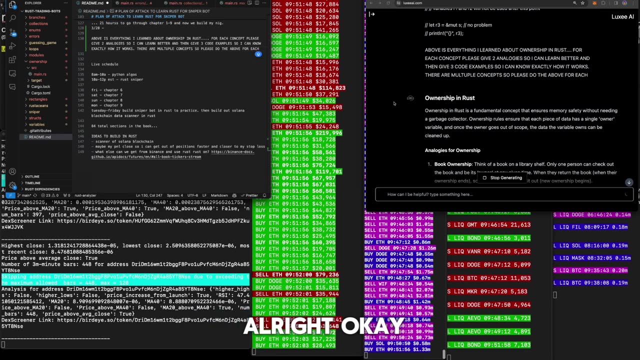 my poor reading, but i'm learning how to read. i'm learning, you see, you remember what i was talking about just a second ago, though i i was talking about how, like when you say you can't do something, your subconscious is like: oh sick, i can't do that. so, although i'm a bad reader, all right, okay, i need. 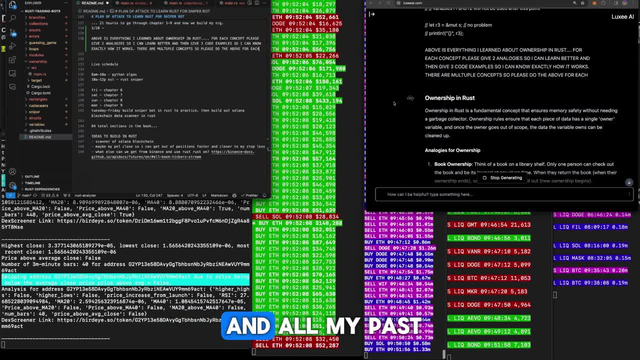 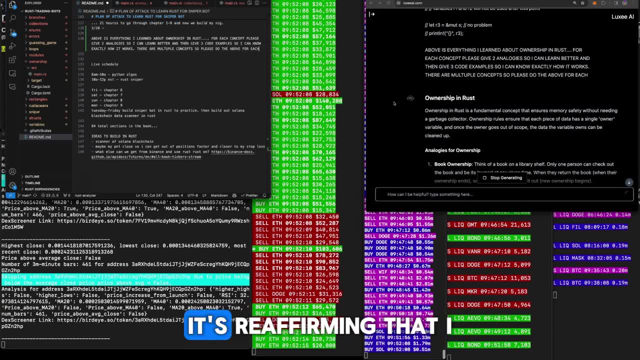 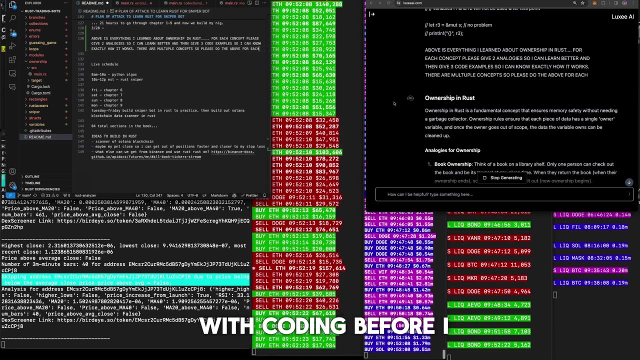 to change that, although in the past i used to not be able to read and all my past videos like: i can't read. sorry, i can't read. that's just that. what that is doing to my subconscious is it's reaffirming that i can't read. so i need to change that, just like i changed with coding before i was like: oh i. 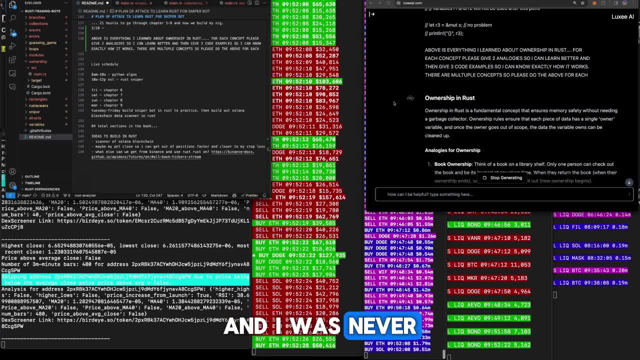 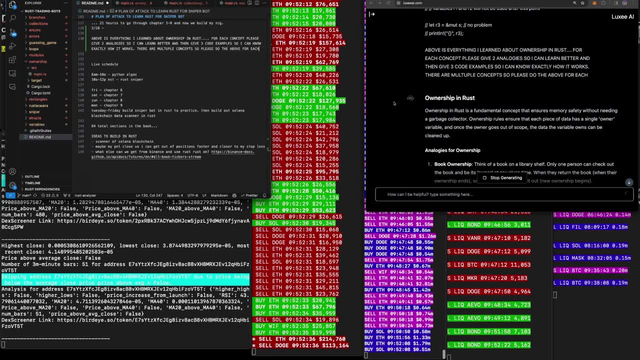 can't, so i can't code. i will never be able to code, and i was never able to code because i said i couldn't code. but once i was like you know what this dude can do? it, i can do it too. that's when i learned how to code. so while you know, in the past i believed i couldn't read, now i'm gonna change. 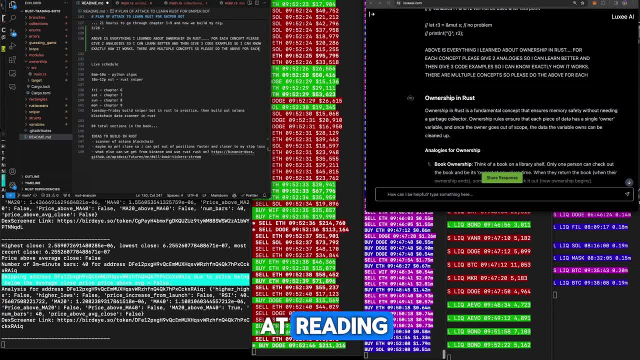 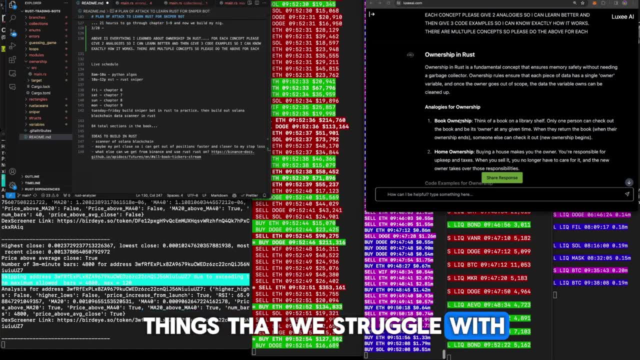 that i'm gonna change that. i'd be like i'm actually getting better at reading. i'm getting, i'm getting real good at reading. so you know, we all have our insecurities. we all have our things that we struggle with. we all have our things that. 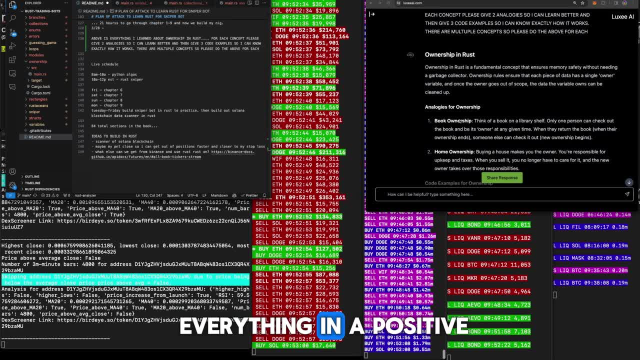 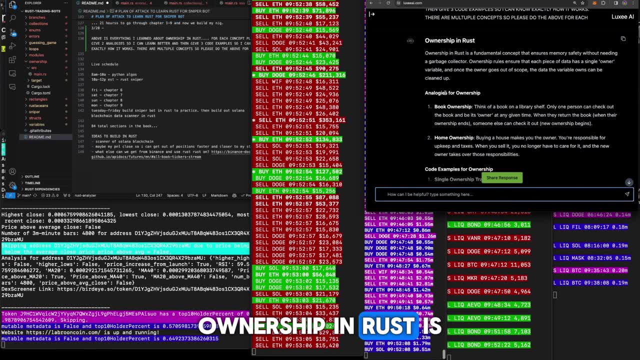 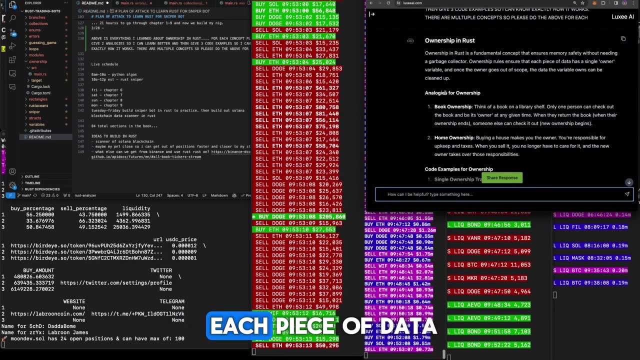 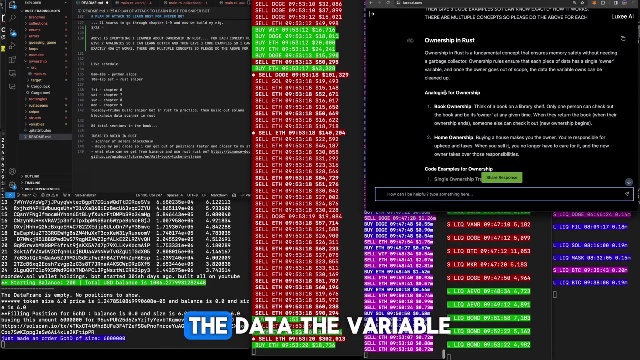 might not be perfect, but try to put everything in a positive light and you can do anything. so stick with me while i read this so elegantly. ownership and rust is a fundamental concept that ensures memory safety without needing a garbage collector. ownership rules ensure that each piece of data has a single owner variable and, once the owner goes out of scope, 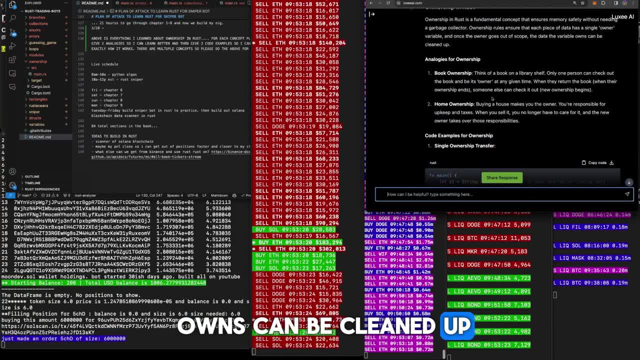 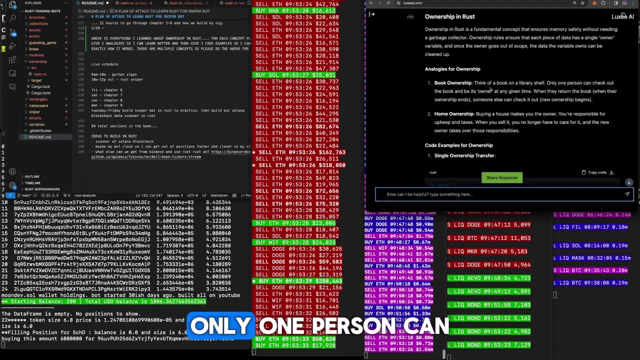 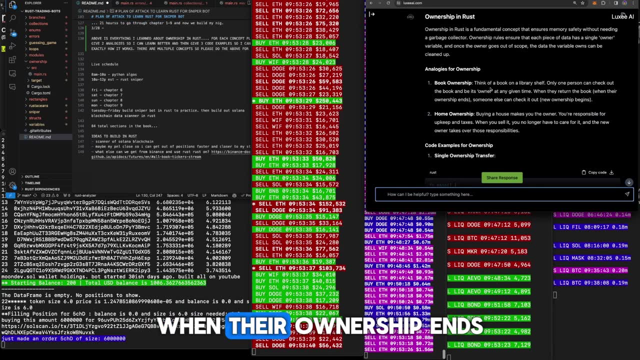 the data, the variable owns can be cleaned up. so analogies for ownership: book ownership- think of a book on a library shelf. only one person can check out the book and be its owner at any given time. when they return the book, when their ownership ends, someone else can check it out. the new: 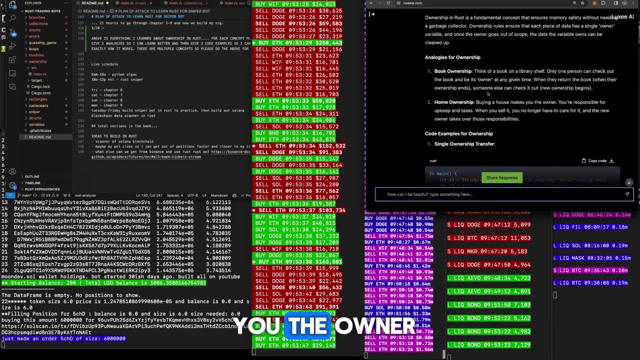 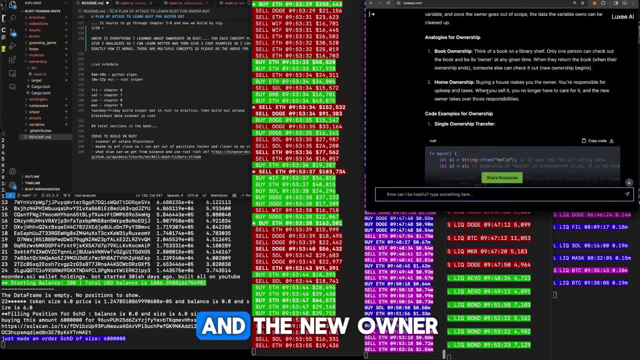 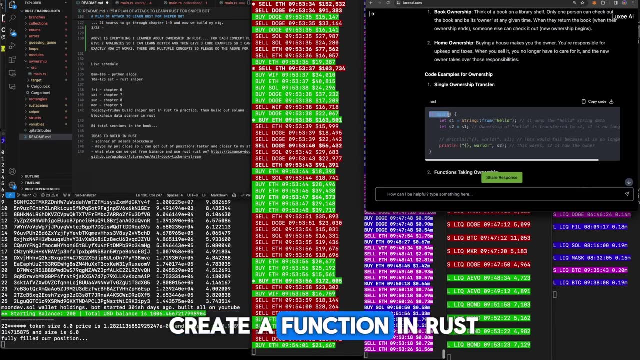 ownership begins. so home ownership buying a house makes you the owner. you're responsible for upkeep and taxes. when you sell it, you no longer have to care for it and the new owner takes over those responsibilities. so let's look at how ownership works here, so you can see. this is how you create a function. 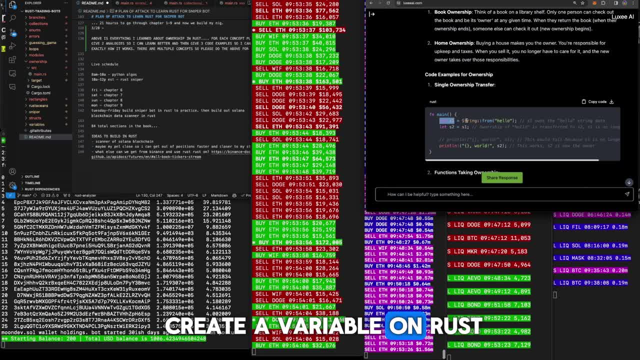 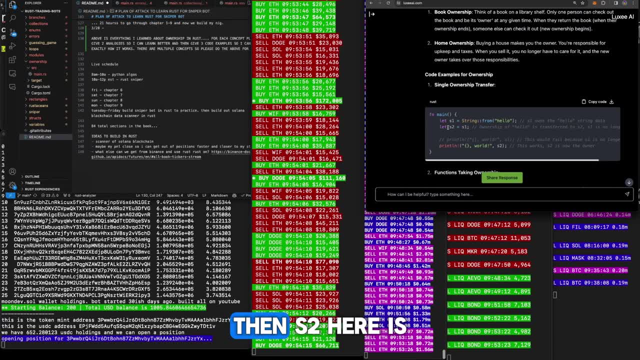 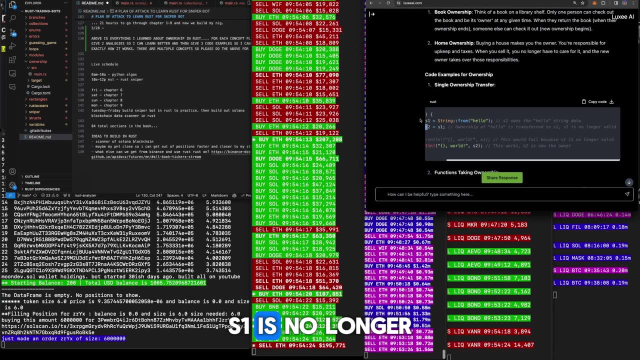 in rust. this is how you create a variable on rust. the variable would be a string from hello. s1 is the owner of that hello string data. then s2 here is set to s1 as a variable. ownership up of the hello is transferred to s2. s1 is no longer valid because it's 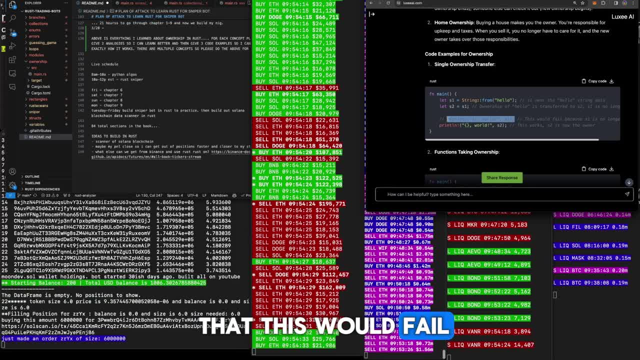 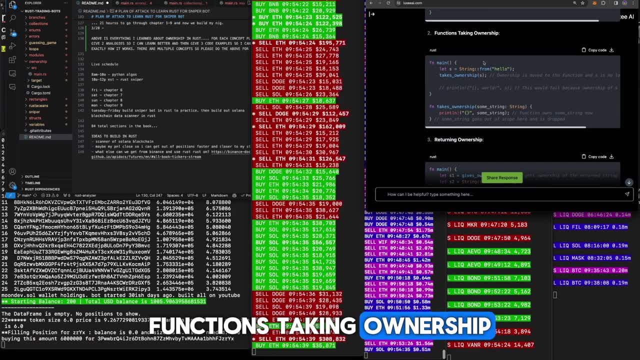 been transferred and there's only one owner, and you can see that this would fail. this line would fail because it's trying to print out s1, but s2 is the owner now, so function functions taking ownership. so you can see this: how you make a function and then this is the mute is actually how you make. 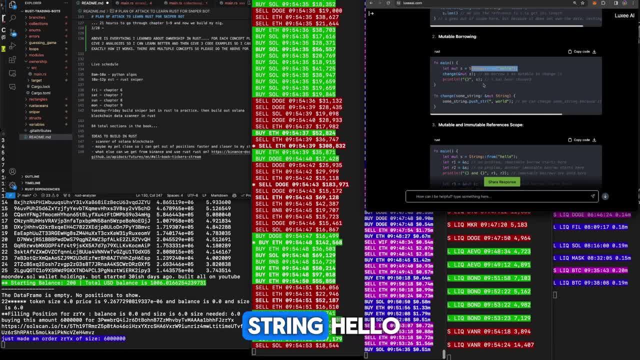 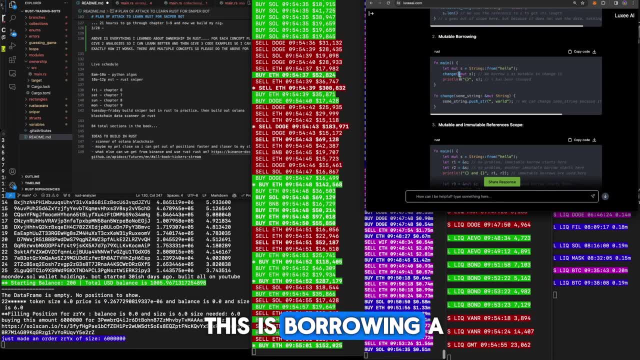 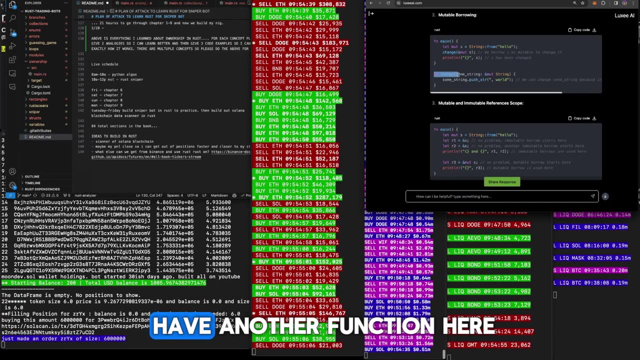 it a mutable, changeable function. so s again is from the string hello, then change. we borrow as a mutable to change. so you see this: this is borrowing a changeable s and then we can print out: fn, change. so we're going to have another function here and it takes in a chain borrowable, changeable. 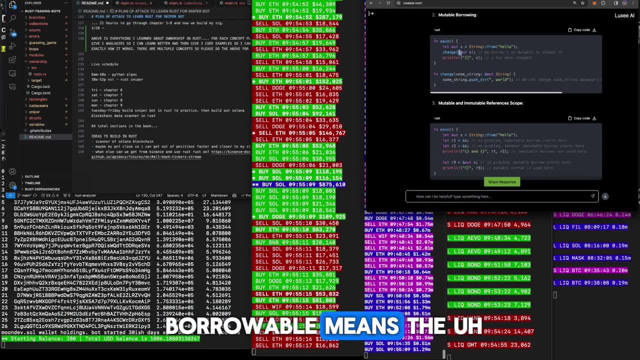 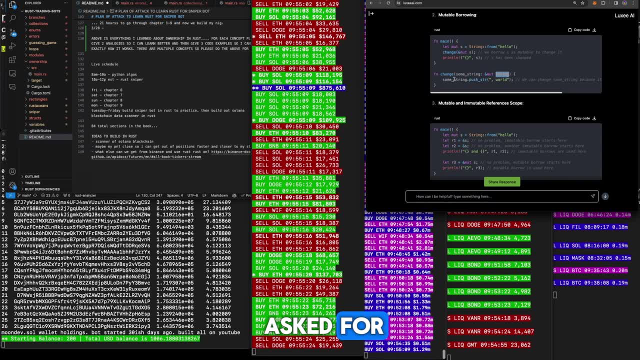 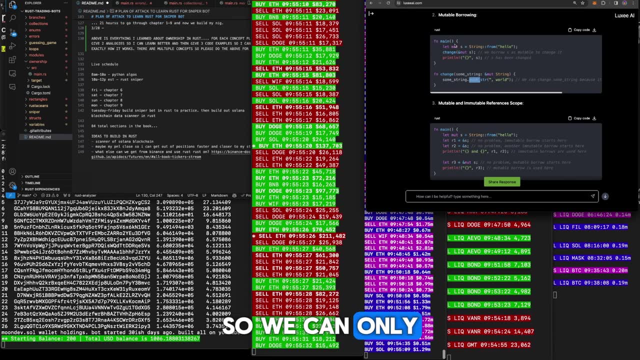 string. so here we're. the borrowable means the, uh, the and sign, and changeable is mute and then s. so we pass that in just like it asks for, and then push string means we can change the string because it's a mutable reference. so we can only change it because it's a mutable mute. 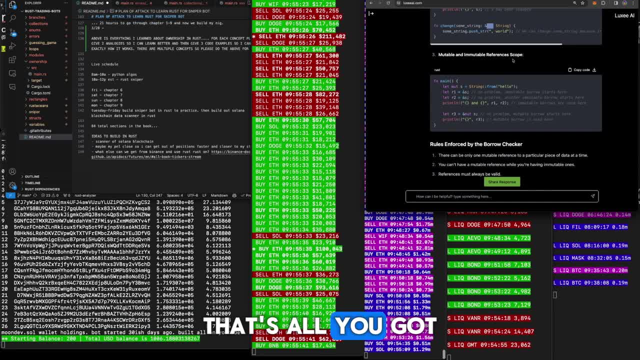 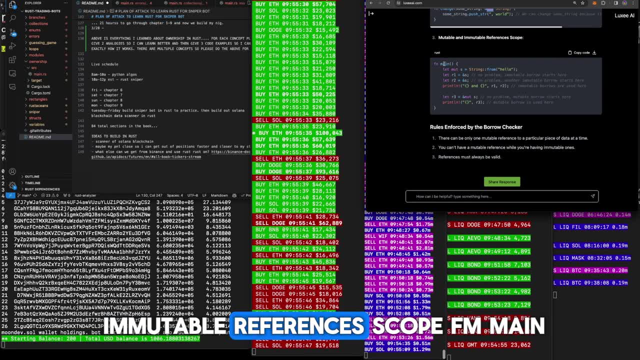 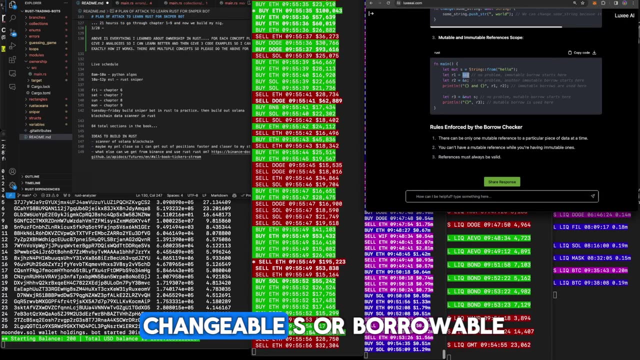 mute, mutable and immutable references. that's all got for me. i put all that code and that's all you got for me, though. anyways, so, mutable and immutable references. scope: fn: main. so you can see: mute is changeable, s equals string. hello, let r1 equals a changeable s or a borrowable, no problem, immutable borrow starts here. 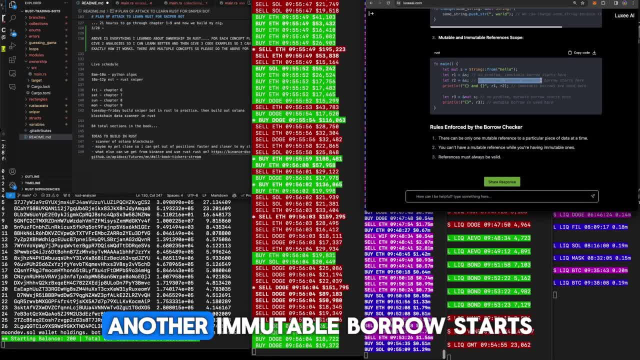 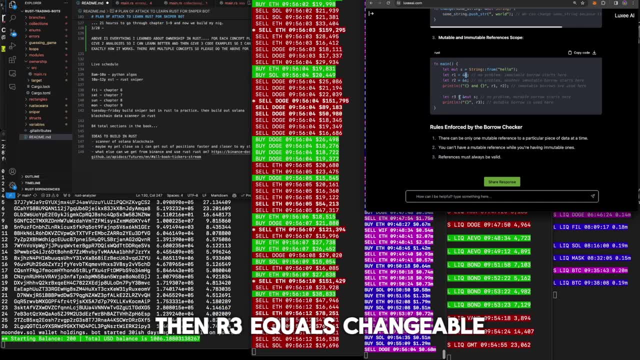 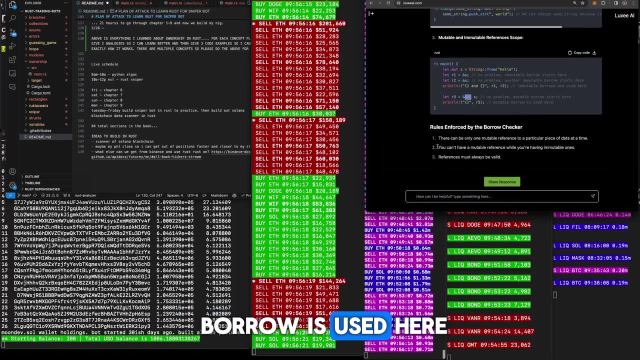 then let r2 equal and s. it's no problem. another immutable borrow starts here, because we're just borrowing it and then we can print out the immutable borrows. then r3 is changeable, mutable s, no problem, mutable borrow starts here. println beautiful borrow is used here. 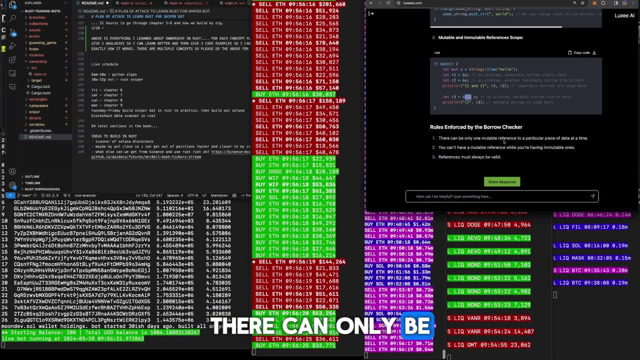 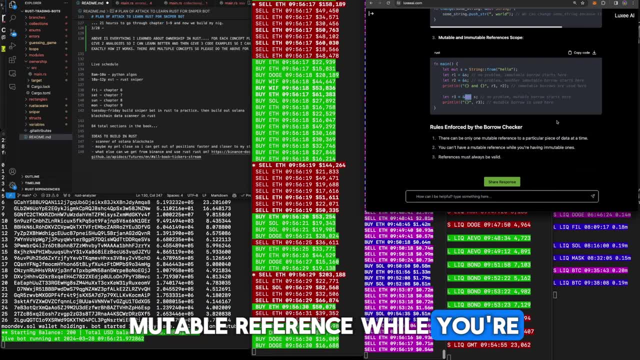 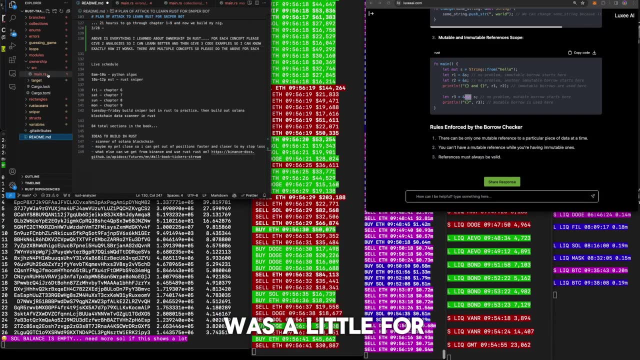 rules enforced by the borrowed checker. there can only be one mutable reference to a particular piece of data at a time. you can't have a mutable reference while you're having immutable ones. references must always be valid. i feel like that was a little for how much code i have here, but let's go ahead and check it out. maybe it was just a bunch of. 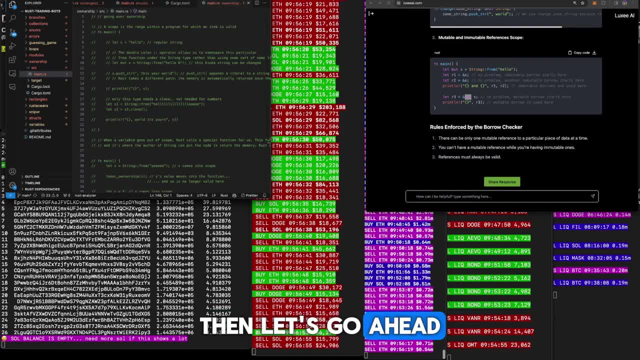 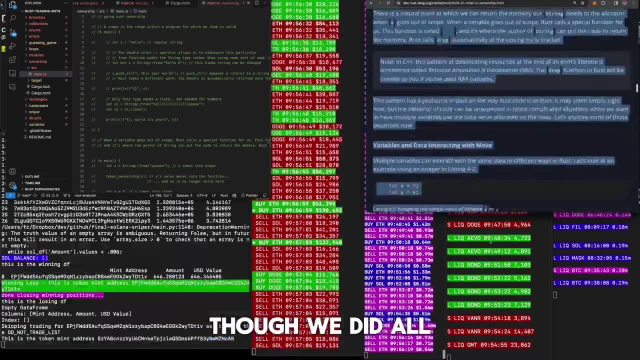 examples of All. right, I guess we're done with ownership, then Let's go ahead and see if there's anything else here. Please do the same thing. but with all this information, I feel like we learned ownership, though We did all of this already in the past vids, I just want to make sure. it's super. 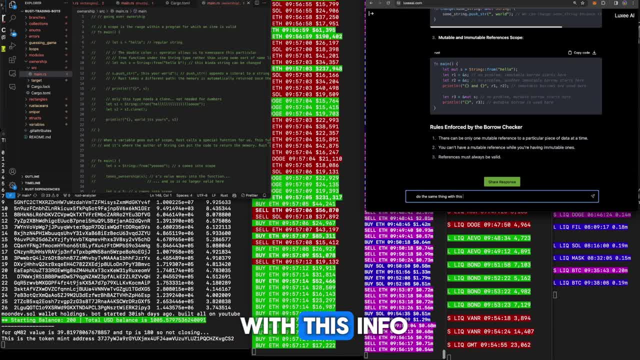 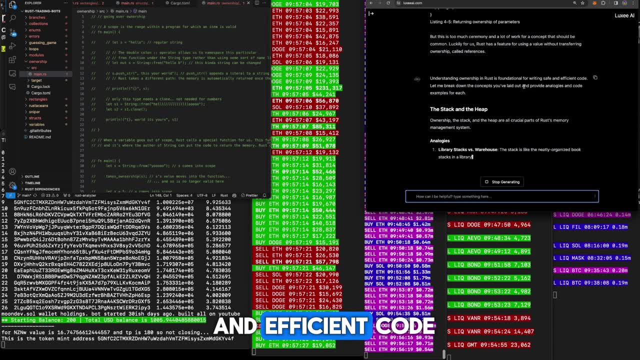 clear. Do the same thing with this info. Just make sure we really understand ownership. Understanding ownership in Rust is foundational for writing safe and efficient code. Let me break down the concepts you laid out and provide analogies and code examples for each: The stack and the heap. 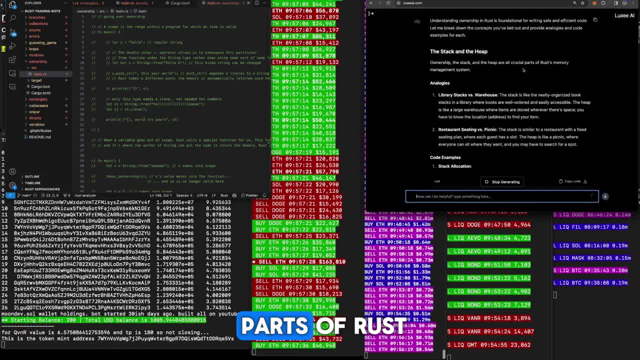 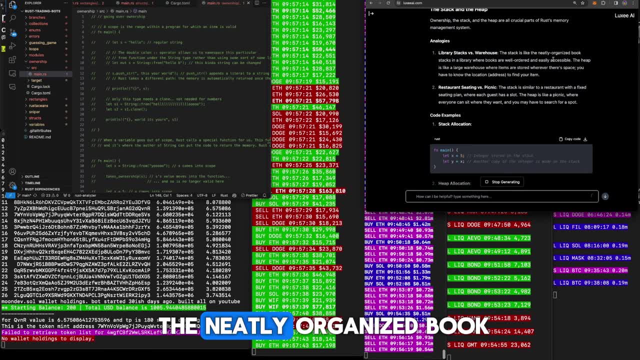 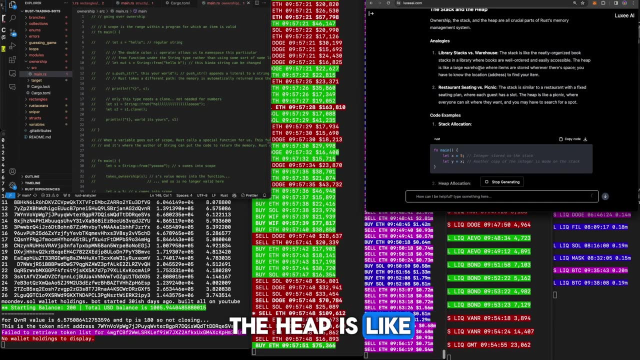 Ownership. The stack and the heap are all crucial parts of Rust memory management. Analogies: Library stacks versus warehouse. The stack is like the neatly organized book stacks in a library, where books are well ordered and easily accessible. The heap is like a large warehouse where items are. 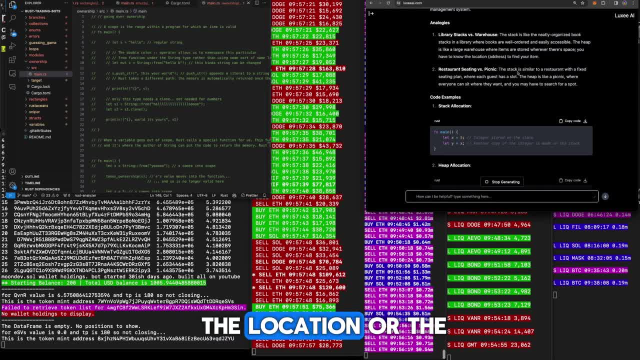 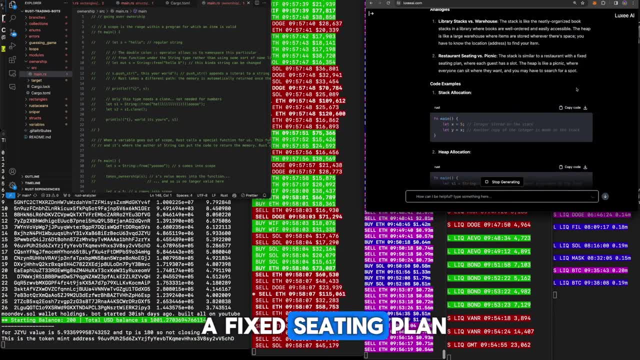 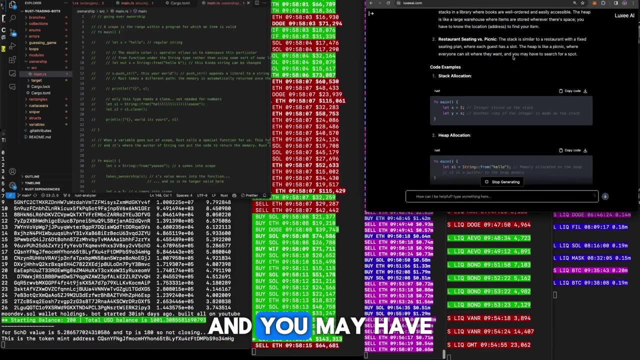 stored wherever there's space. You have to know the location or the address to find them. Restaurant seats. Seating versus picnic. The stack is similar to a restaurant with a fixed seating plan where each guest has a slot. The heap is like a picnic, where everyone can sit where they want and you may have. 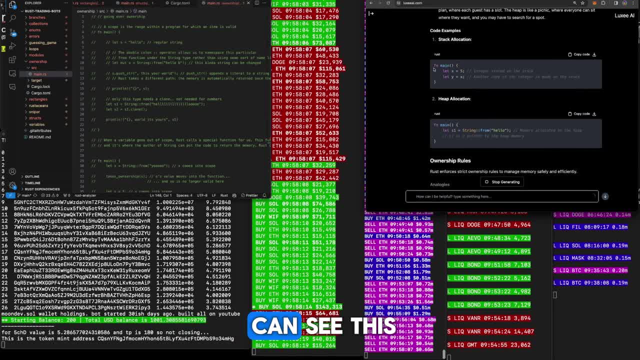 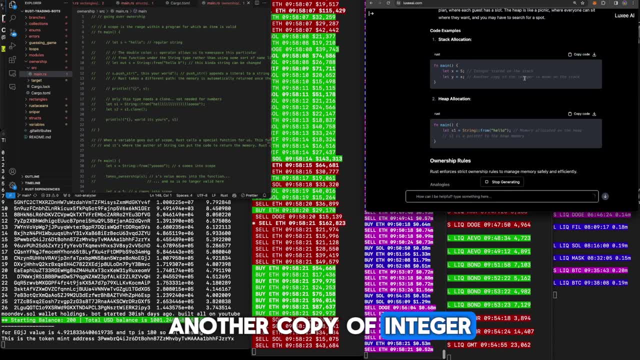 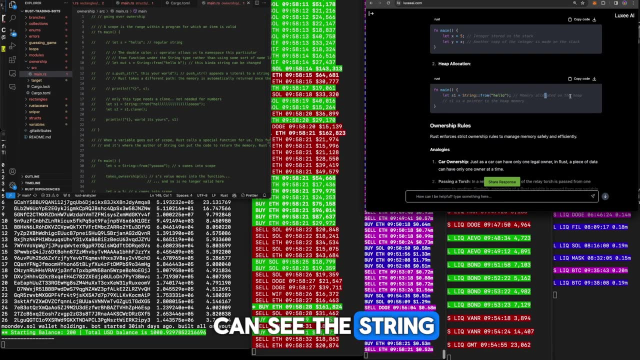 to search for a spot. Stack allocation. You can see this is how you make a function. fn. main Integer stored on the stack would be this: Another copy of an integer stored on the stack would be that Integers are on the stack essentially, Then here you can see this string would: 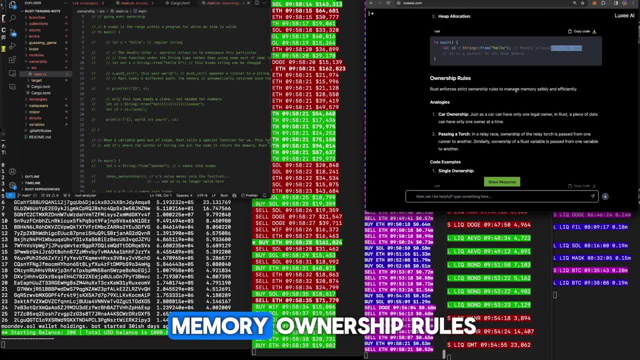 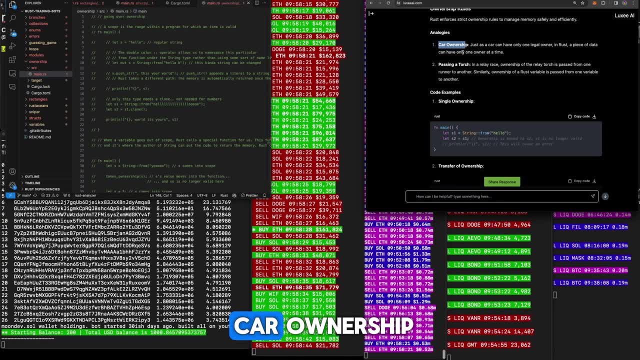 actually be the stack. The stack is the stack. The stack is the stack. The stack is the stack. This one is a pointer to a heap memory Ownership rules. Rust enforces strict ownership rules to manage memory safely and efficiently. Analogies: Car ownership. Just as a car can have only one. 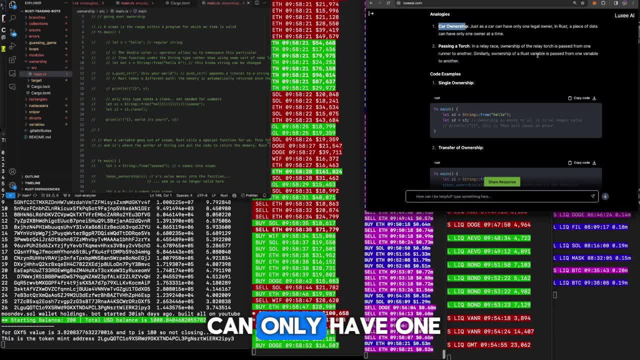 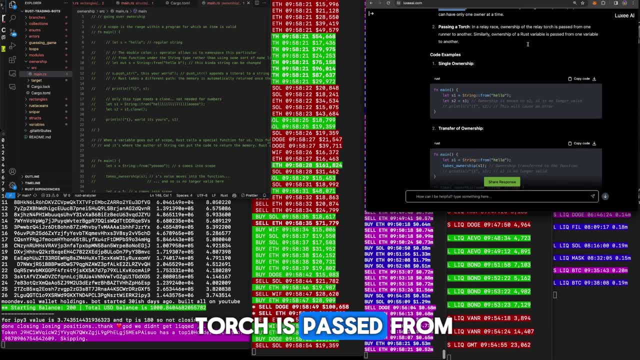 legal owner. in Rust, a piece of data can only have one owner at a time. Passing a torch in a relay race, Ownership of the relay torch is passed from one runner to another. Similarly, ownership of a Rust variable is passed from one runner to another. Passing a torch in a relay race. Ownership of a? 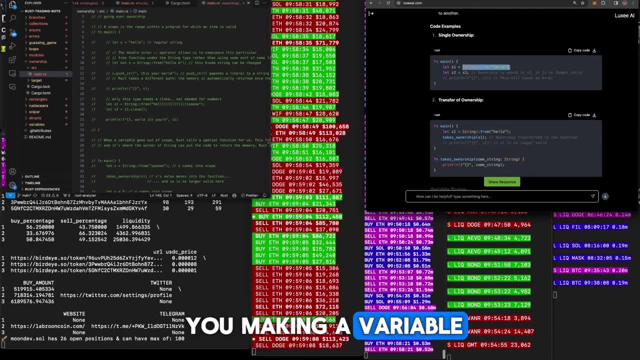 Rust variable is passed from one runner to another. Passing a torch in a relay race, Ownership of a Rust variable is passed from one runner to another. You can see you're making a variable of s1 and then we're saying, hey, we're moving the ownership over. Then again, string of hello and it takes. 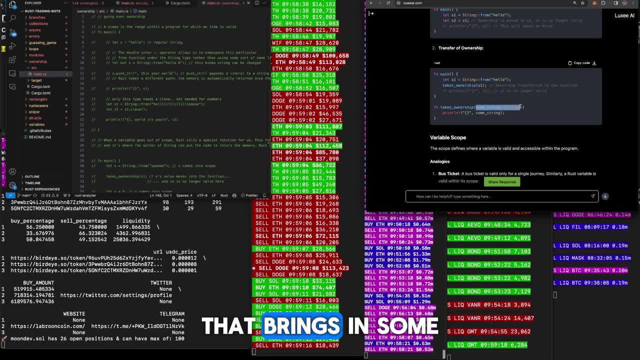 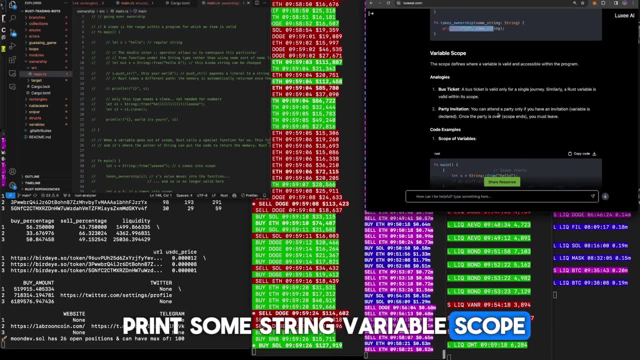 ownership, because we have a function called take ownership that brings in some sort of string and it's this string because it's s1, and you see s1 here, and then we print some string. Variable scope: The scope defines where a variable is valid and accessible in a. 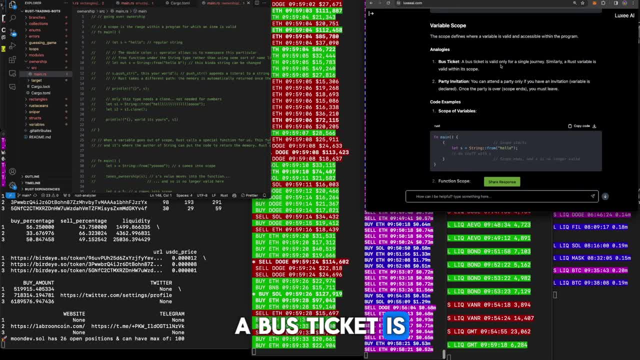 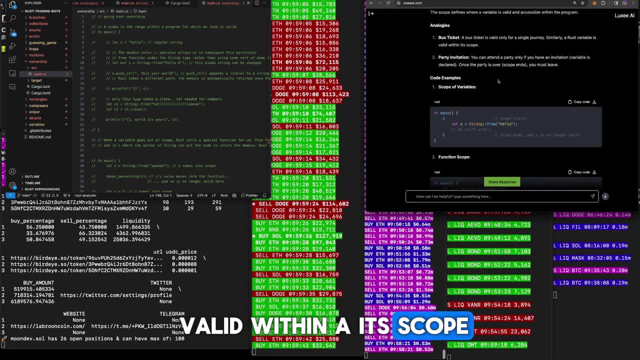 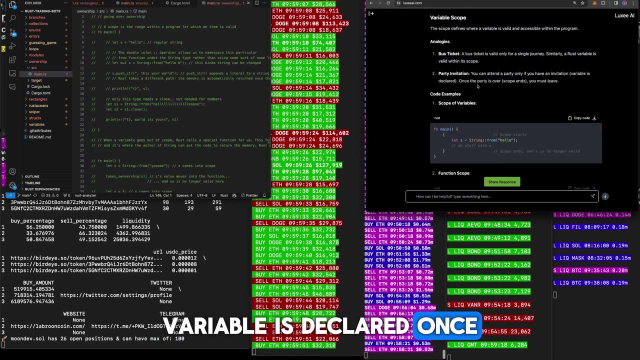 program- Bus tickets. A bus ticket is valid only for a single journey. similarly, a rust variable is valid within its scope. party invitation: you can attend a party only if you have an invitation. variable is declared. once the party is over scope ends, you must get out of my house. so scope of variables. 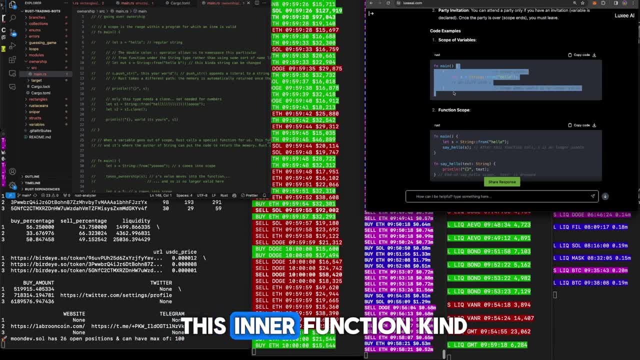 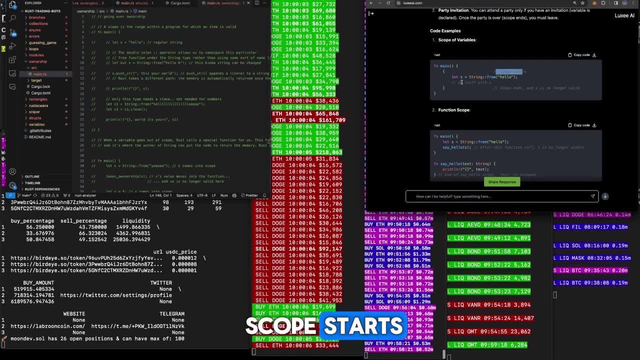 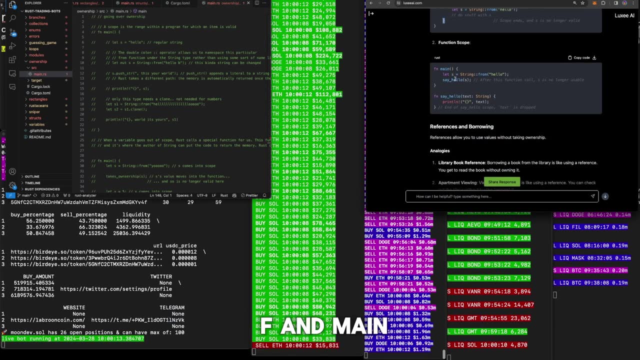 you can see here the function here, and then it made this inner function kind of LS. string is hello, and so anything in this would be that the scope starts and then do stuff with us. you could do stuff right here with us and the scope ends after this, so it's out of scope. so function scope F and main: let s equal. 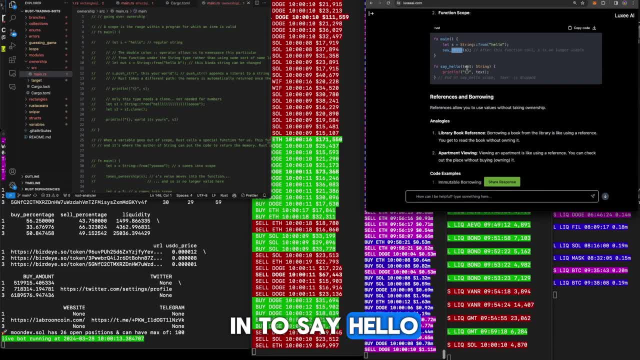 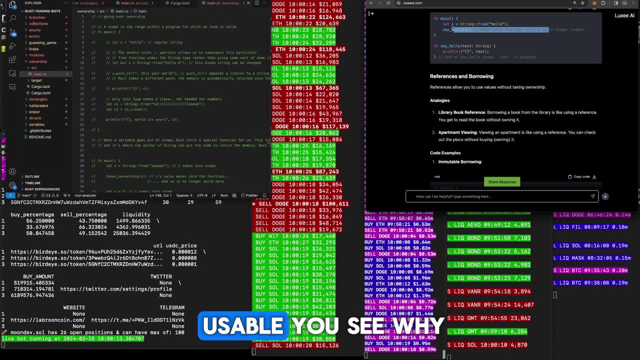 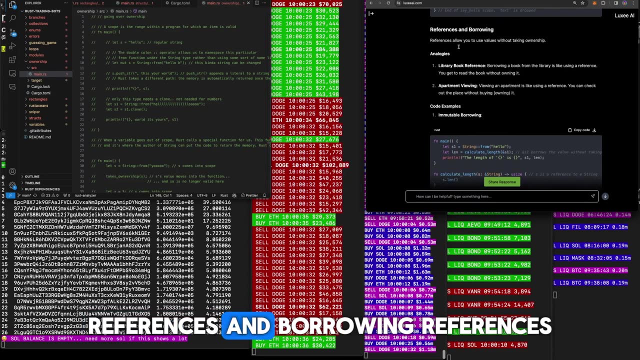 string hello, another hello string, then we pass it in to say hello, which is expected a string, and then we print ln with text. so, after this function, call s is no longer usable. you see why? because the ownership it doesn't have the, and if it was usable still would be. and references and borrowing references. 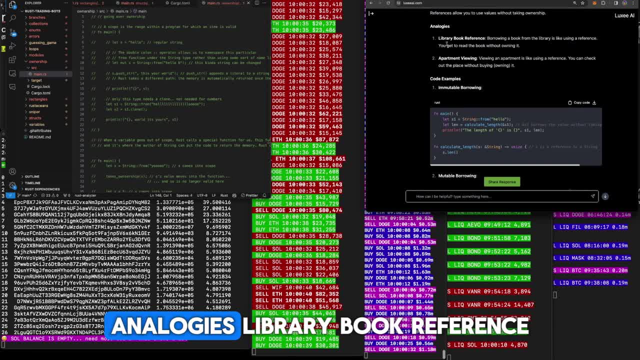 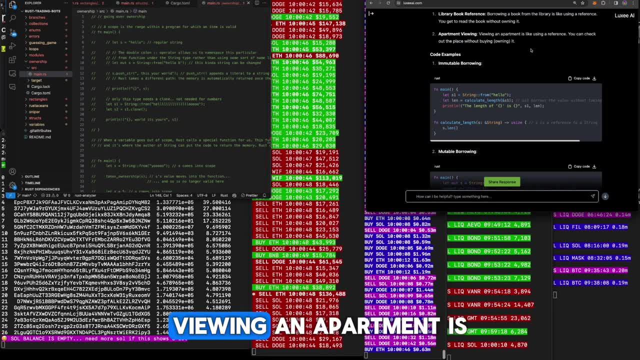 allow you to use values without taking ownership. you see why? because the ownership it doesn't have the end if it was usable. do analogies? library book reference. borrowing a book from the library is like using a reference: you get to read the book without owning it. viewing an 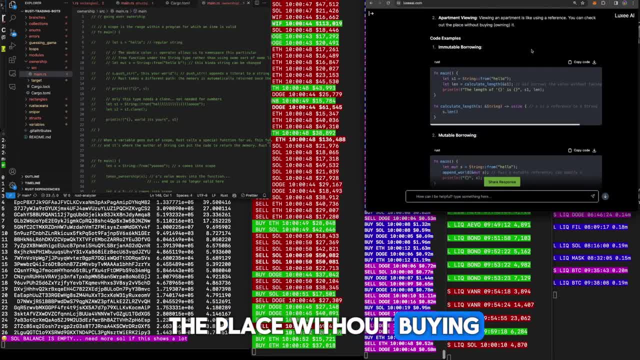 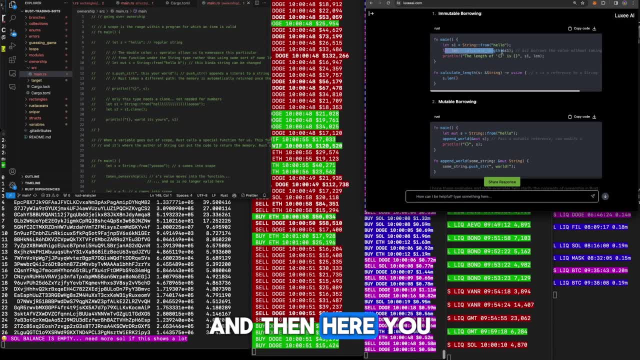 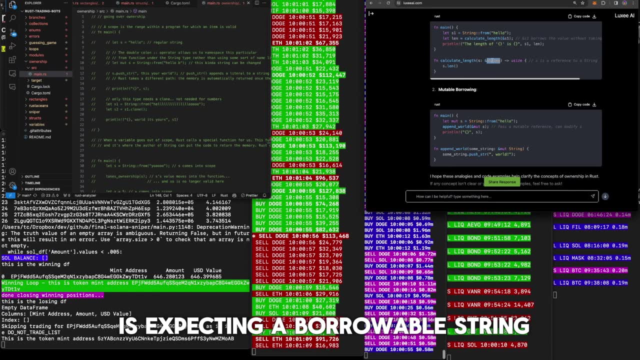 apartment is like: using a reference, you can check out the place without buying or owning it. code examples: immutable borrowing. so you can see same thing saying up the string. and then here you can see this is we're borrowing the s1, but it's immutable, not changeable, and this is expecting a borrowable string. 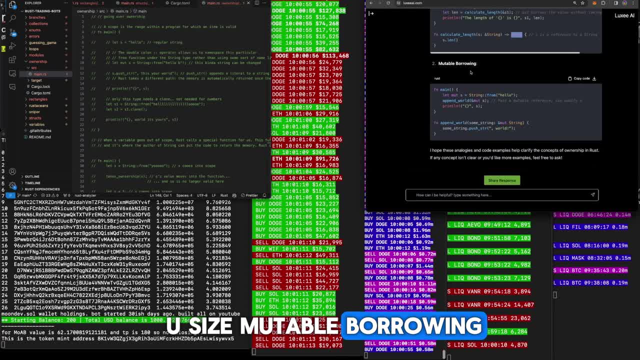 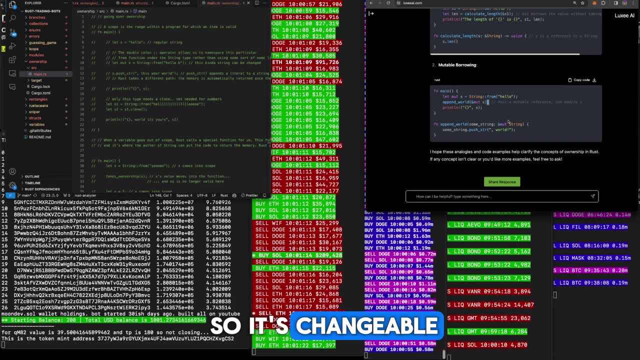 and it outputs a u-size mutable borrowing. so you can see. the only difference here is: this has mute, so it can change. so we borrow with the n sign and this is mutable, so it's changeable. and it says down here that it's expecting that and this is just a pending, a string. so I think that's a. 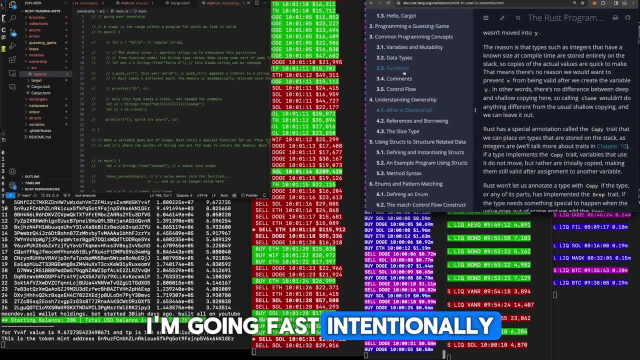 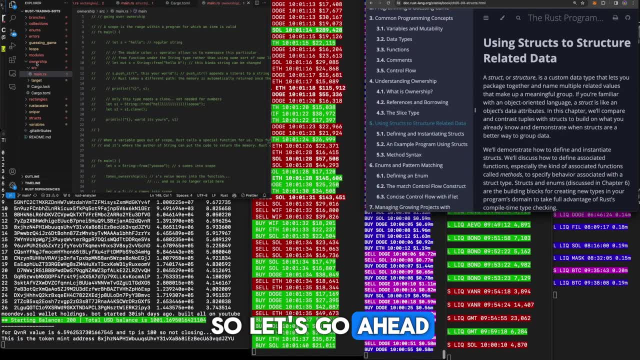 good little review of what ownership is. I'm going fast intentionally, because we've already gone through all of this using structs and structure related data, so let's go ahead and see if we can find our structure structs right here, and let's go ahead and see if we can find our structure. 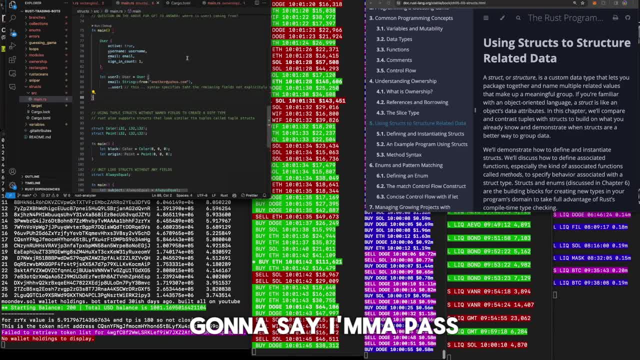 structs right here and let's go ahead and see if we can find our structure here. there it is. and then I'm just gonna say: I'm gonna pass all this into Luxy, and then let's go ahead and get that, read me here and let's learn about. 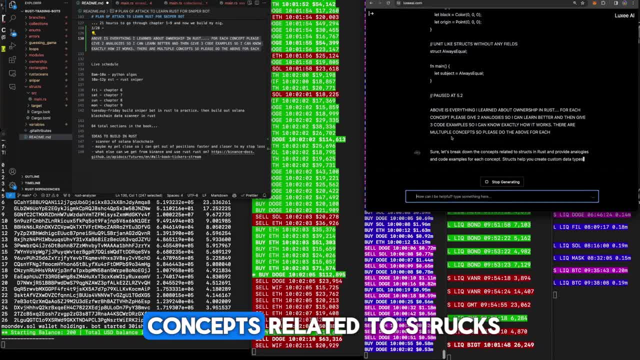 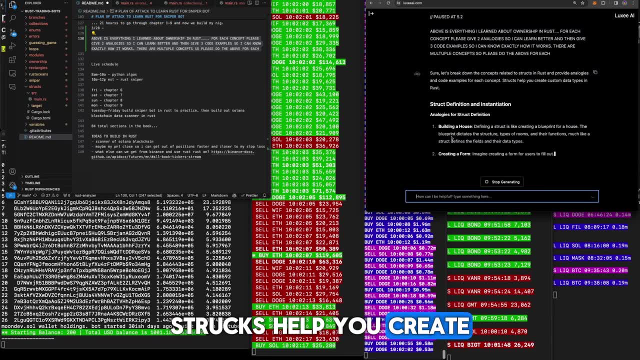 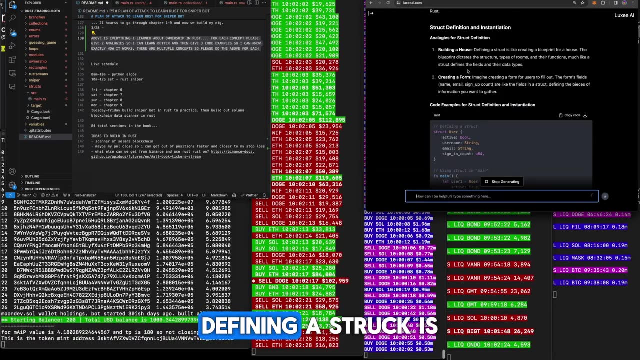 this. let's learn about it. sure, let's break down the concepts related to structs in rust and provide analogies and code examples for each concept. structs help you create custom data types in rust: struck definition and instantiation. instantiation: building a house, defining a struct, is like creating a blueprint for a house. the blueprint dictates. 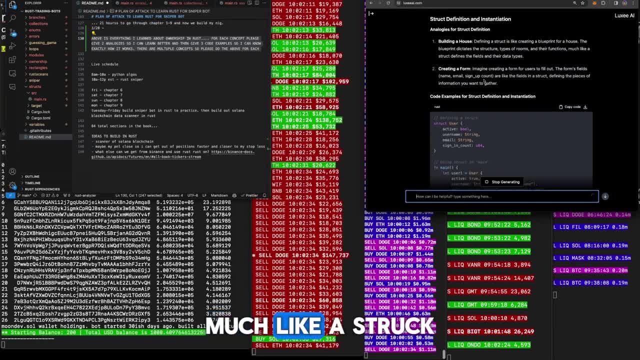 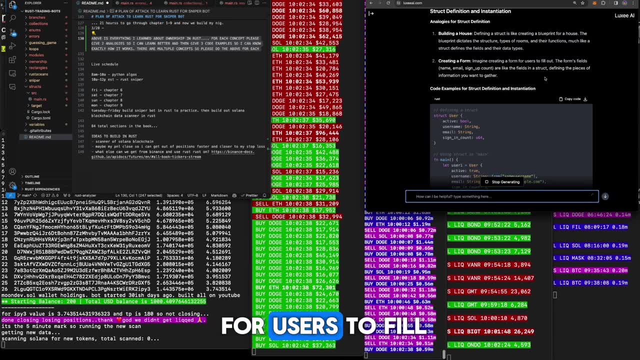 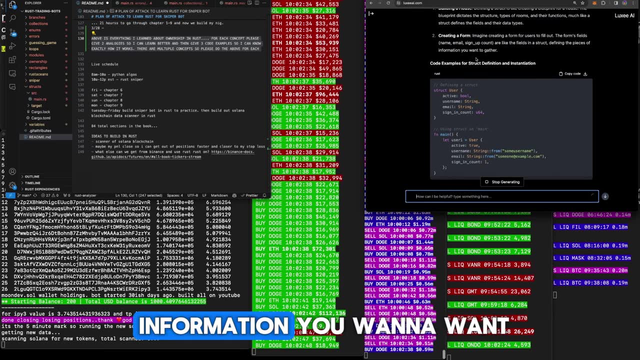 the structure, types of rooms and their functions, much like a struck defines the fields and their data types. creating a form- imagine creating a form for users to fill out the forms. fields- name, email, signup count- are like the fields in the struck, defining the pieces of information you want to want to gather. 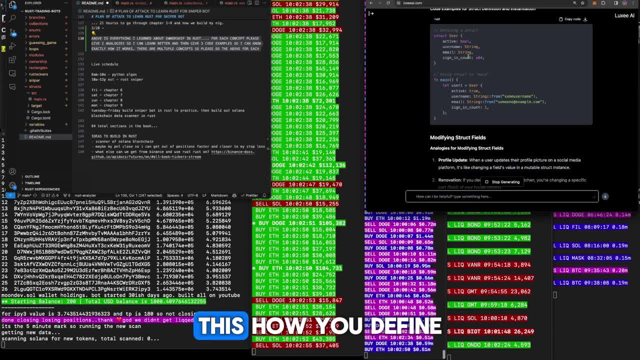 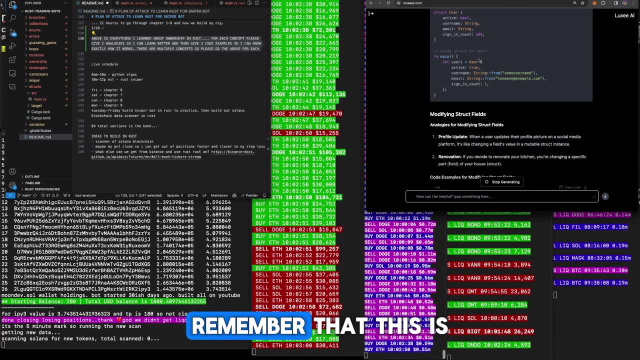 so code examples. so this is the actual struck is how you define a struck and you can say it's gonna be a bull string, string or a number. u 64 means number a. remember that this is how you make a function again and then you say: let user. 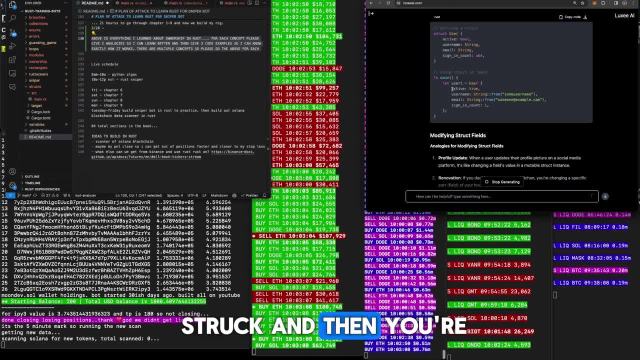 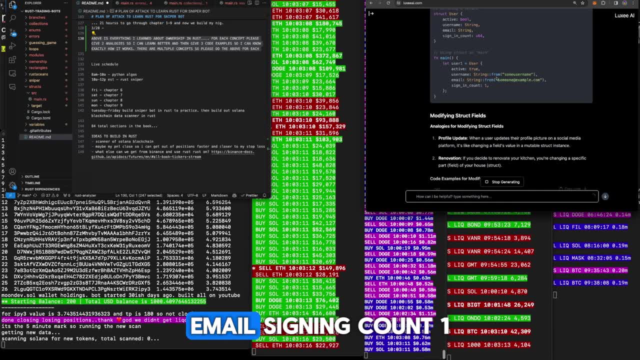 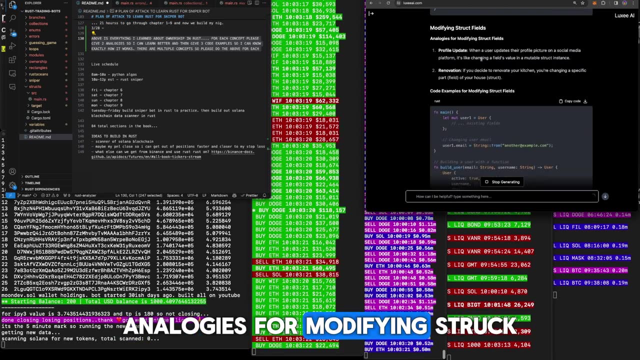 one equal user. so you're calling this struct and then you're saying it's active. is true username? is this username? email? is this username or email? signing count one and you can see it's expecting a number here. modifying struct fields. analogies for modifying struct fields: profile update: when a user updates their 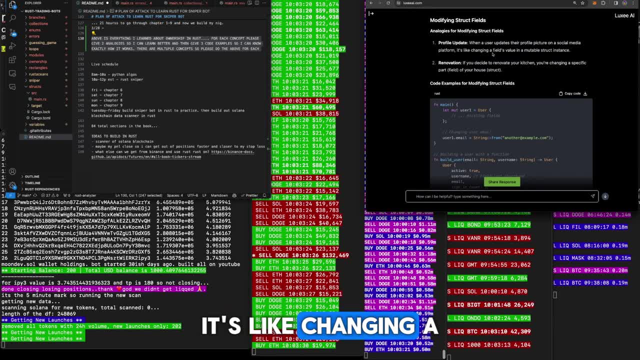 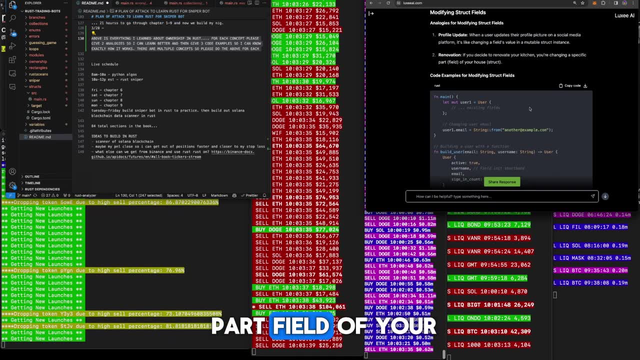 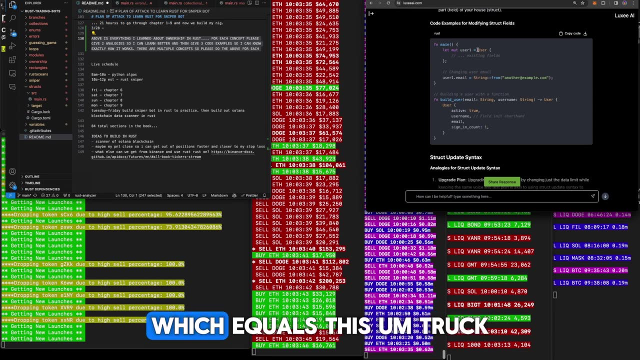 profile picture on a social media platform. it's like changing a field value in a mutable strut renovation: if you decide to renovate your kitchen, you're changing a specific part field of your house struck. here's some code examples of that. so we have the main function here and it's a mutable user which. 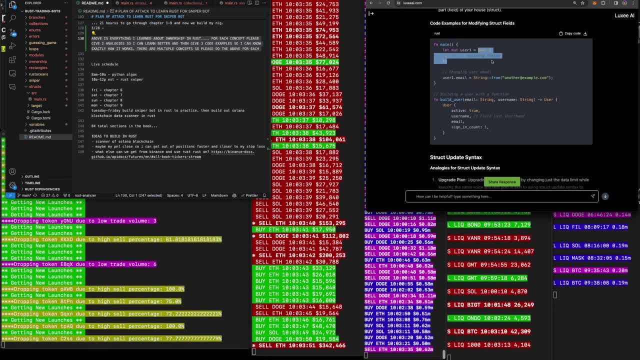 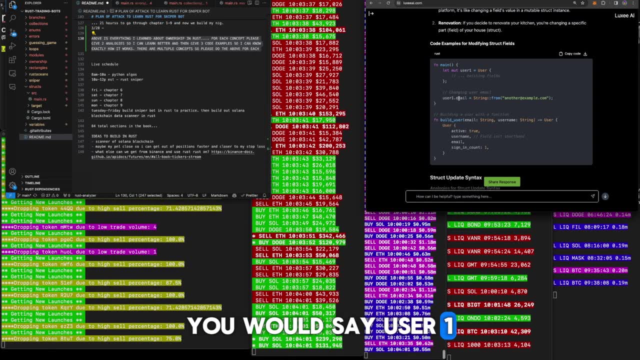 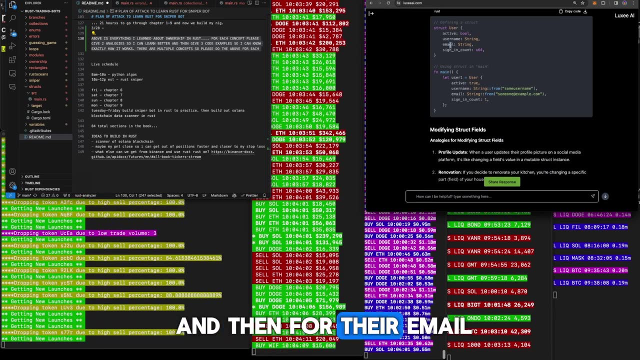 equals this truck. yep, you can see. the struct is up here, so it's playing off this one. and then you changing the email. you would say user one, dot, email and string, because user one will be calling this, which is calling this you, and then for their email it would pass in a string right there and then 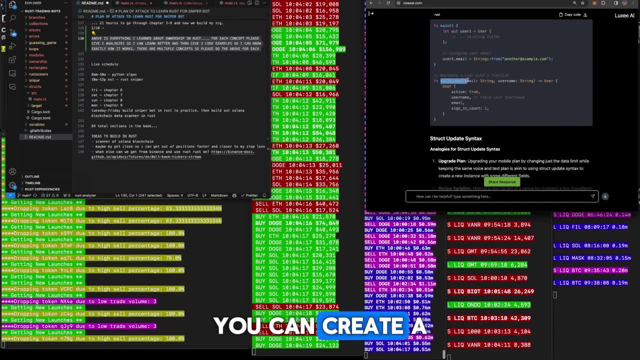 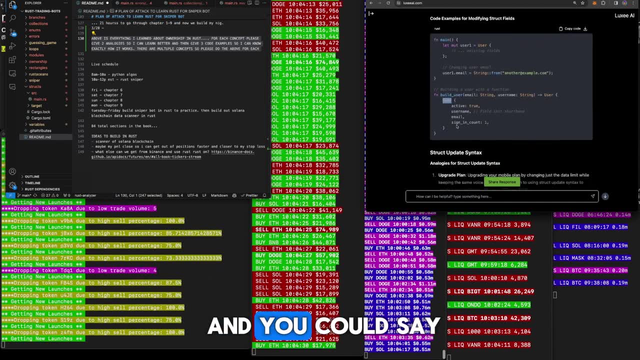 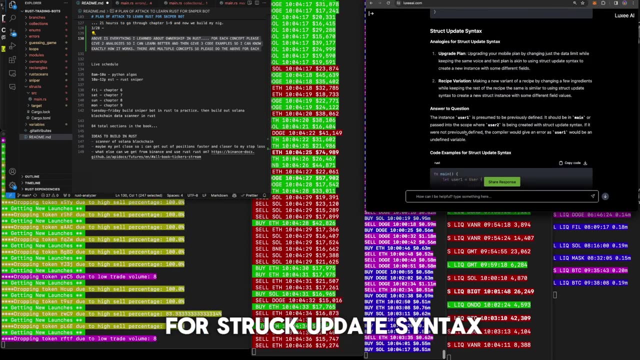 building a user with a function. so you can see you can create a new user by creating a function and say user again, that's calling this one up here, that's struck up there and you could say active, true, and then just pass in their username, email and how many times they signed in, struck, update syntax analogies for 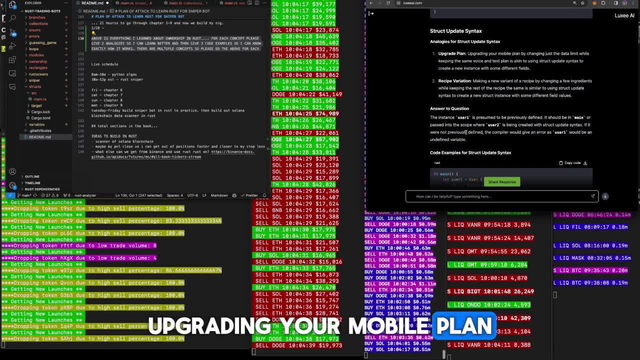 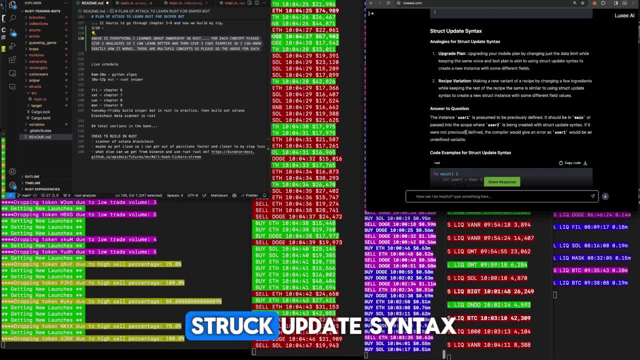 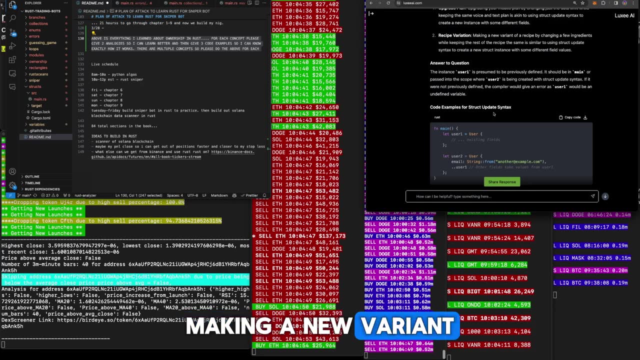 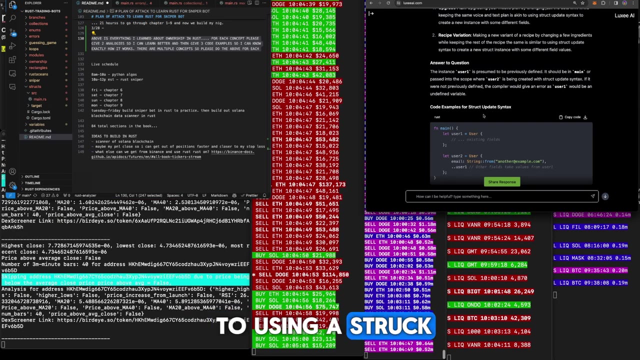 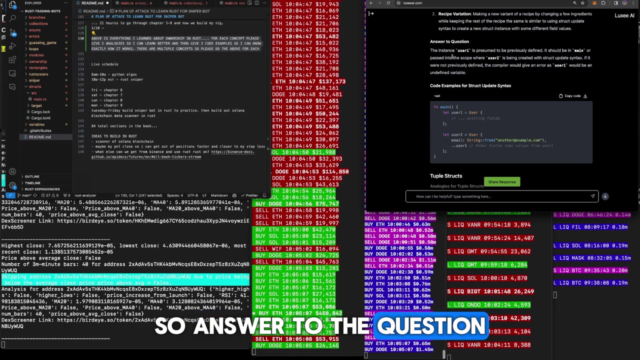 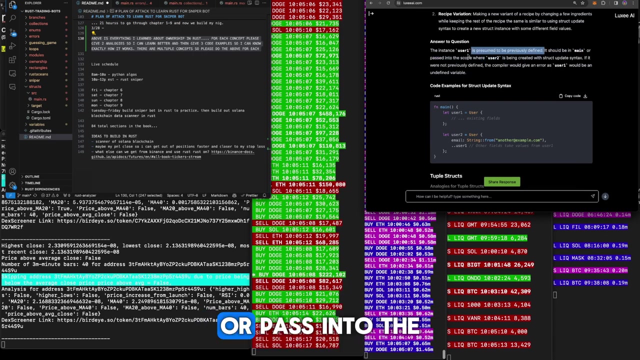 struck: update syntax, upgrade plan, upgrading your mobile plan by changing just the data limit while keeping the same voice and text plan in the same way. the method that grew into the recipe variation, the defense is rule file, are defined this method as following in main, or pass into the scope where user 2 is being created with the struct syntax, if it were. 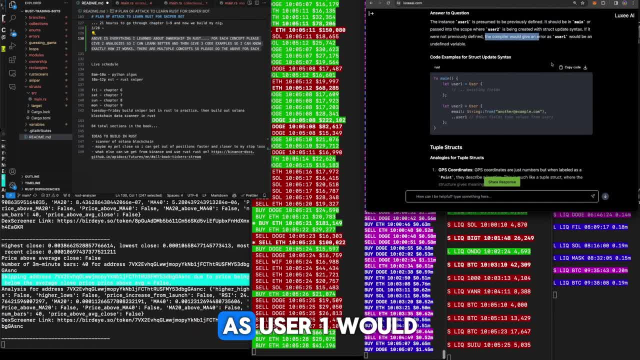 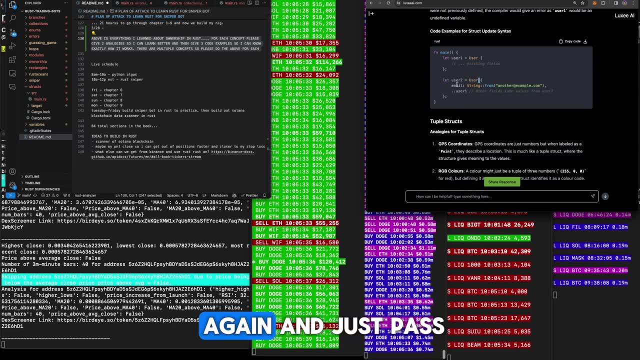 not previously defined. the compiler would give an error as user 1 would be undefined variable. so this is the same thing user 2 would call. we would call the struct again and just pass in the email here, and then this helps it inherit what's in user one. so whatever user one was, it inherits. 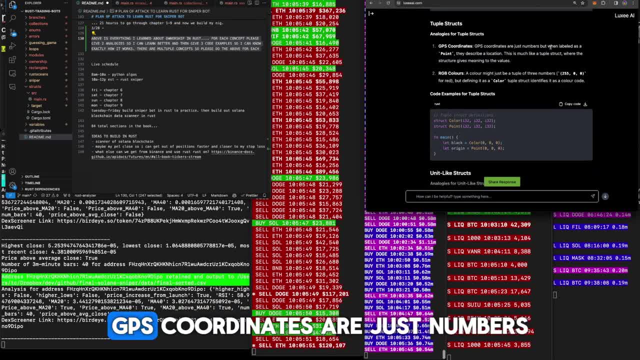 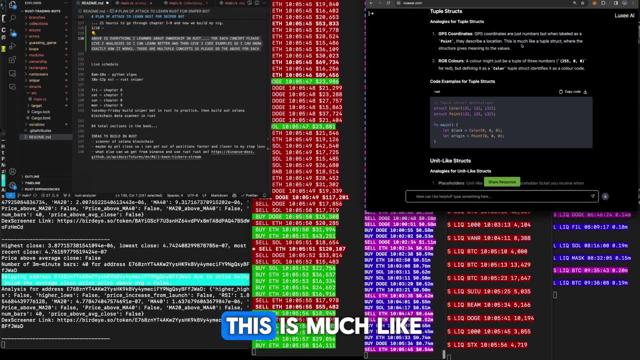 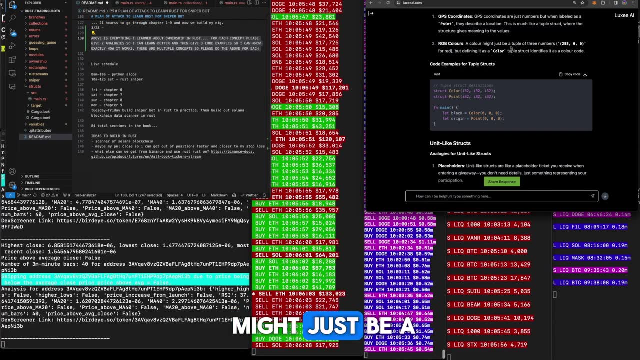 all that tuple structs analysis. for tuple structs, gps coordinates are just numbers, but when labeled as point they describe a location. this is much like a tuple struct, where the structure gives meaning to the values. rgb colors: a color might just be a tuple of three numbers: 20 255 0 0. 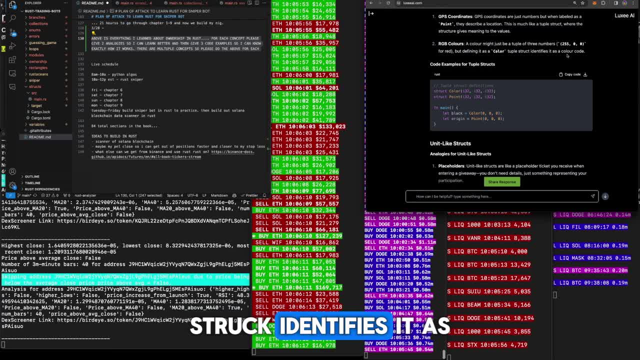 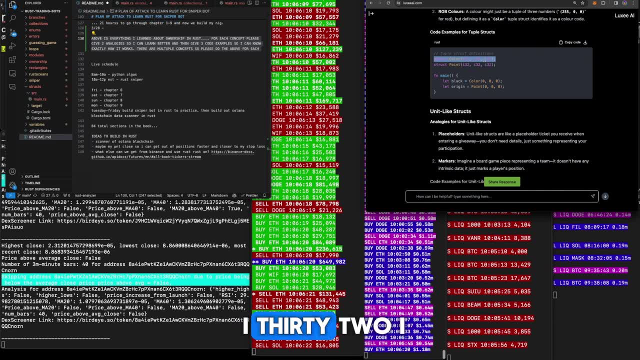 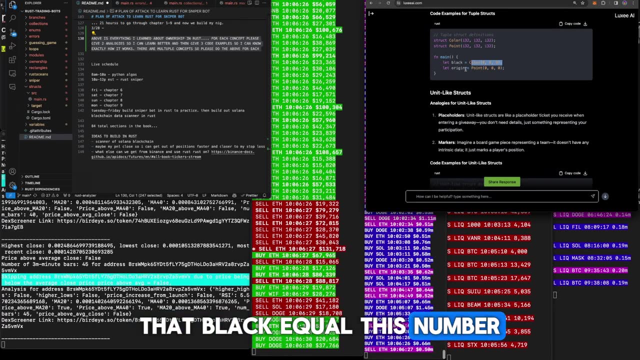 for red. but defining it as a color tuple struct identifies it as a color code, so you can see couple examples here. a struct color is i32, i32, i32- this is a little different format though- and then point i32, i32, i32. let black equal this number and let origin equal point zero. 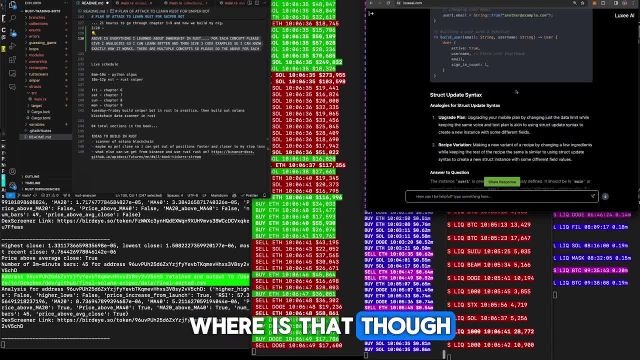 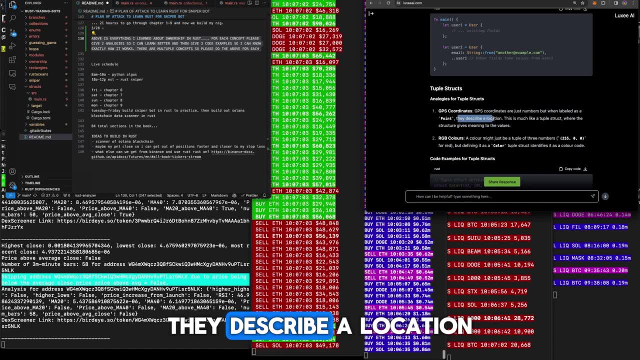 and what did point do again? oh, it points to. where is that, though? where'd you go? gps coordinates? gps coordinates are just numbers, but when labeled as point, they describe a location. location. this is much like a tuple struct, where the structure gives meaning to the value unit. like structs, 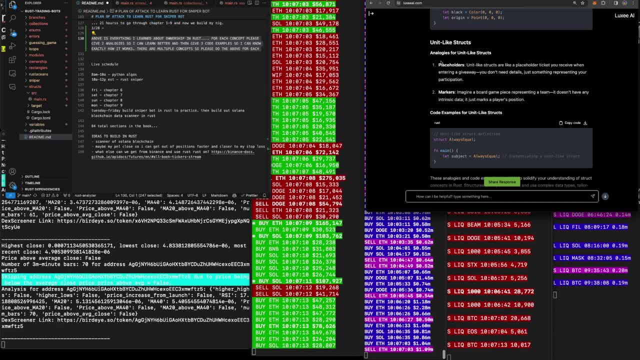 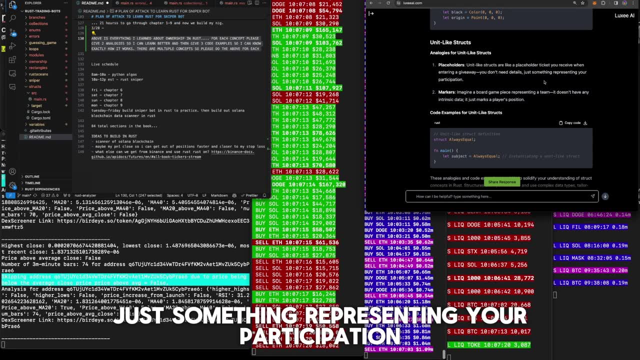 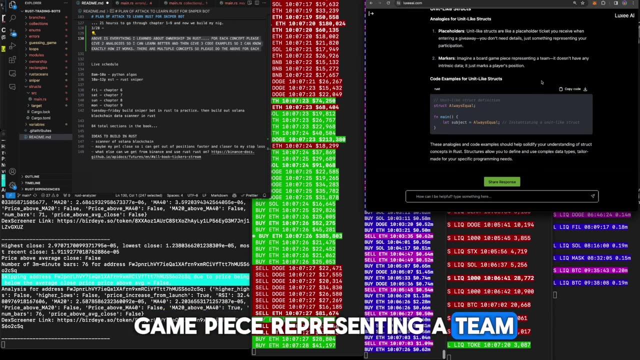 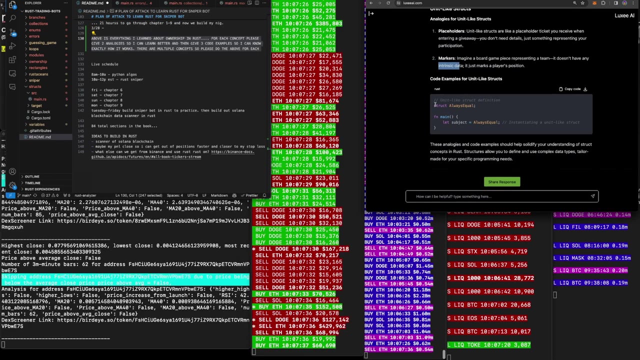 analogies for unit like strut, structs placeholders. unit like structs are like a placeholder ticket you receive when entering a giveaway. you don't need details, just something representing your participation markers. imagine a board game piece representing a team. it doesn't have any interest in trend intrinsic data, it just makes a player's position. so here. 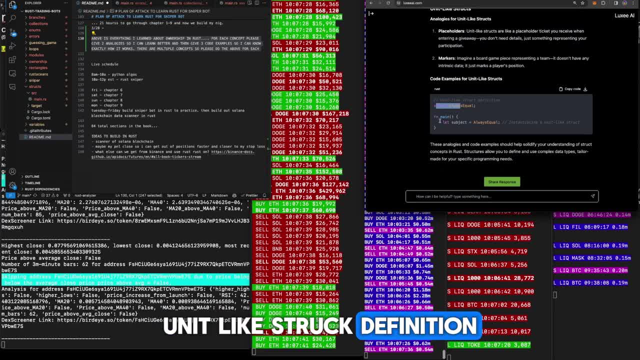 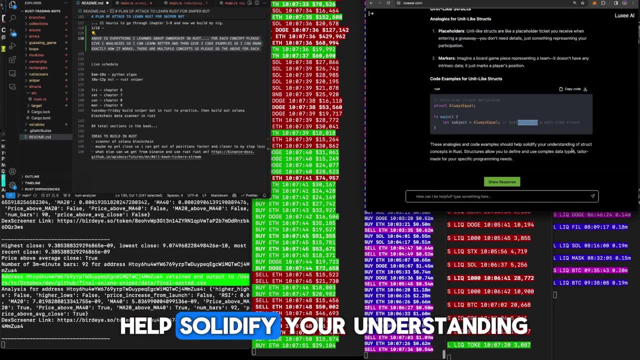 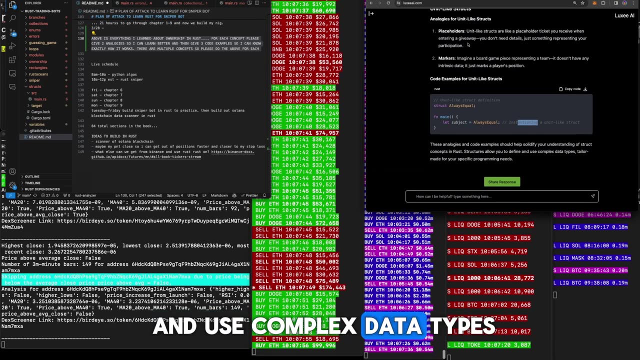 the structure gives meaning to the value. unit like structs. analogies for unit like structs: struct is always equal. unit like struct. definition. and then let subject instantiating a unit like struct. these analogies and code examples should help solidify your understanding of struct concepts and rust structures, allow you to define and use complex data types tailor-made for your 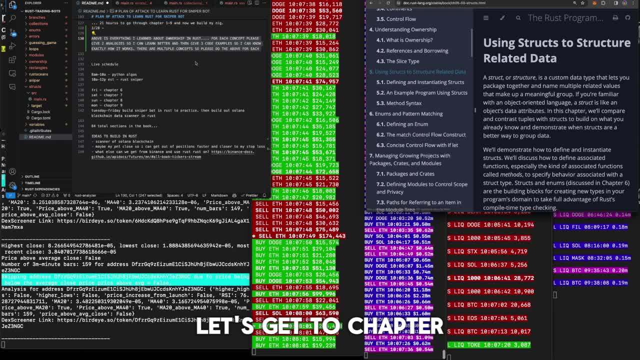 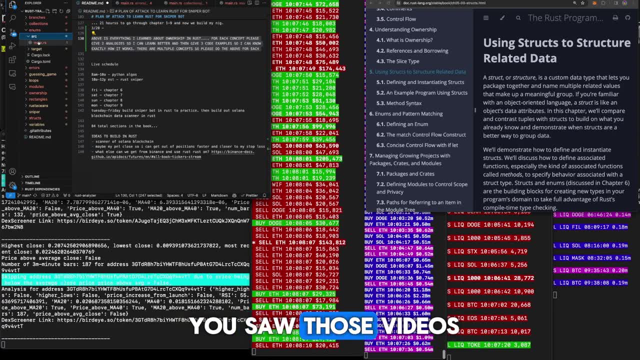 specific programming needs. all right, let's move on. let's get to, uh, chapter six, enums. so these are again my notes over here. we already went through all of these and hopefully you saw those videos. if you're interested in learning more about the structure of structs, you can click the link in the 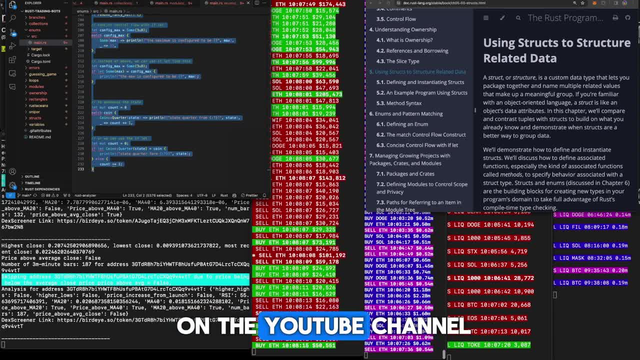 description box below and you'll be able to see all of these and hopefully you saw those videos. if you're interested in learning more about the structure of structs, you can click the link in the description box. not, they will be here soon, they will be here on the youtube channel for free, because everything's. 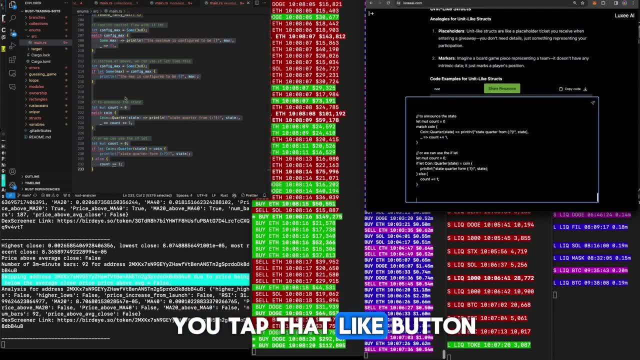 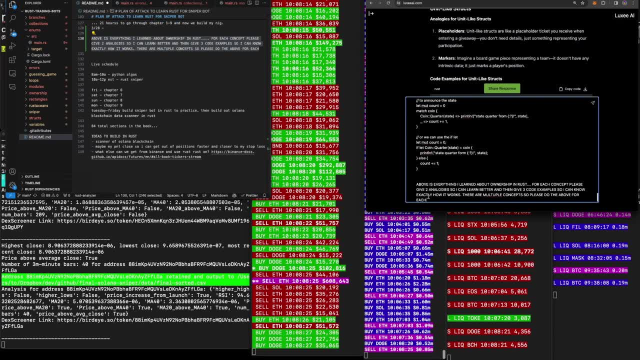 free on the youtube channel. all i ask is you tap that like button. that's the only thing i need from you. you don't have to pay me anything. ever, ever, ever ever. if you want a fast path pass, you can join the bootcamp. the bootcamp shows you, step by step, how to get up to speed with me. 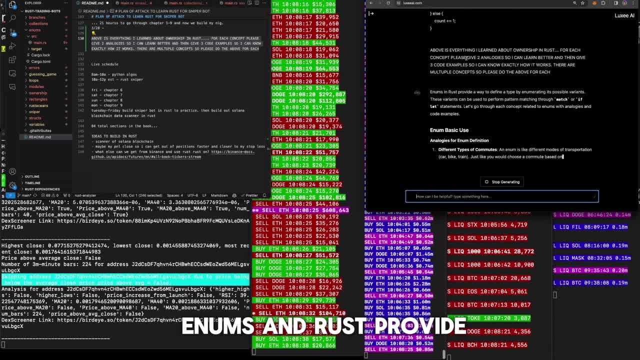 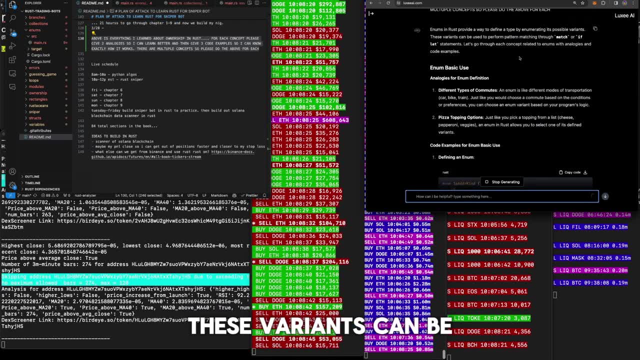 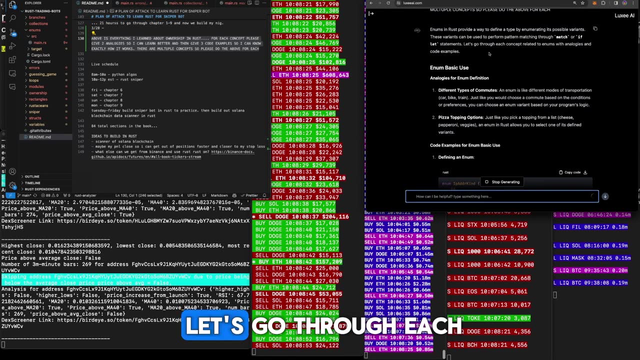 but it's not required. enums and rust provide a way to define a type of enumerating its possible variants. these variants can be used to perform pattern matching through match or, if let, statements. let's go through each concept related to enums and with analogies and code examples. 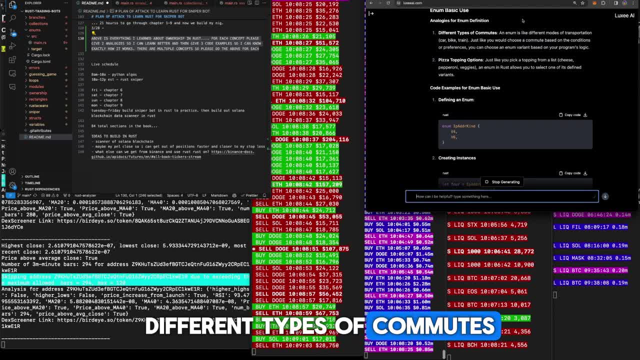 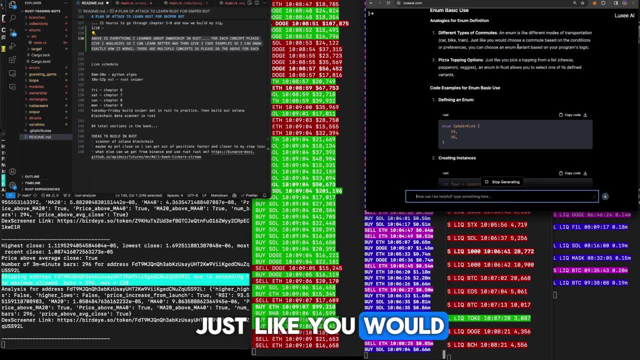 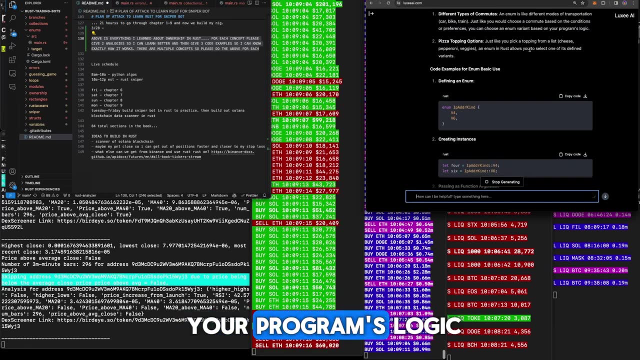 analogies for enum definition: different types of commutes. an enum is like different modes of transportation: car, bike, train. just like you would choose a commute based on the conditions or preference, you can choose a commute based on the conditions or preference. you can choose a commute based on the conditions or preference. you can choose an enum variant based on your program's. 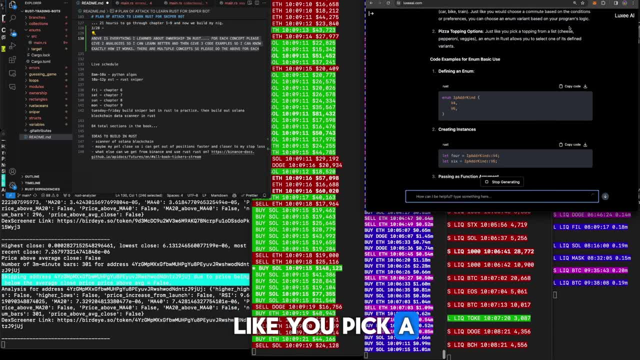 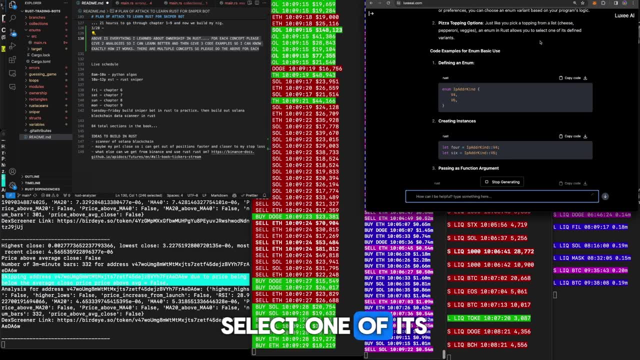 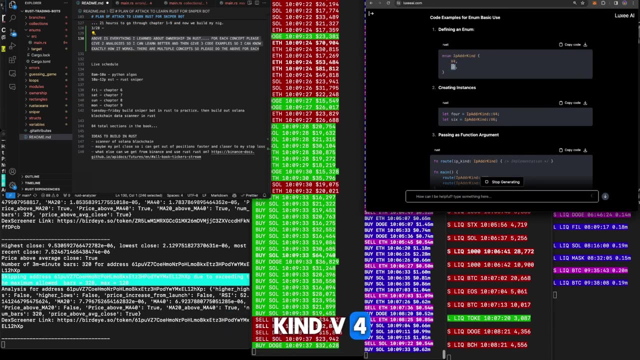 logic enum variant based on your program's logic pizza topping options, just like you pick a topping from a list- cheese, pepperoni, veggies- an enum is in rust allows you to select one of its defined variants. so defining the enum is like this: this is the enum name. ip address: kind v4, v6- create. 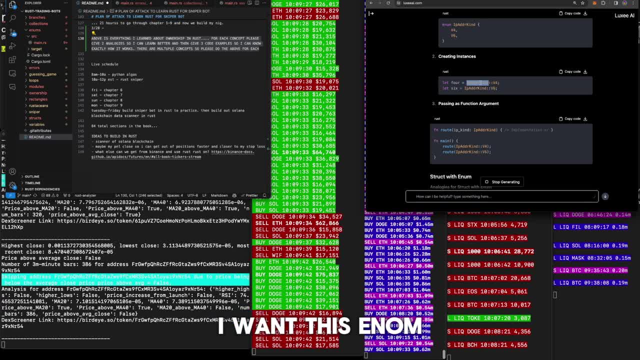 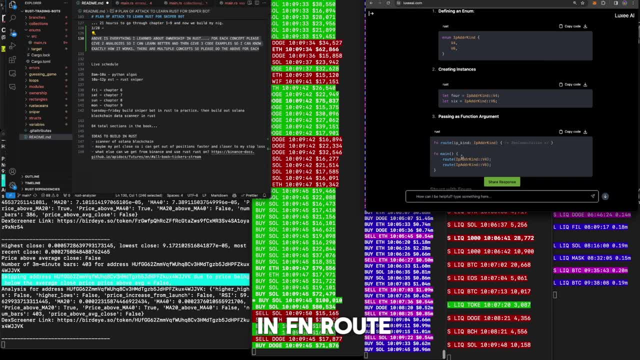 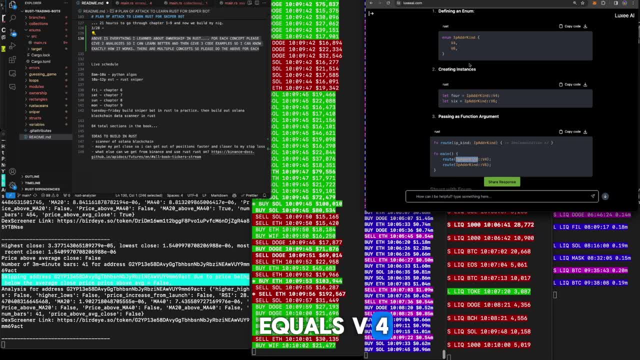 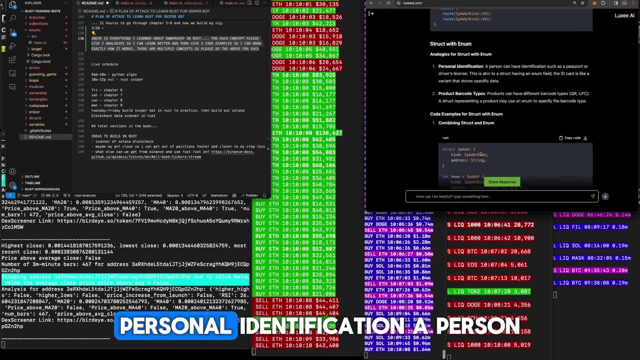 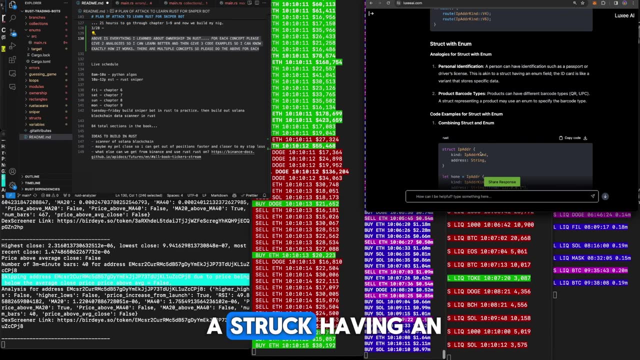 ip kind and then route: ip kind equals v4, so it'd be v4 and v6. struct with enums. analogies for struct with enums: personal identification. a person can have identification such as a passport or driver's license. this is akin to a struct having an enum field. the id card is like a variant that stores. 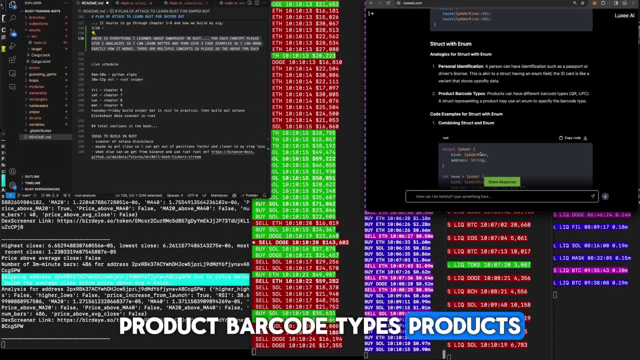 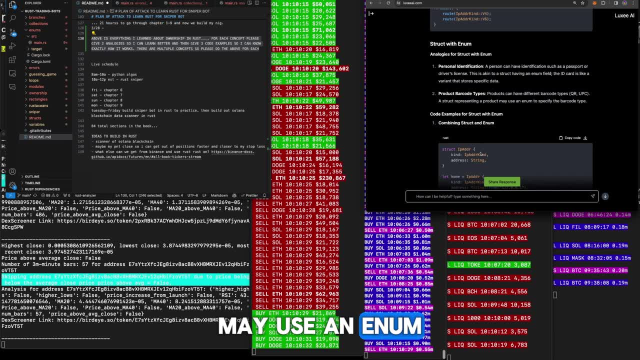 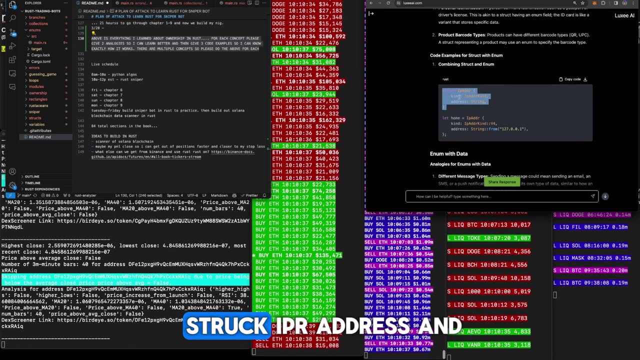 specific data: product barcode types. products can have different barcode types: qr, upc. a struct representing a product may use an enum to specify the barcode type. so this is combining structs and enums. remember, we just learned about structs, so we make a struck ipr address and then let home equal. 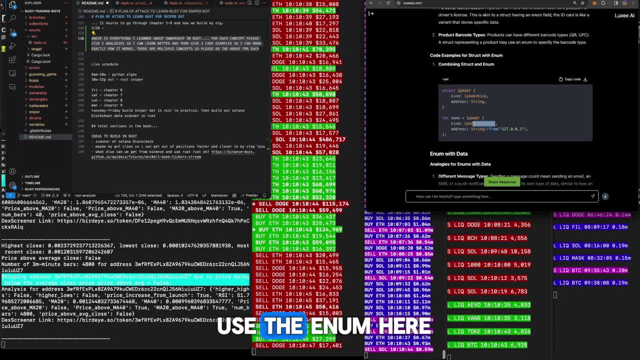 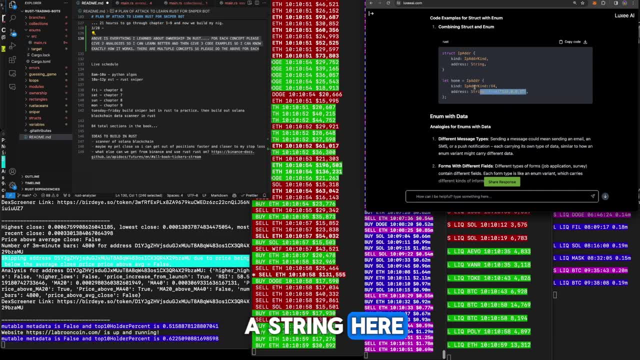 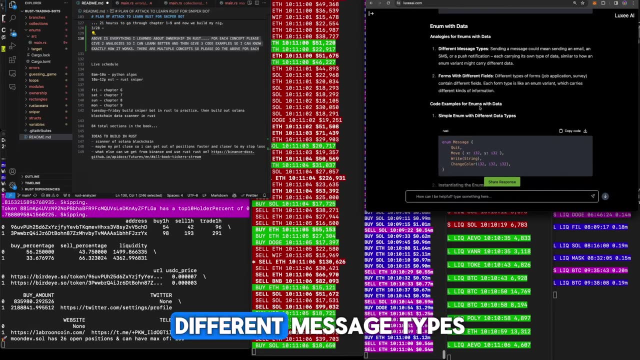 ip address, the kind is going to use the enum here from up here and the string is going to use- or it's going to be a string here, but you can see it needs the ip address kind and the address string. so enum with data. analogies for enum with data, different message types. sending a message could mean. 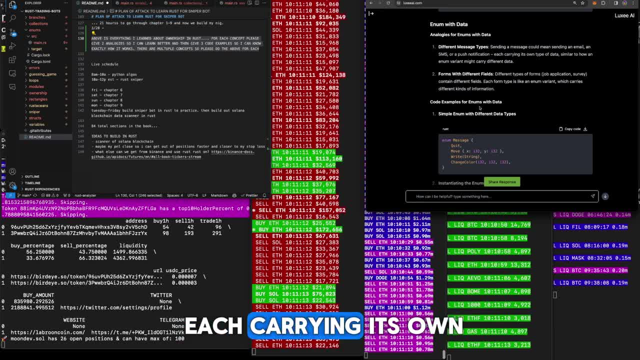 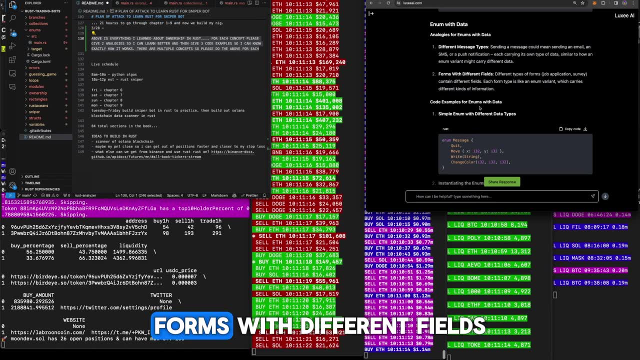 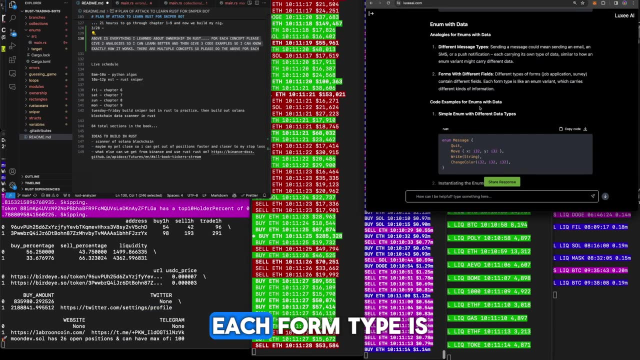 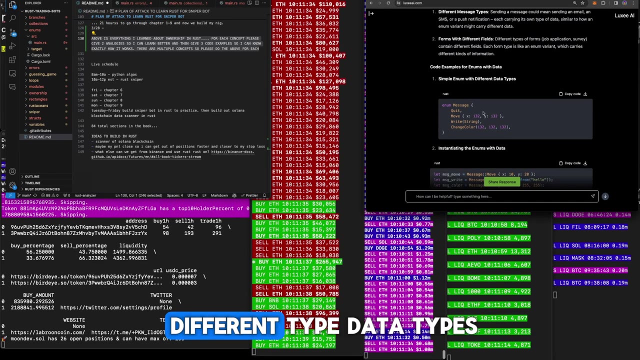 sending an email, an sms or a push notification, each carrying its own type of data. similar to how an enum variant might carry different data forms with different fields. different types of forms. job applications surveys contain different fields. each form type is like an enum variant which carries different kinds of information. so simple: enum with different. 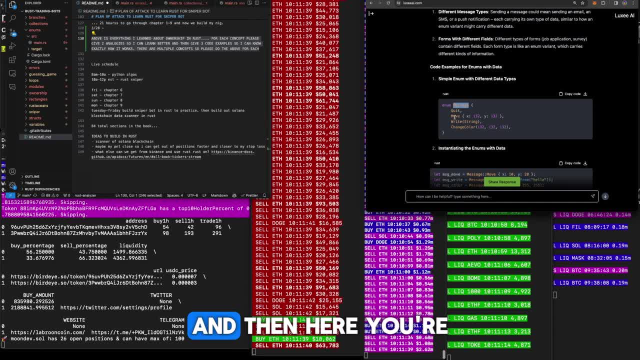 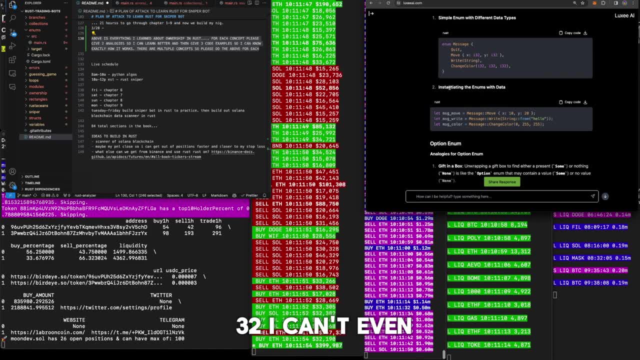 type data types. you can see, here you make the enum and then here you're defining different data types. i32 is the type of number. uh, this is string i32. i can't even say that word. instantiating the enums: i can't even say that word. yes, you can, bro. 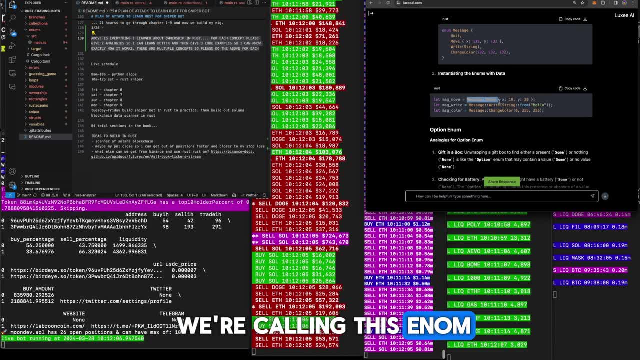 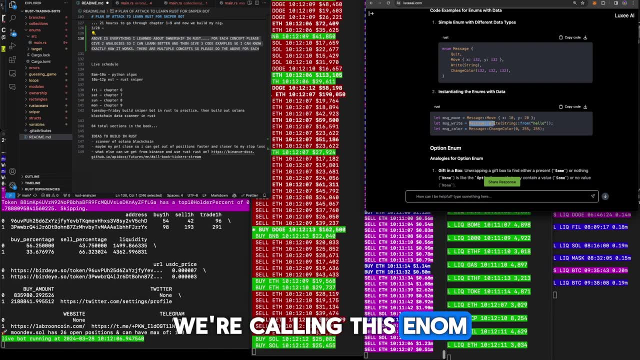 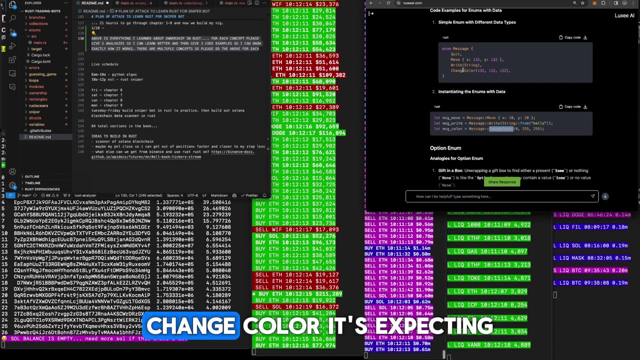 do anything, dude. so you can see we're calling this enum, move here. and then we're passing in the two numbers: same here, message we're. we're calling this enum of message again, but right here it needs to be a string. so we're passing the hello message: change color. it's expecting. 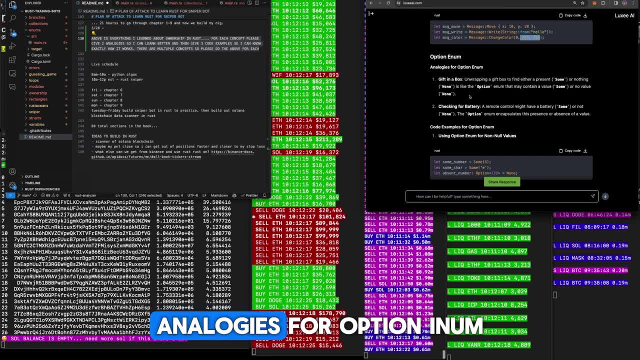 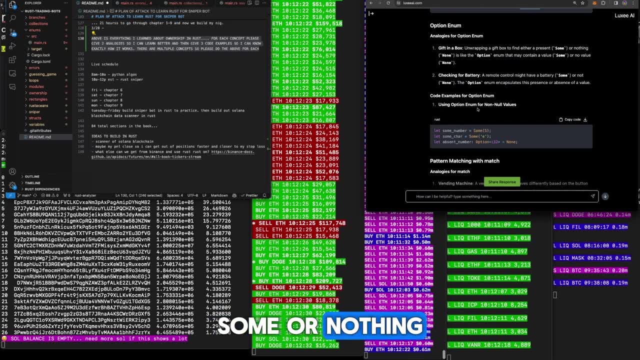 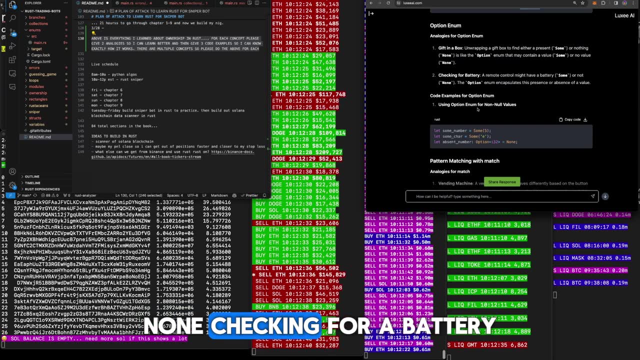 three numbers which we give it: option enum. analogies for option enum: gift in a box. unwrapping a gift box to find either a present, some or nothing. none is like the option that may contain a value, some or no value- none. checking for a battery: a. 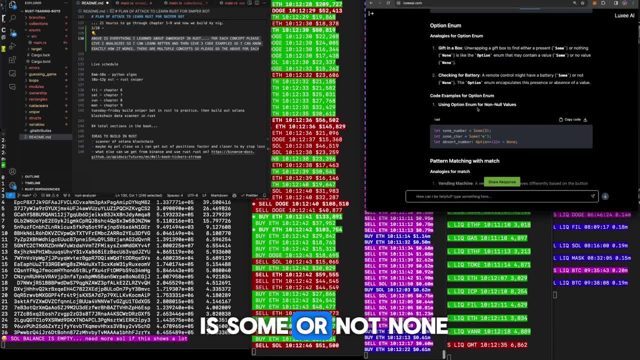 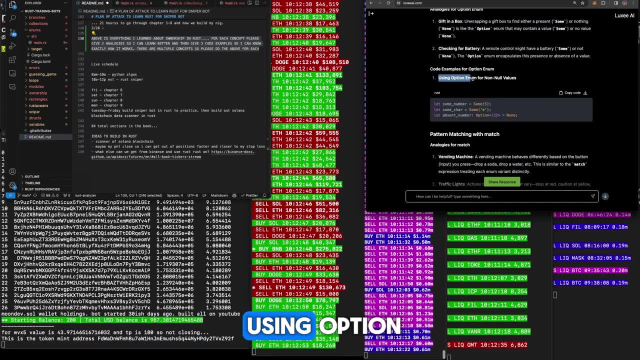 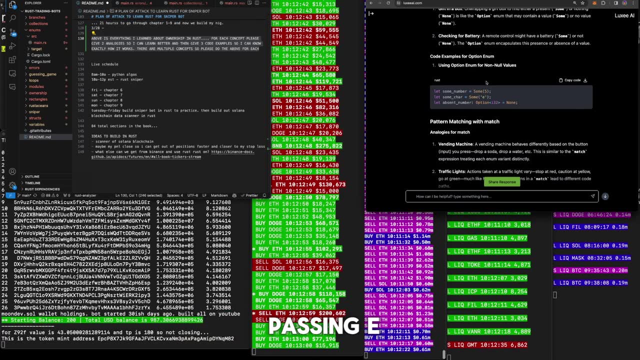 remote control might have a battery which is some or not none, or the option enum encapsulates this presence or absence of a value, using option enum for non-null values. so some number equals some passing five, some char equals some passing e, and then this is the option t thing we learn and we're. 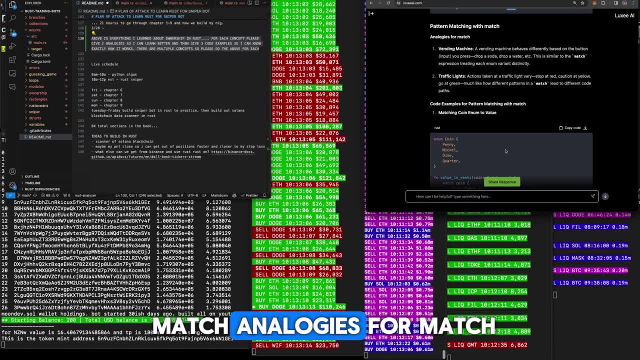 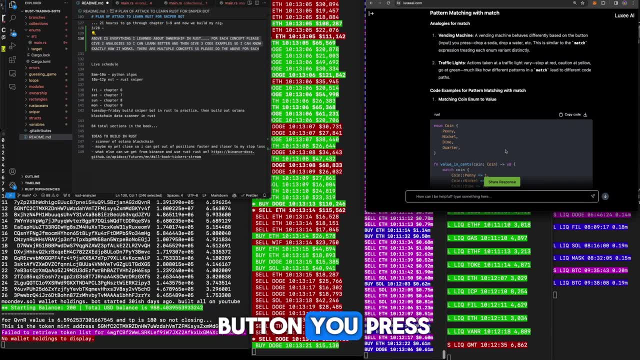 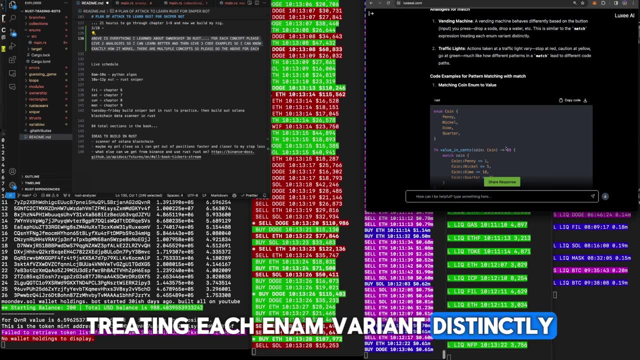 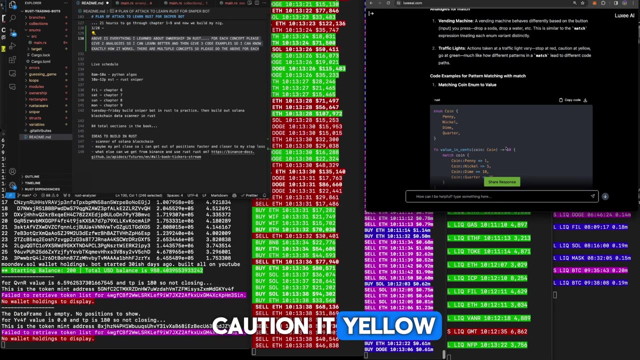 saying none. so pattern matching with match analogies for match vending machine: a vending machine behaves differently based on the button you press: drop a soda, drop of water, etc. this is similar to the match expression treating each enum variant distinctly. take actions taken at a traffic light vary: stop at red, caution at yellow, go to green, much like how different patterns in a match. 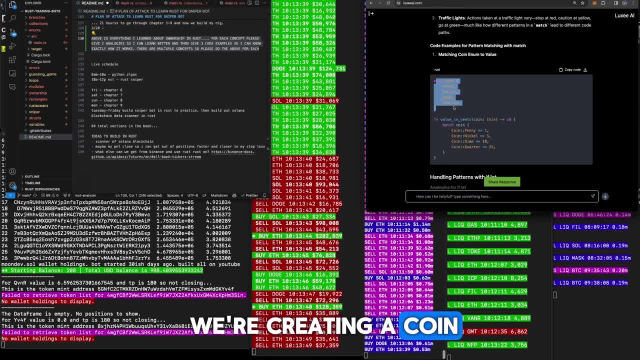 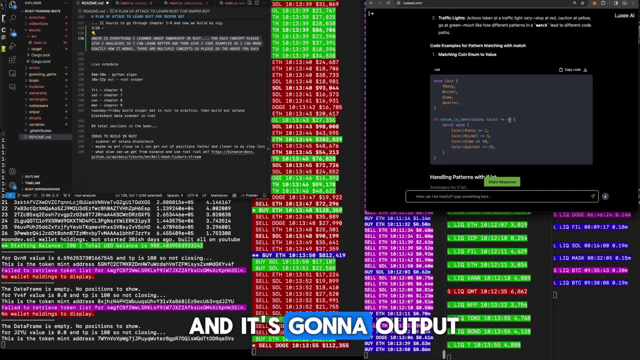 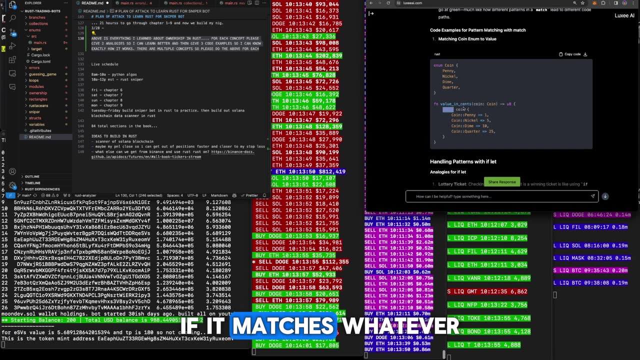 lead to different code paths. so you can see, we're creating a coin enum here saying penny, nickel, dime, quarter. then we're creating a function here and it needs coin and it's going to output a number, a u8 number, which is a certain type of number- we learned about that- and then we're saying, hey, if it matches. 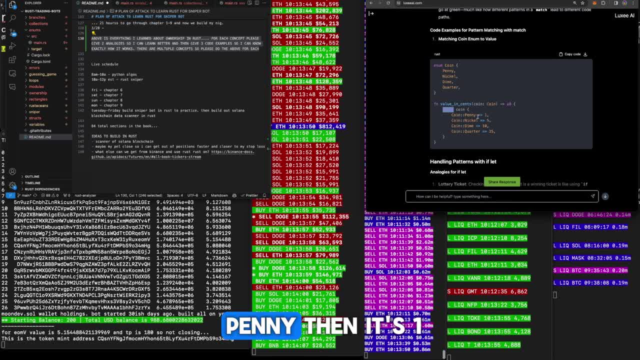 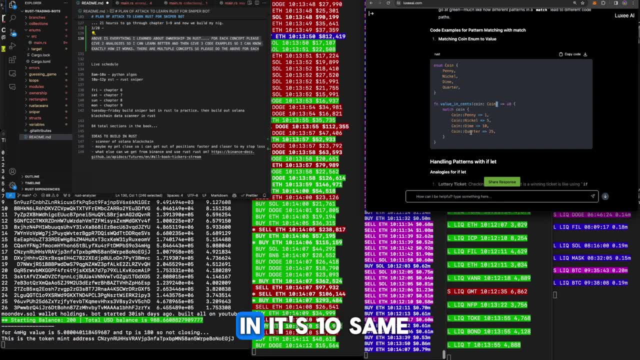 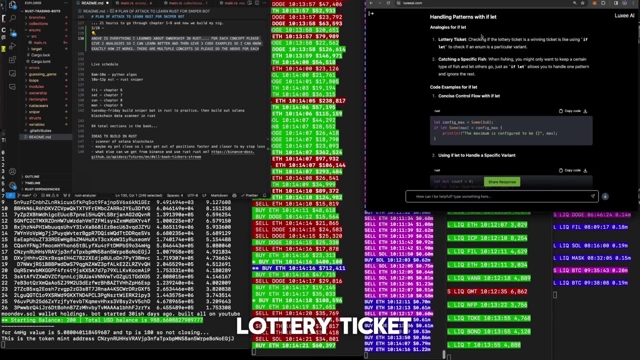 whatever we pass in, if it matches a penny, then it's one. if it matches a nickel, then it's five. if it matches a dime, the thing we passed in, it's ten same. with the quarter handling patterns, with if let, analogies for if let, lottery ticket checking: if the lottery ticket is a winning. 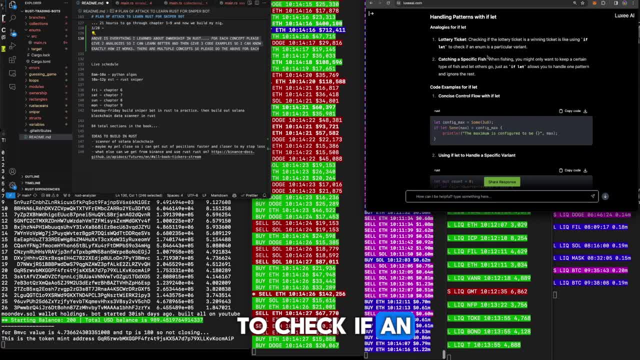 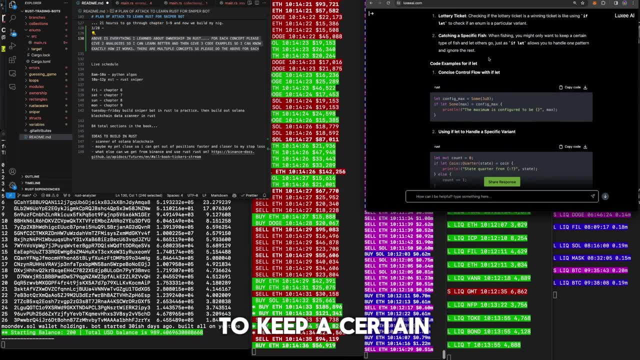 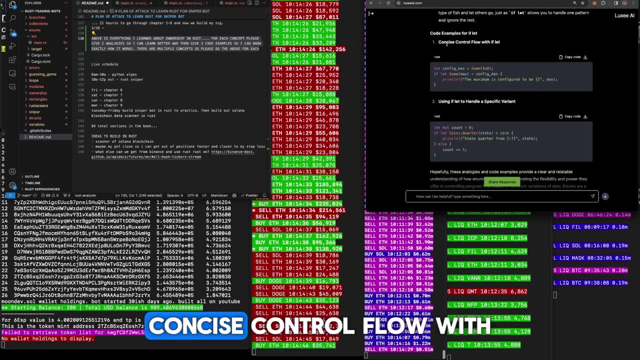 ticket is like if let to check if an enum is a particular variant catching a specific fish. when fishing you might only want to keep a certain type of fish and let others go, just as if let allows you to handle one pattern and ignore the rest. concise control flow with if let, so let config. 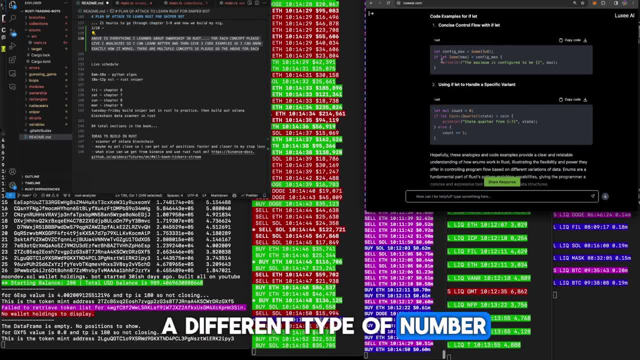 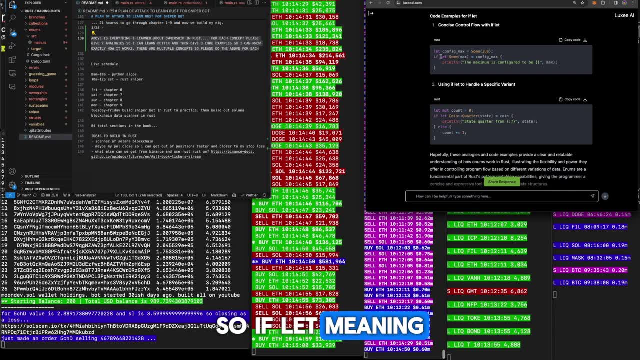 equals sum 3u8 be a different type of number. if let sum max, so we pass in some max config print ln. so if let, meaning if that thing is true, then go in there and print. if not, then don't using if let to handle a. 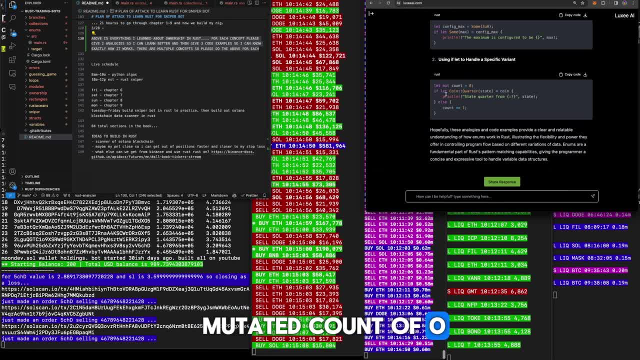 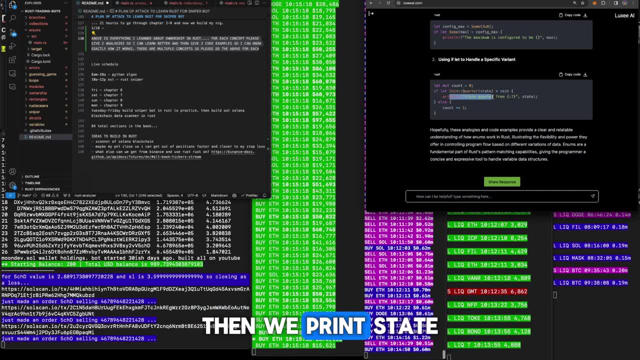 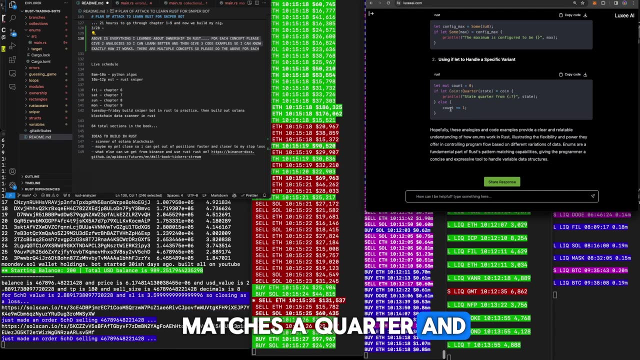 specific variant. so this is a mutated count of zero. if coin state- if it matches a quarter- equals coin, then we print state quarter from blank state. so we pass in the state if it matches a quarter and then we add one. hopefully these analogies and code examples. 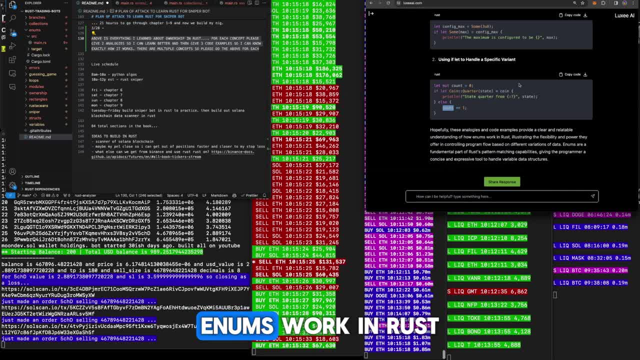 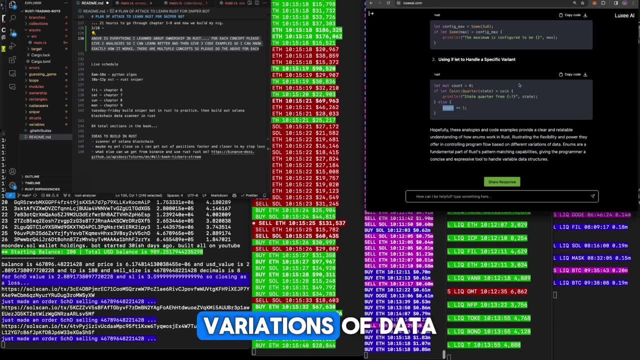 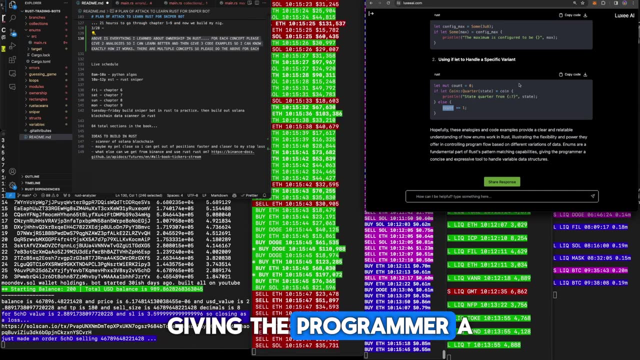 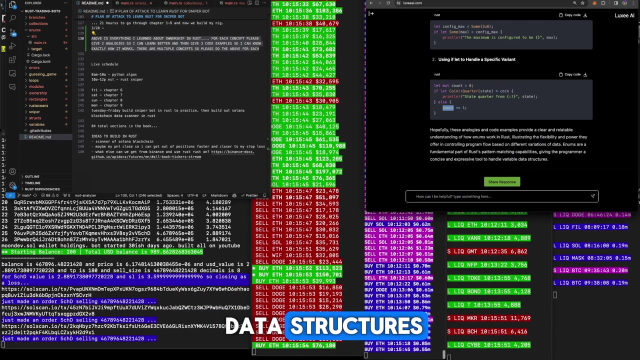 provide a clear and relatable understanding of how enums work in rust, illustrating the flexibility and power they offer in controlling program flow based on different variant variations of data. enums are a fundamental part of rust pattern matching capabilities, giving the programmer a concise and expressive tool- a concise and expressive tool to handle variable data structures. 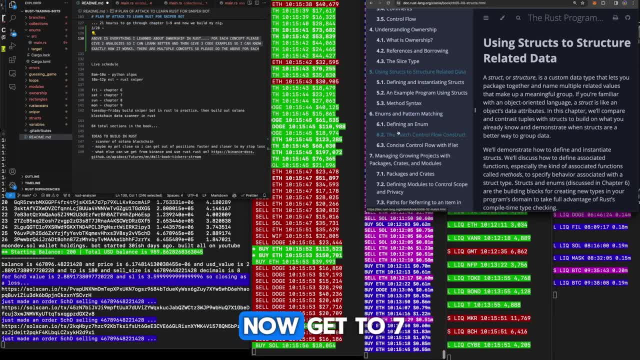 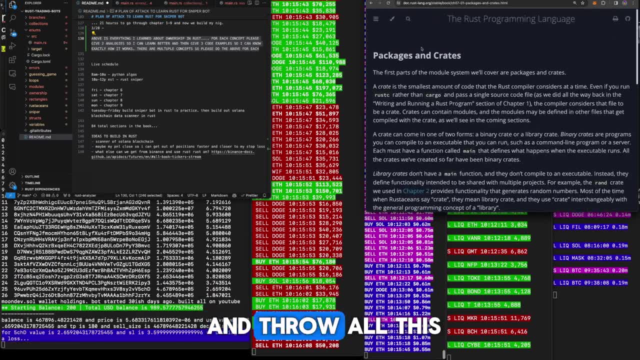 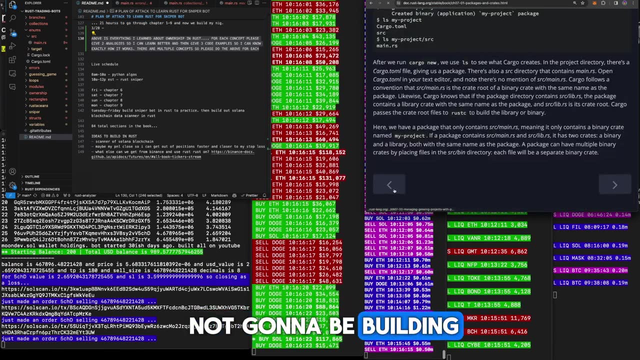 nice dude. so we're flying through this. let's go ahead and now get to seven, which we don't need too much. but, um, let's just go ahead and throw all this in there, because we didn't actually read this chapter, because it's not needed, i guess, because we're not going to be building crates and stuff. but 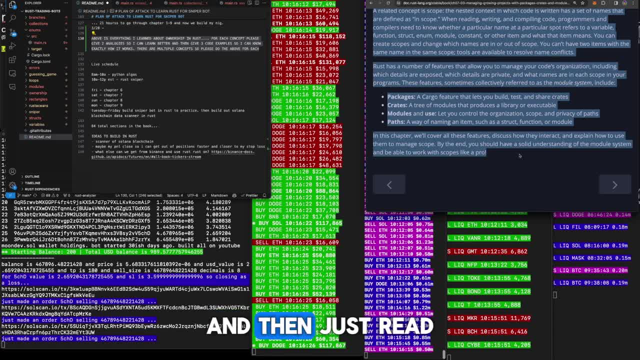 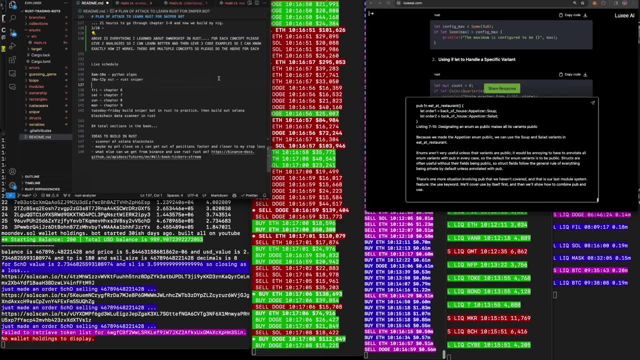 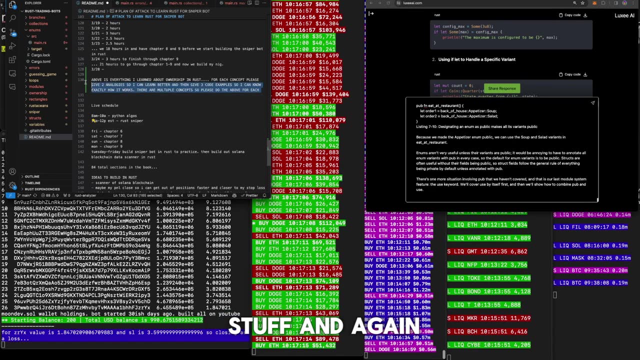 let's just go ahead and throw all this stuff in there and then just read through it really quickly. i put all of this in there so we don't miss a thing. that's probably good. i hear it's not too important to know this stuff, but i think we'll learn it on on the road to building stuff and 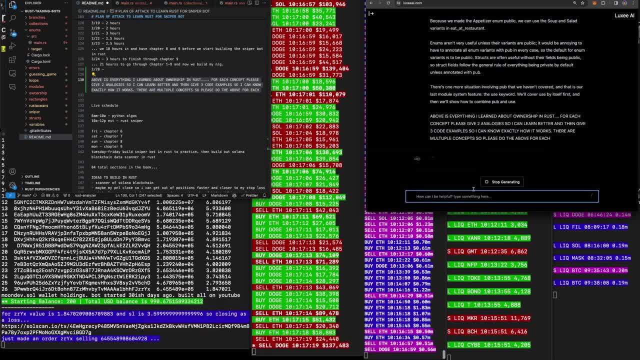 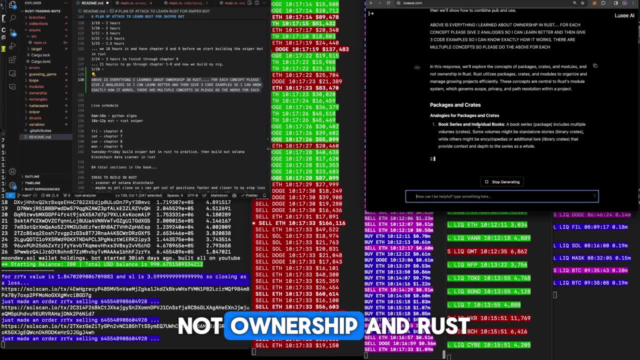 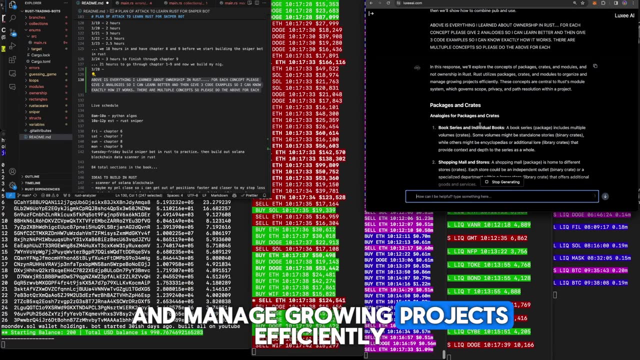 again. i'm learning all this stuff so i can parse through the solana blockchain. just in case you're wondering, in this response we'll explore the concepts of packages, crates and modules, and not ownership and rust. rust utilizes packages, crates and modules to organize and manage growing projects. 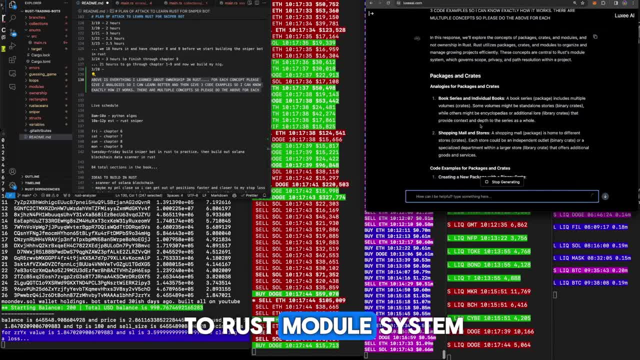 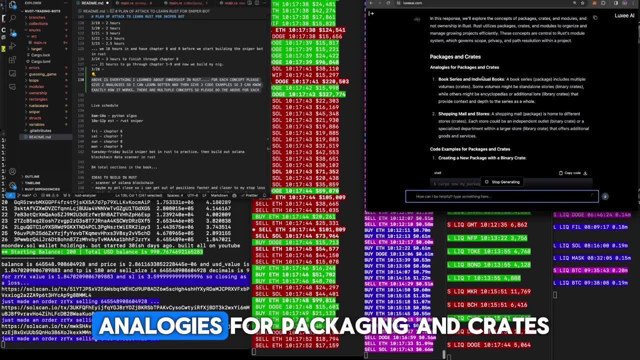 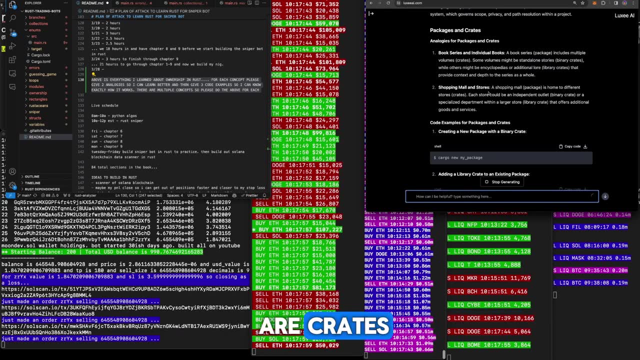 efficiently. these concepts are central to rust module system which can govern scope, privacy and resolution within a project. so packaging and crates, analogies for packaging and crates, book series and individual books. a book series package includes multiple volumes which are crates, though some volumes might be standalone stories which are binary crates, while others might be. 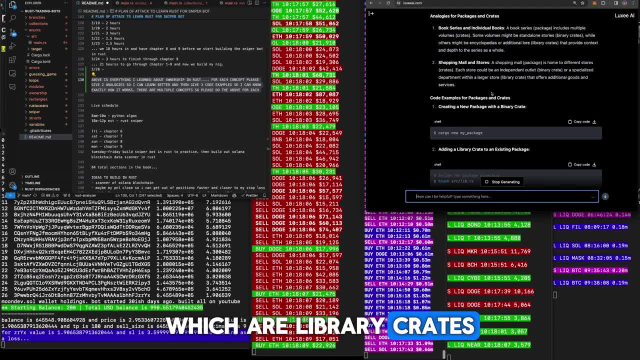 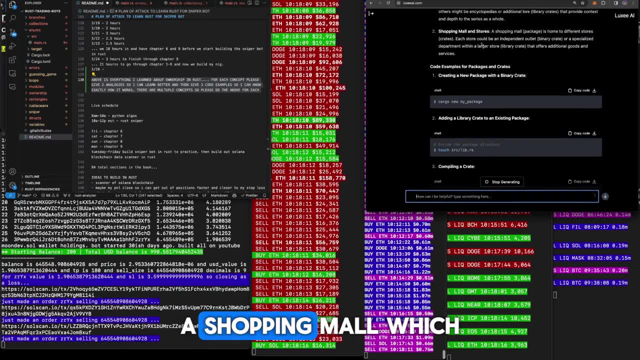 encyclopedias or additional lore, which are library crates. that provides context and depth to the series of a whole shopping mall and stores. a shopping mall which is packaged is home to this book series package includes multiple volumes which are crates, though some volumes might be. 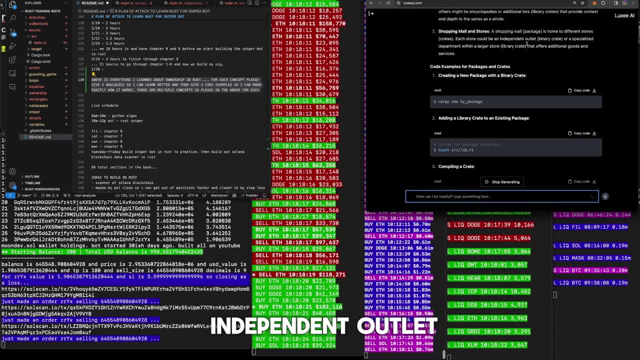 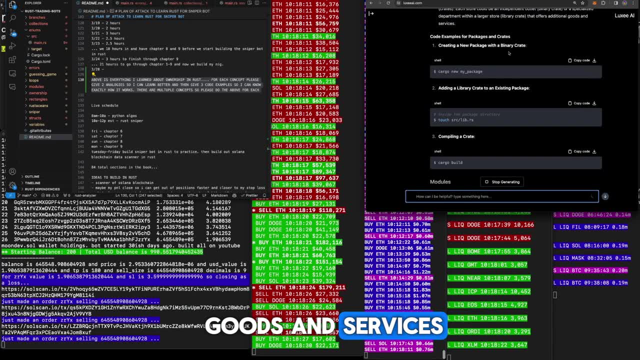 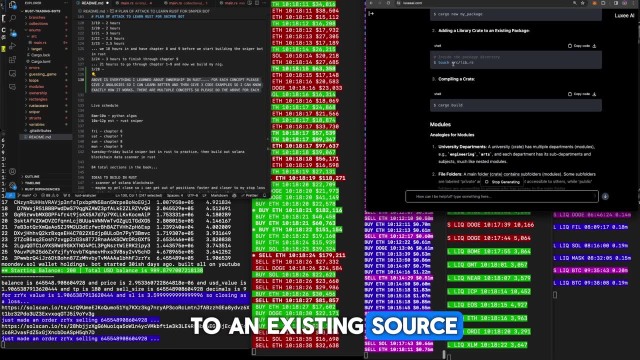 stores, which are crates. each store could be an independent outlet, binary crate or a specialized apartment with a larger scope, which is the library crate that offers additional goods and services. so this is how you create a new package, cargo, new my package, adding a library. create to an existing source, the RS. 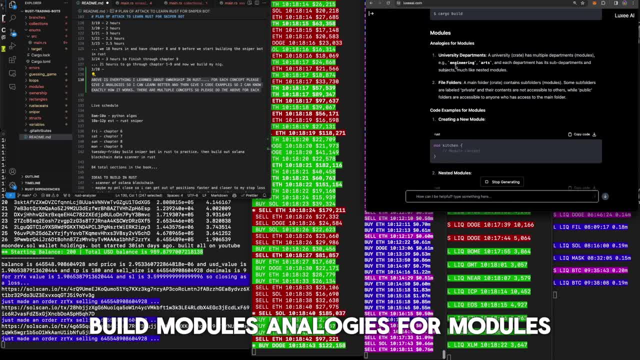 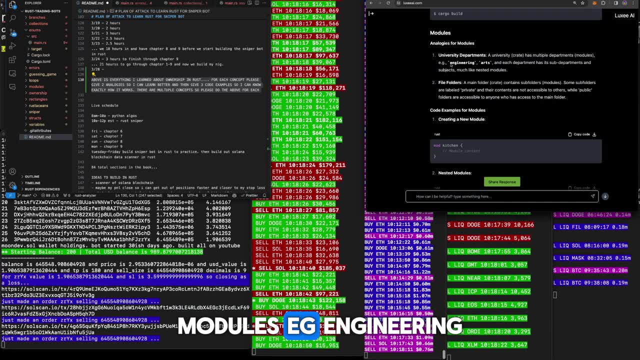 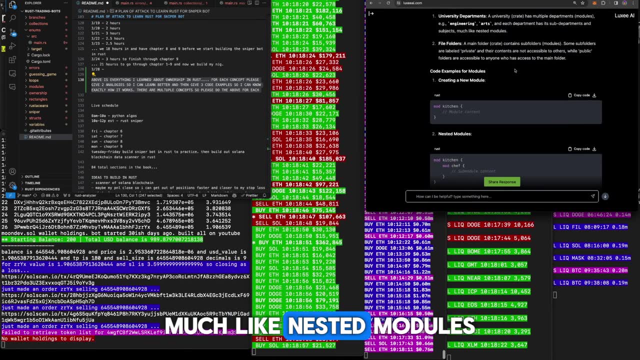 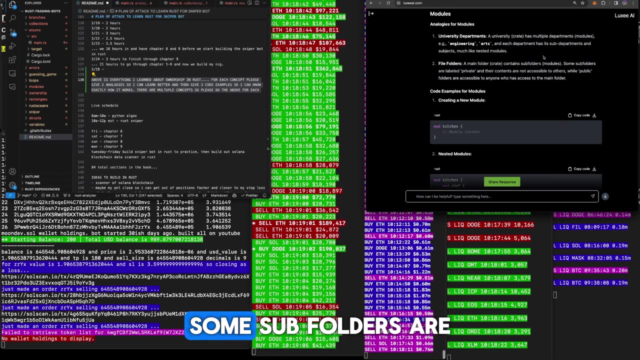 compiling a crate cargo build modules. analogies for modules: University departments. a university crate has multiple departments, modules, eg engineering, arts, and each department has its sub departments and subjects, much like nested modules. file folder folders. a main folder crate contains subfolders which are modules. some subfolders are labeled private and their contents are. 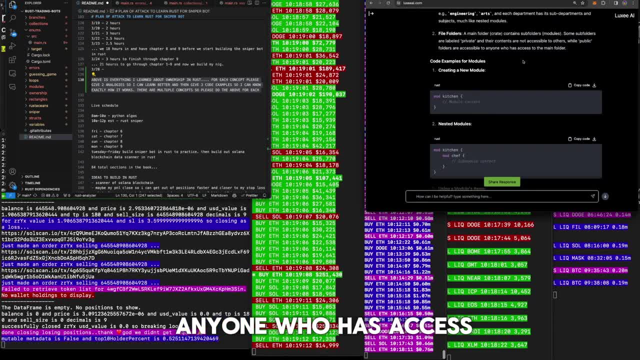 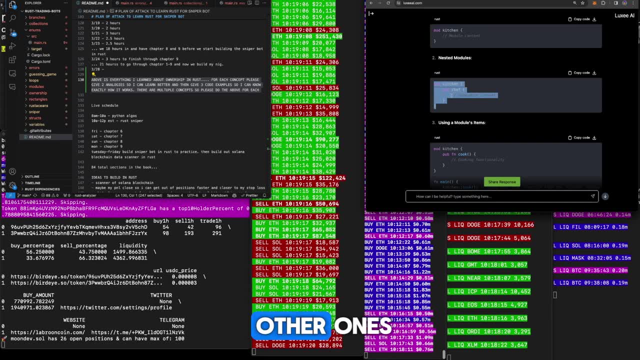 not accessible to others, while public folders are accessible to anyone who has access to the main folder. so create a module like this: you just make a folder and then you create a module like this: you just make a module mod, it nested module, so just like the other ones, you can do a function inside. 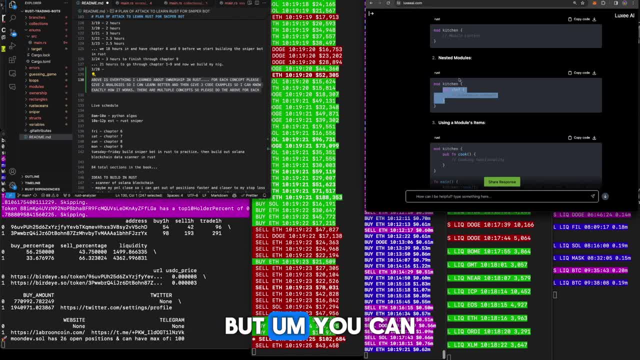 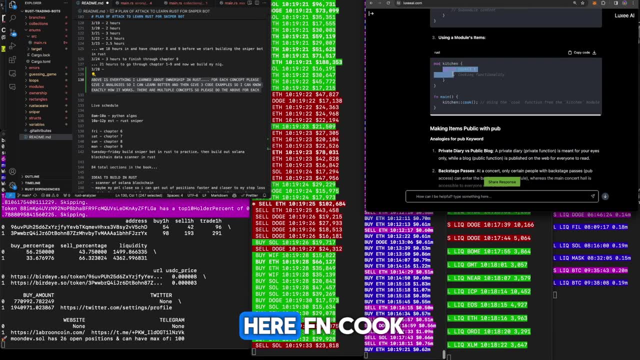 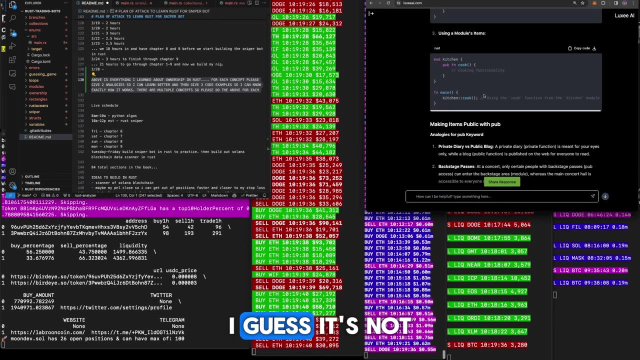 a function, or maybe not a function inside of a function, but you can have these nested things- and that's denoted by these- using the modules items. so mod, so pub here, FN cook, so I can't remember what pub means, but to revisit that again, I guess it's not too important since it's in this modules chapter or this. 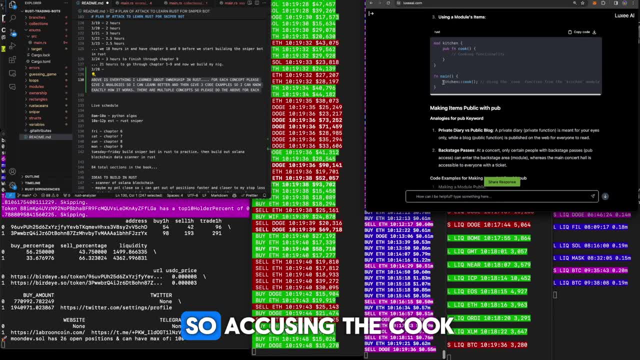 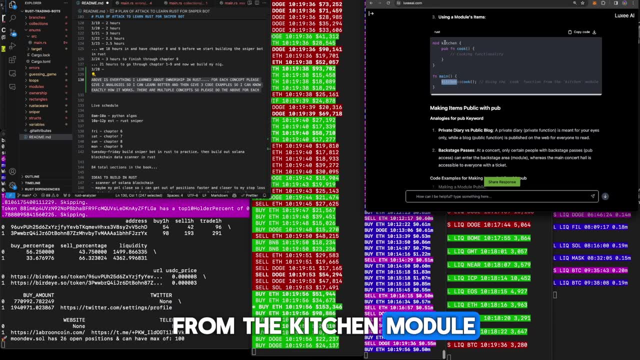 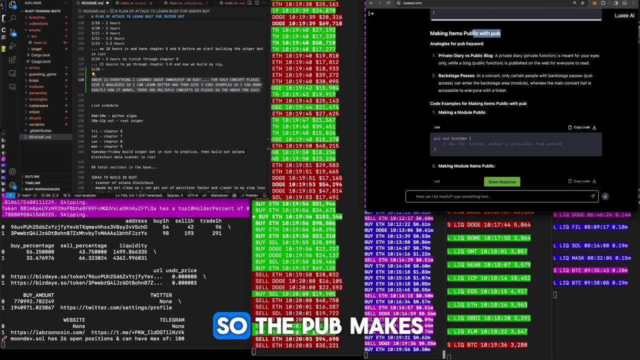 crates chapter which we kind of flew through. so using the cook function from kitchen module. so this is how you call in the function from the kitchen module. so this is saying of a module and then these are the functions. so pub, is that making items public with pub? there we go, so the 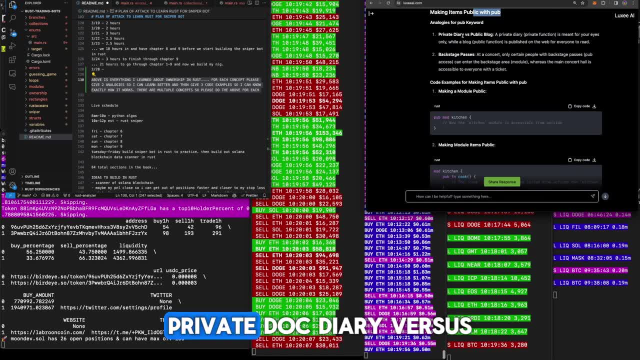 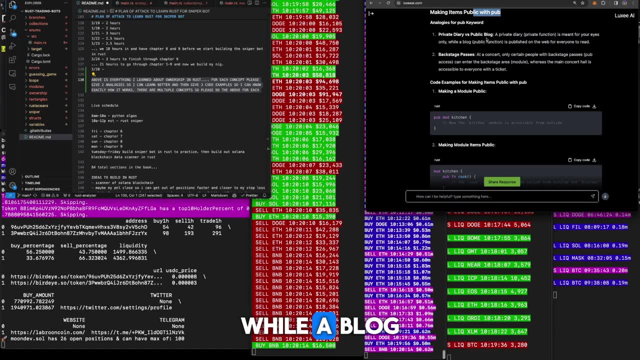 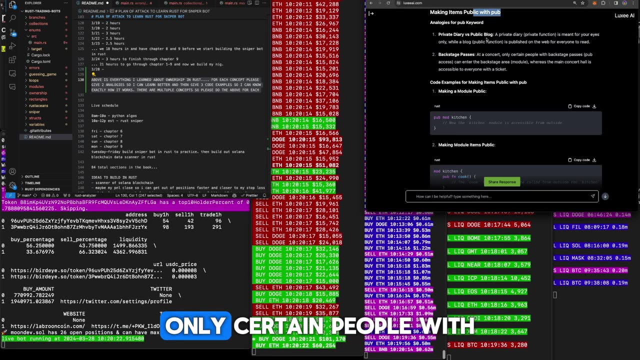 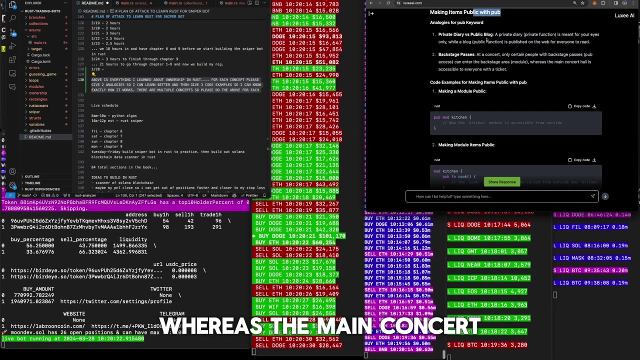 pub makes them public. analogies for pub: keyword: private diary, verse: public blog. a private diary private function is meant for your eyes only, while a blog public function is published on the web for everyone to read. backstage passes a you can enter the backstage area module, whereas the main concert hall is. 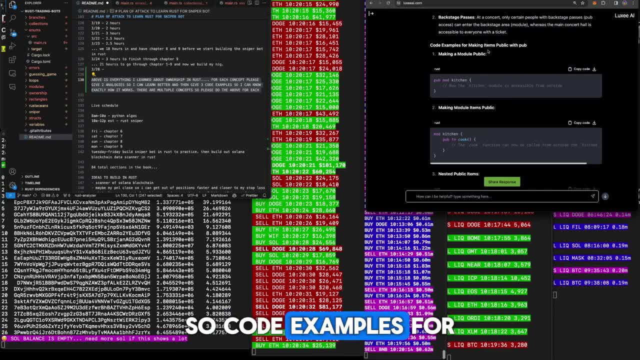 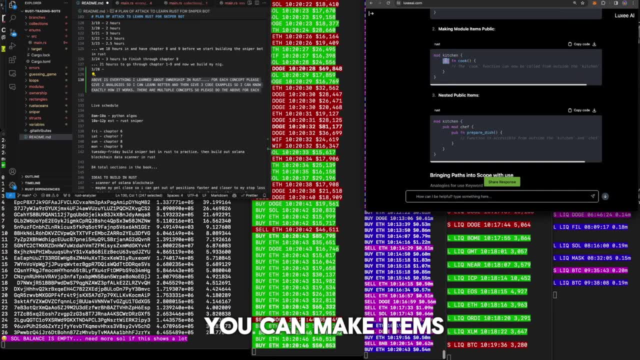 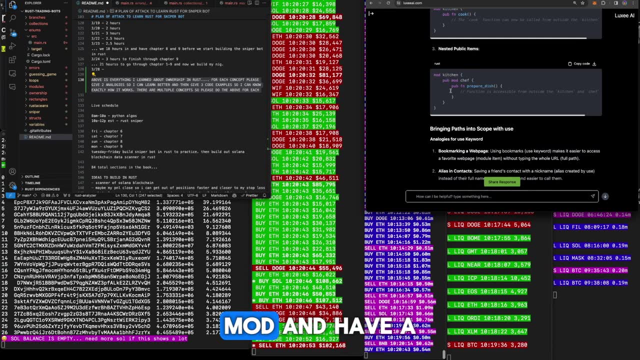 accessible to everyone with the ticket. so code examples for making a items public, so you just put that pub there when you save making a module items public. so inside a module you can make items public, so nested public, so mod, which is a module, and you say pub mod and have a nested one, so one on the 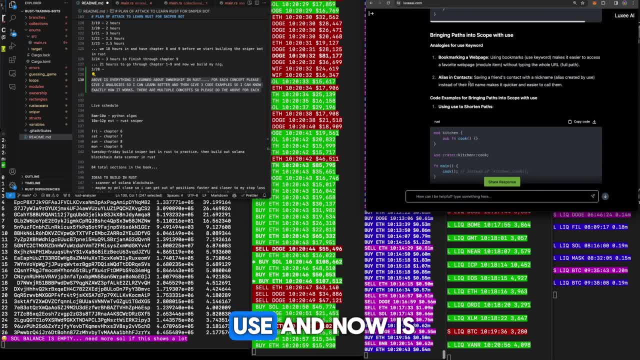 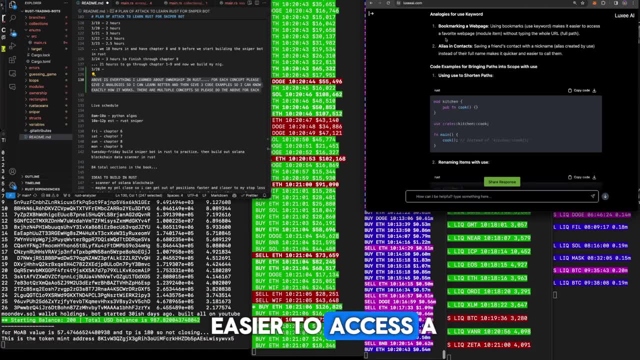 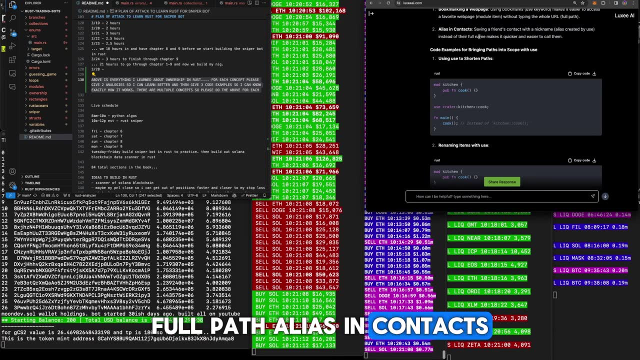 inner side: bringing paths in the scope with use. analogies for use keyword: bookmarking a web page. using bookmarks. use keyword make it easier to access a favorite web page module item without typing the whole url. full path alias in contacts. saving a friend's contact with a nickname alias. 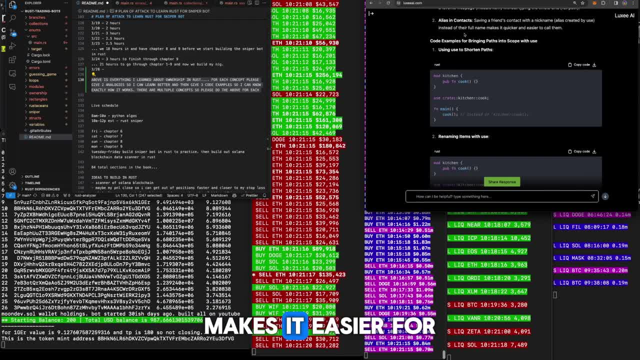 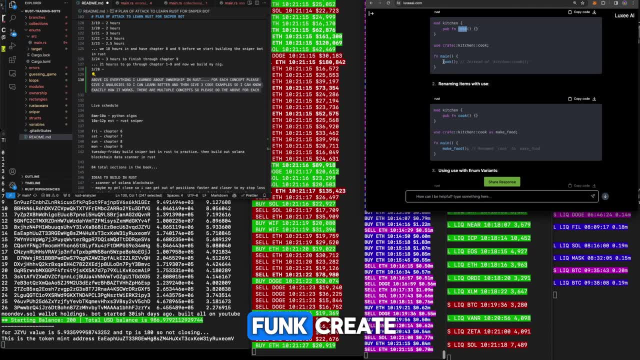 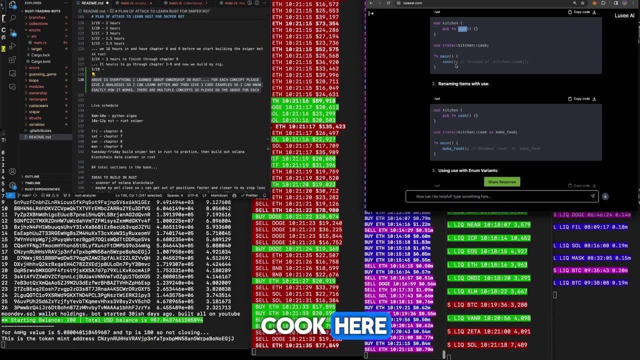 created by use instead of their full name makes it easier for you to call them. so here's some code examples: mod of fn: make a funk, create we're calling the kitchen, then the cook. so inside a kitchen we're actually grabbing that cook here and then you can see I can just use it there. renaming. 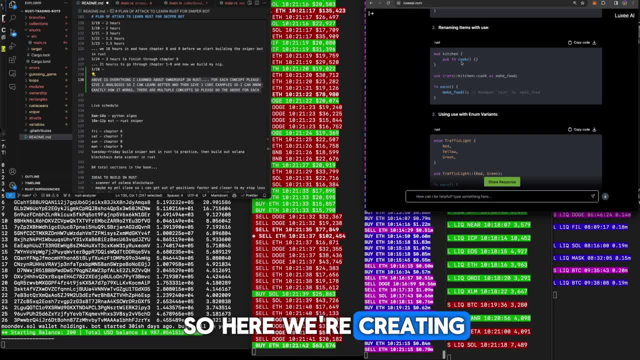 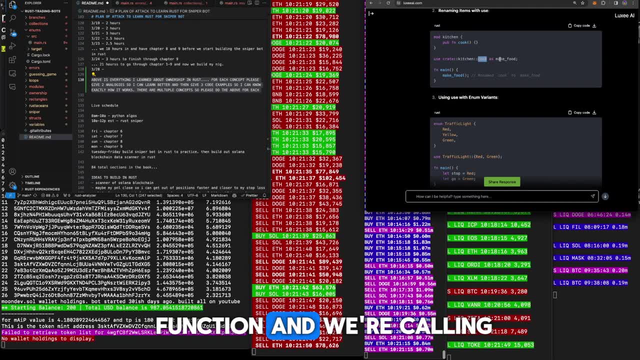 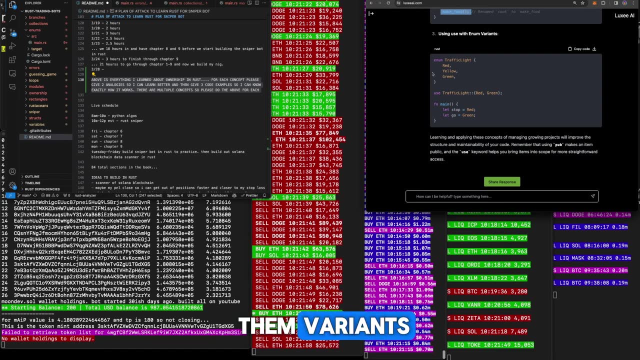 items with use. so here we're creating a module and here it looks like we're saying use crate, we're using the cook function and we're calling it make food, and then we reamed it. so now we just call make food using uh, use with enum variants, so enum- here we set up an enum, like we learned earlier, and then we say: 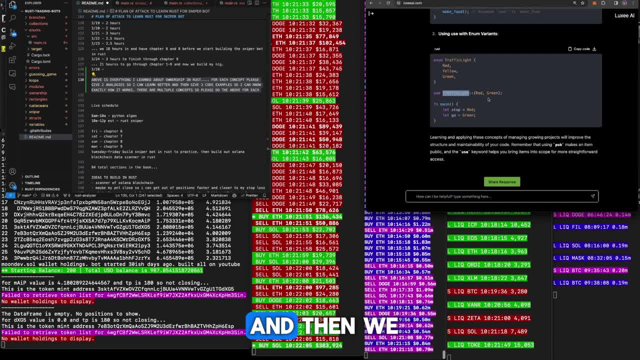 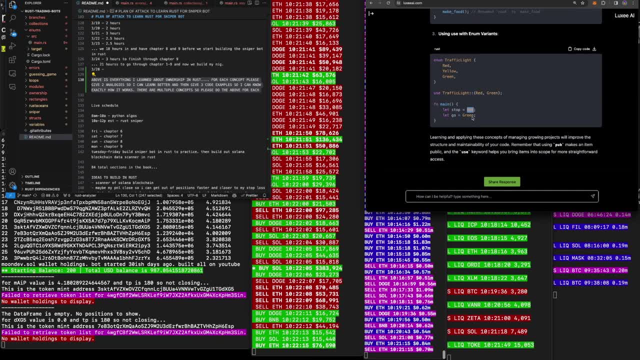 use traffic lights, we're going to use the red and the green, and then we, so we renamed it red and green, and now it says: let's stop equal red, go equal green. not too hard. if you've been here the whole time, then this shouldn't be too hard. I know I'm going fast, but this is intentionally going. 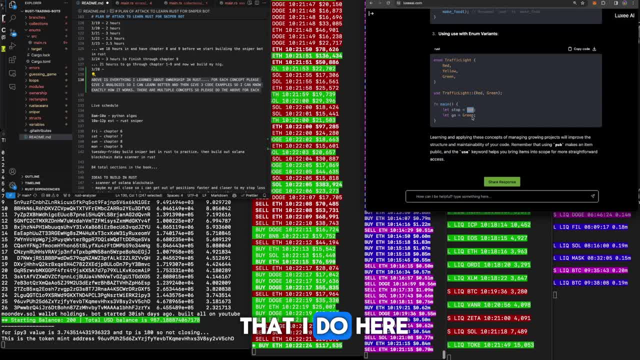 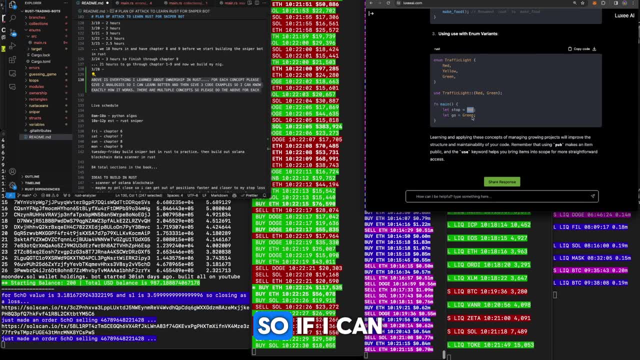 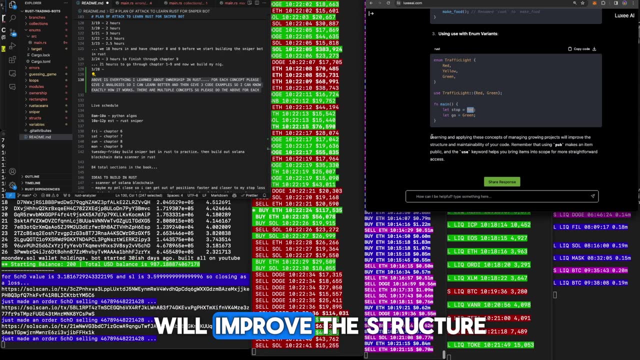 fast. I want to kind of test myself. everything that I do here I am literally needing to do dude- and I'm just a regular dude, so if I can do this, you can do this too. learning and applying these concepts of managing growing projects will improve the structure and maintainability of your 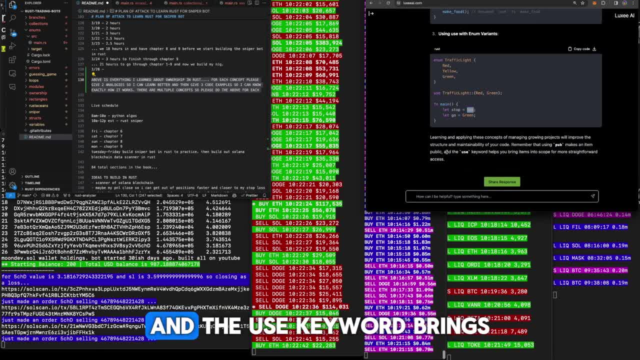 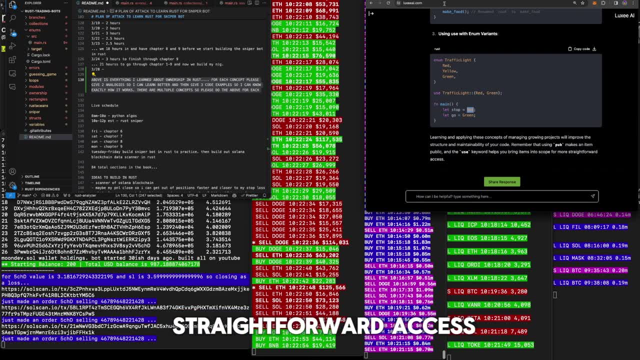 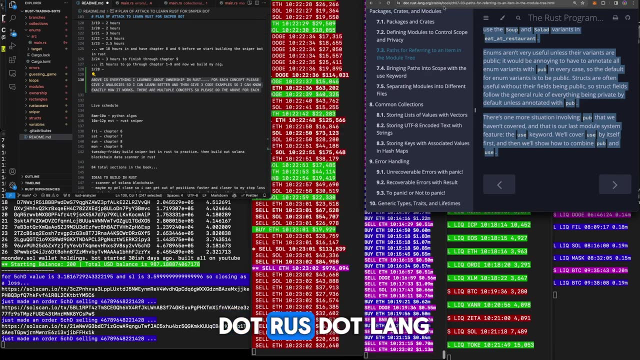 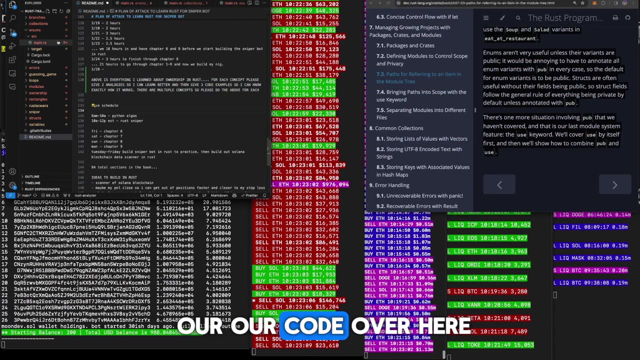 code. remember that using pub makes an item public and the use keyword brings helps you bring items into scope for more straightforward access. nice dude. so I'm just reading from this: chapters these books and you can get it at docrussellcom. this is their official book, so next thing is common collection. so let's go see our code over. 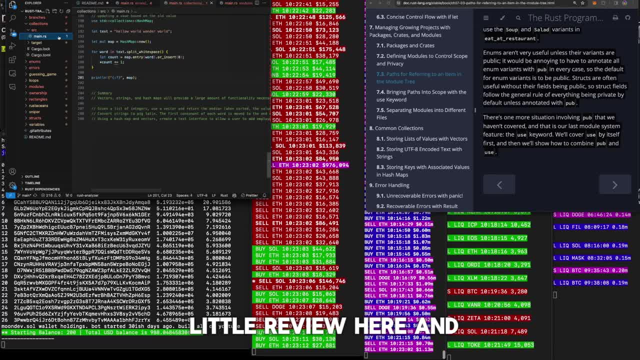 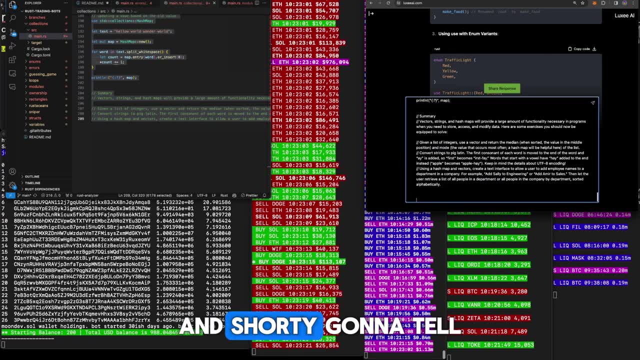 here because we've already done all this. we're just doing a little review here and let's see what it has. you can see it has 200 lines here, so I'm going to paste all that into a little shorty here and shorty going to tell us exactly what we need to do. do everything that we learned. we're 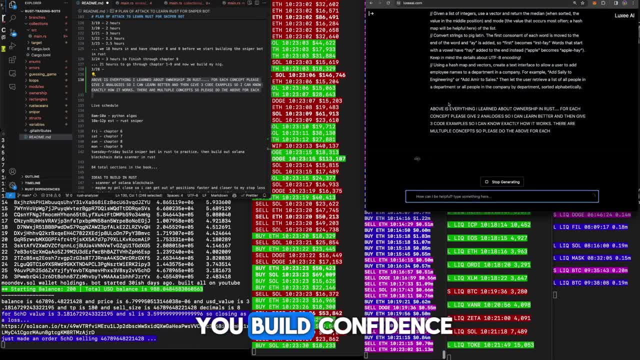 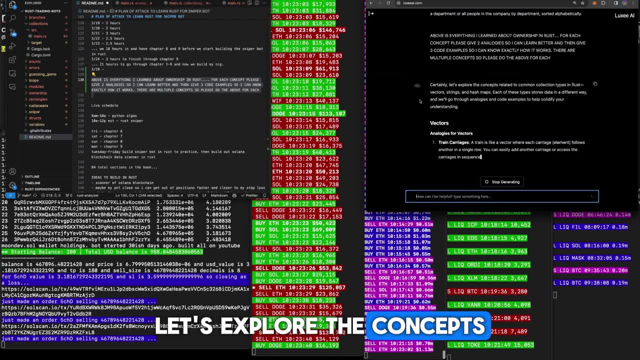 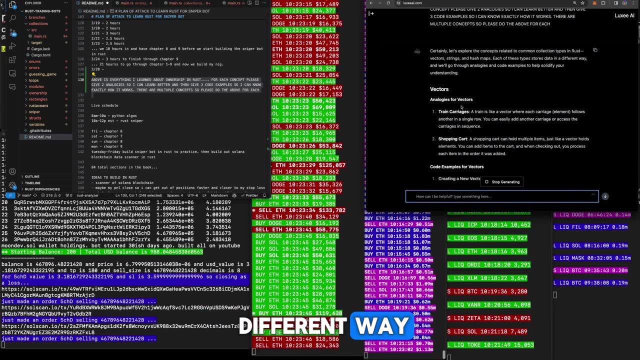 going to go over, because repetition is key in anything. that's how you build confidence in everything. right, if you're scared to do something, it's just because you're not scared. certainly, let's explore the concepts related to common collection types and Russ vectors, strings and hash maps. each of these types stores data in a different way, and we'll go. 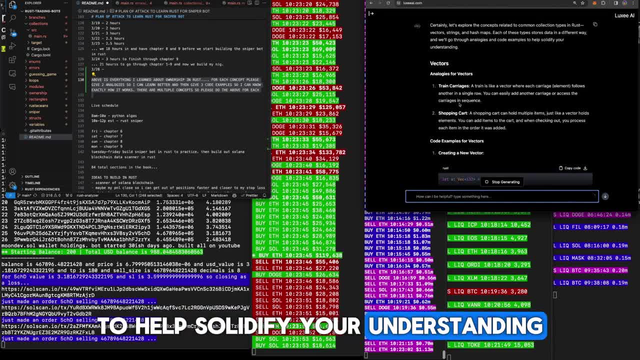 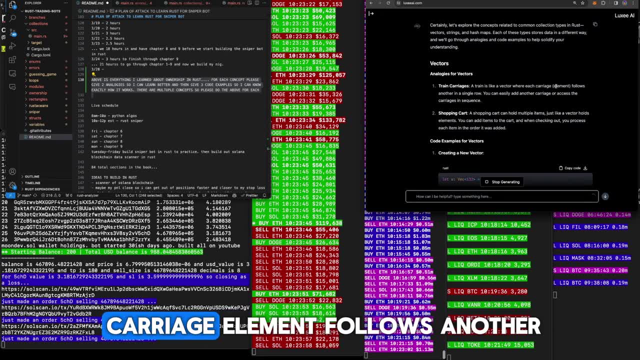 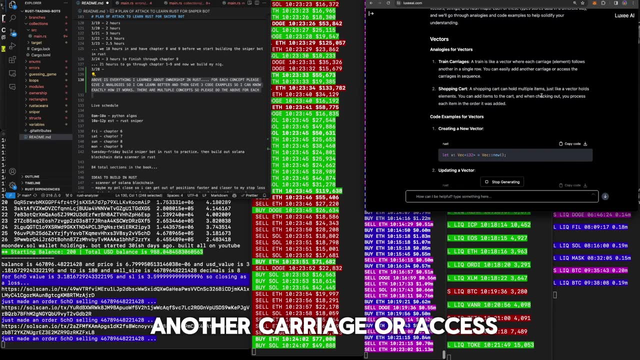 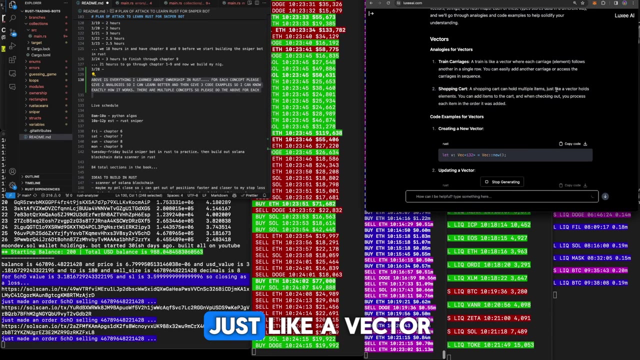 through analogies and code examples to help solidify your understanding. vectors: analogies for vectors: train carriages: a train is like a vector, where each carriage element follows another in a single row. you can easily add another carriage or access the edges in sequence. shopping cart analogy: a shopping cart can hold multiple items, just like a vector. 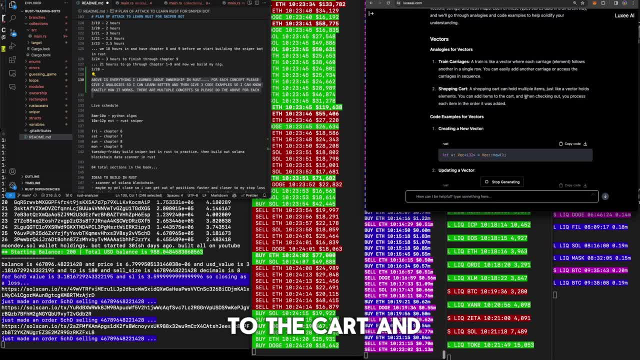 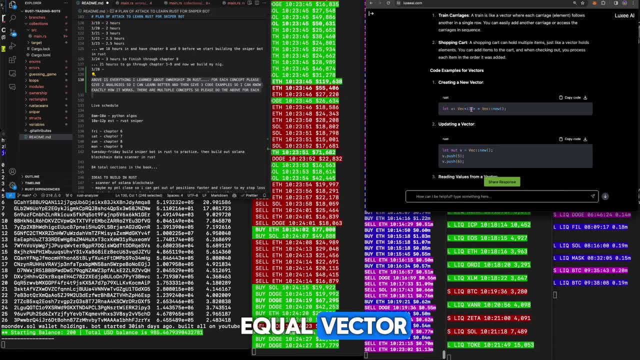 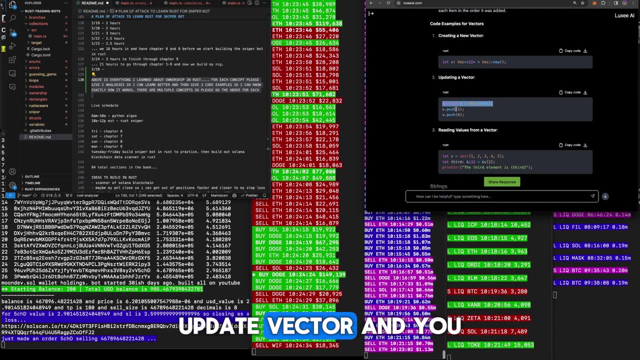 holds elements. you can add items to the cart and when checking out you process each item in the order it was added. so, creating a vector, you say let v equal vector, so you're saying what it is. and then you say vec dot new. then updating the vector has to be a mutable update vector and you 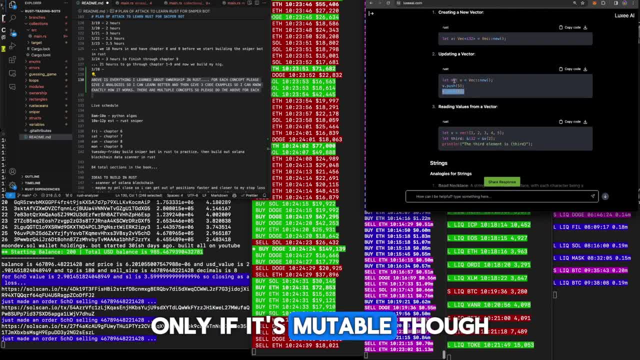 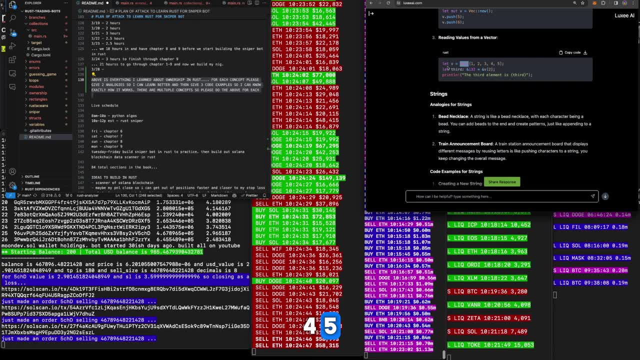 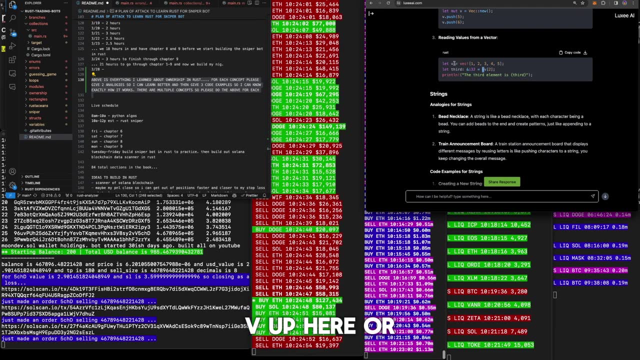 could say: hey, let's push the five and push the six only if it's mutable though, reading values from a vector. so let v equal a vector of one, two, three, four, five. then let third equal. it's a number, it's a changeable number and it's v changeable, v up here or not changeable. sorry, borrowing a v. 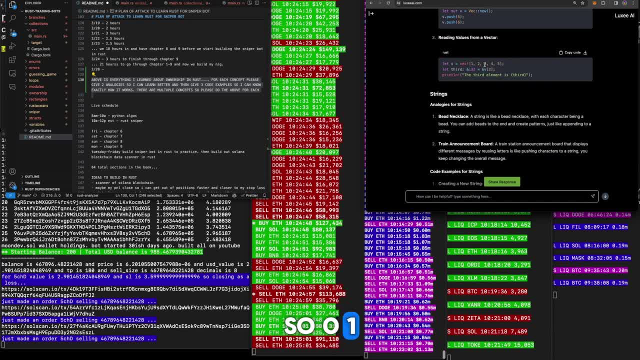 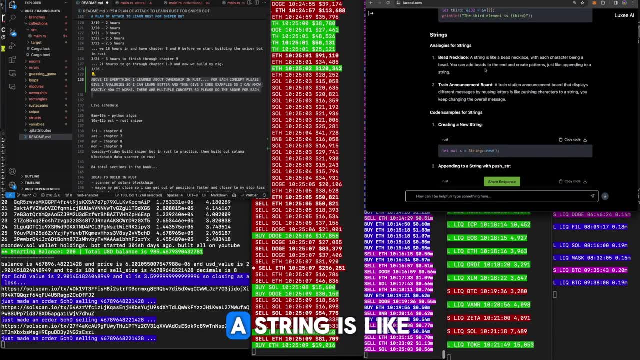 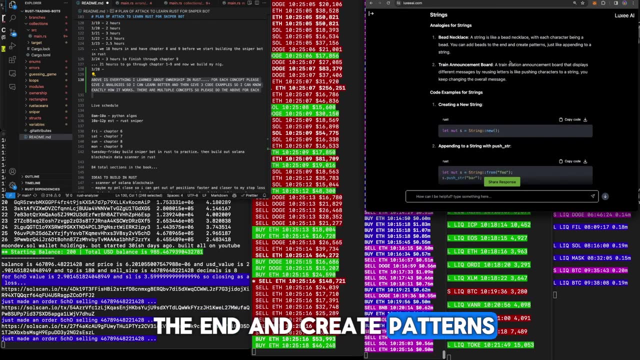 uh and this and sign equals. borrow v2. so zero one. two is the third right, because we start with zero strings. analogies for strings: bead necklace. a string is like a bead necklace, with each character being a bead. you can add beads to the end and create patterns, just like appending to a string. 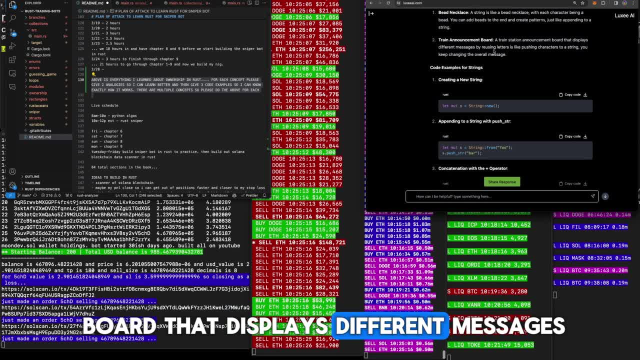 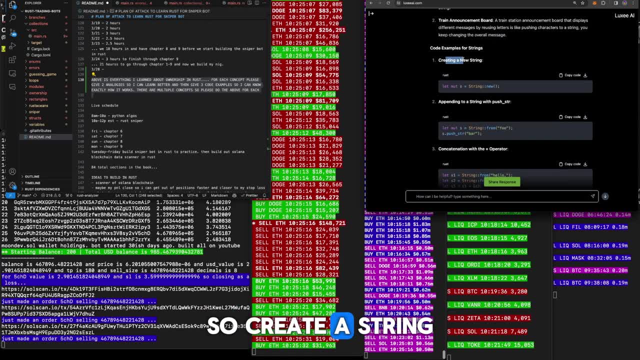 a train station announcement board that displays different messages by reusing letters is like pushing characters to a string. you keep changing the overall message, so creating a string here you can see. this is how you create a string and notice that it's mutable because we put the 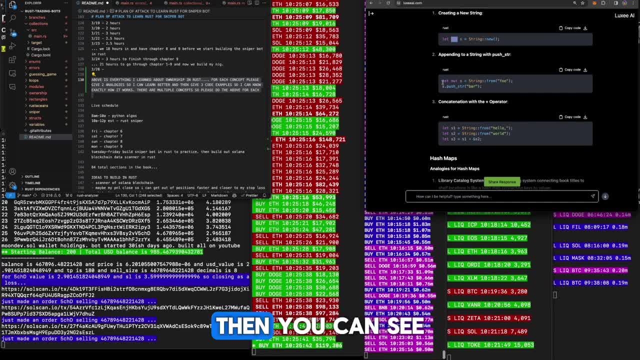 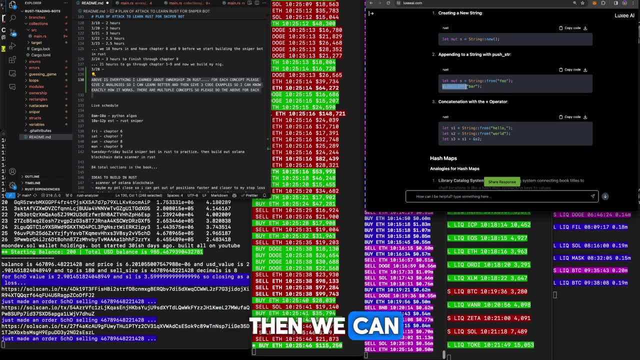 mute keyword and in rust nothing is mutable unless you put the mute there. then you can see we're saying the same thing here, for us here, uh, but we're saying the string is so the string is foo, and then we can. we can push the string, meaning we can append. if you're coming from, 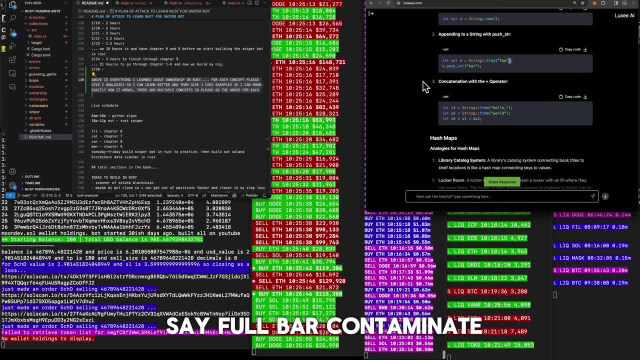 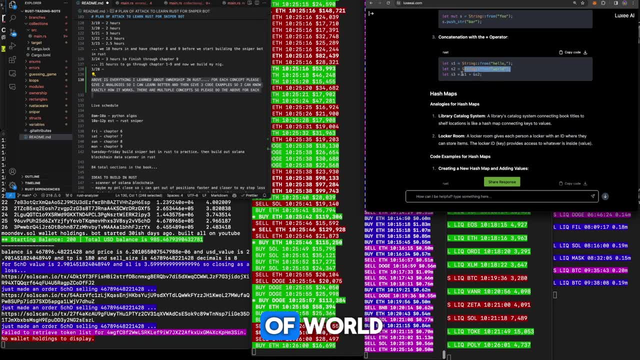 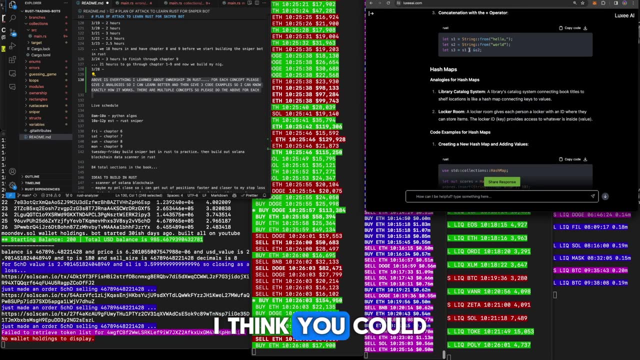 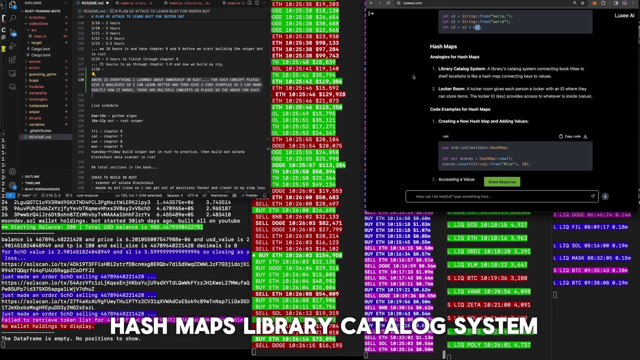 python bar. so now it should say foobar concatenate with the plus operator. so s1 is a string of hello, s2 is a string of world, and we can say s1 plus changeable s2 equals hello world. i think you could also do regular s2, if i'm not mistaken. but hash maps- analogies for hash maps- library catalog. 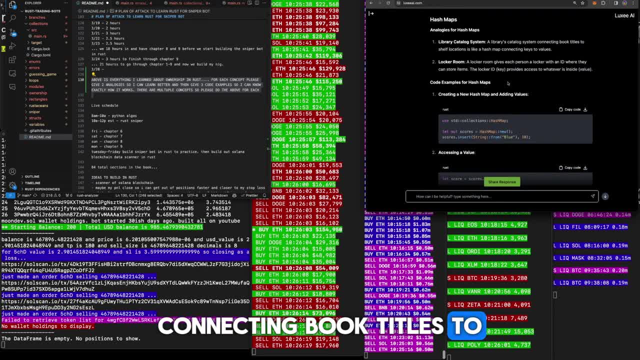 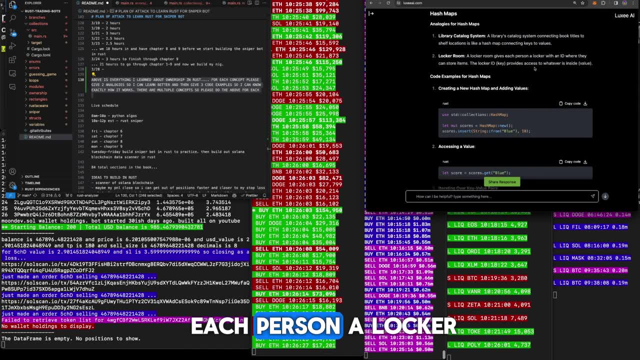 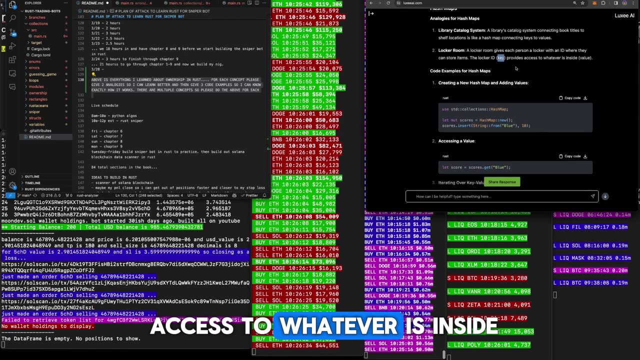 system, a library's catalog system. connecting book titles to shelf locations is like a hash map connecting keys to values. a locker room gives each person a locker with an id where they can store items. the locker id, which is the key, provides access to whatever is inside, which is the value. 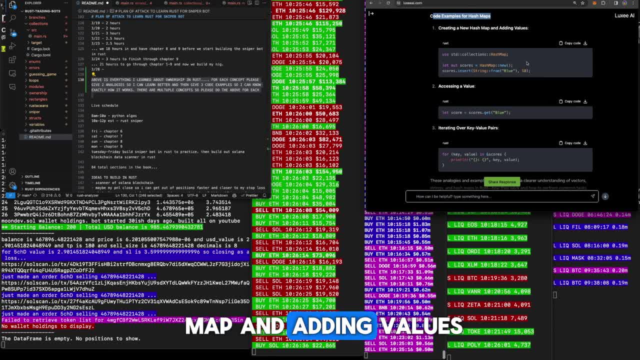 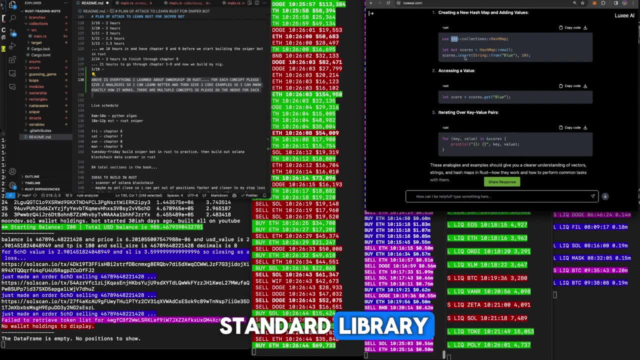 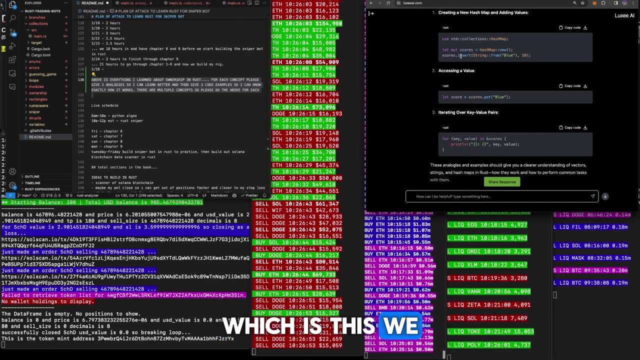 code examples for hash maps: creating a new hash map and adding values. so you can see we're going to use. so we're using hash maps from the collection standard library and we're saying mute, changeable scores equal the hash map. a new hash map and then we can say scores, which is this we insert. insert the string. 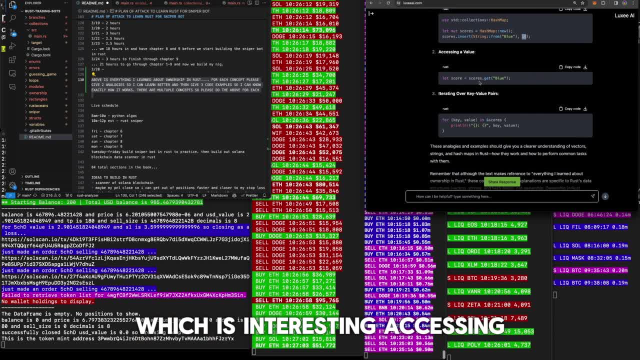 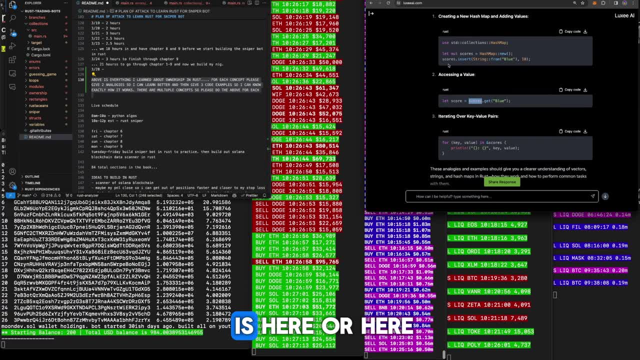 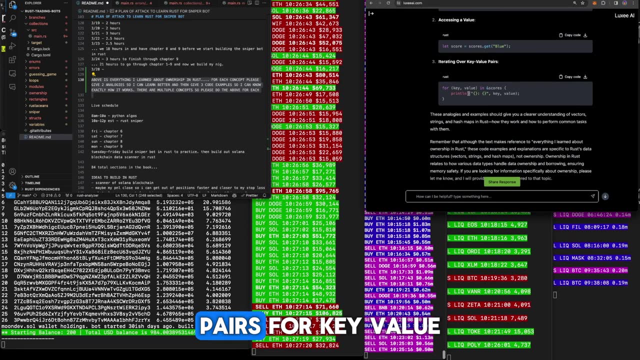 blue and also 10, which is interesting, accessing a value. let's score equals scores. dot get blue, so scores up here is here or here, and then it gets oh blue, so it'd be 10.. iterating over key value pairs for key value in scores: changeable scores. borrowable scores. print. 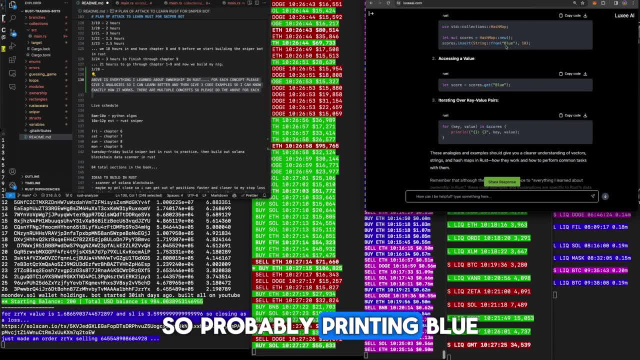 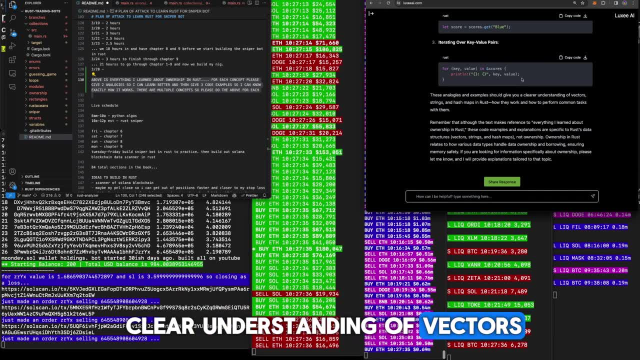 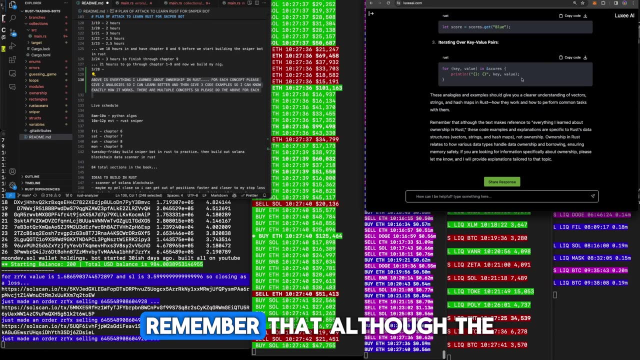 ln, so it prints in the key and the value, so probably printing blue and 10.. i'm not a pro at this one. yet these analogies and examples should give you a clear understanding of vectors, strings and hash maps and rust, how they work and how to perform common tasks with them. remember that. 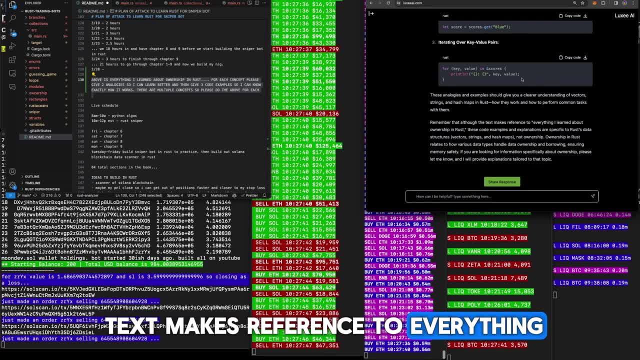 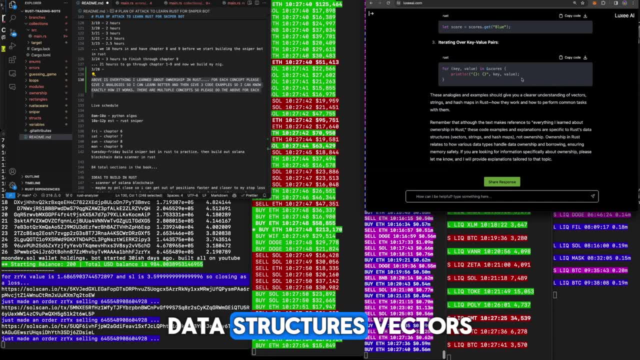 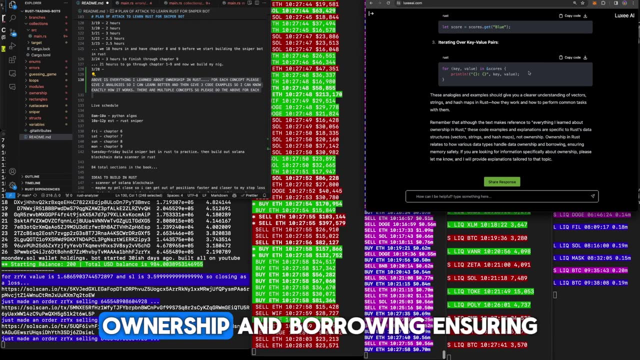 x makes reference to everything i learned about ownership and rust. these code examples and explanations are specific to rust- data structures, vectors, strings and hash maps, not ownership. ownership and rust relates to how various data types handle data ownership and borrowing, ensuring memory safety. if you're looking for information specifically about ownership, please let me know. 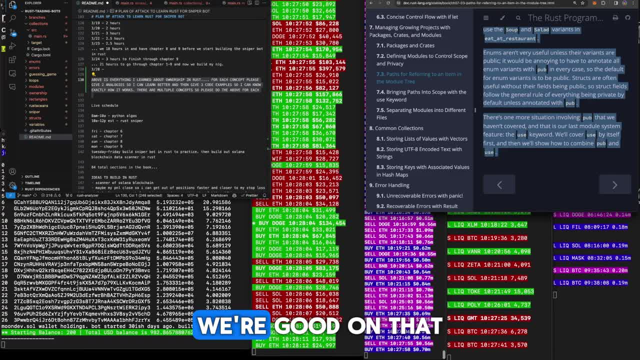 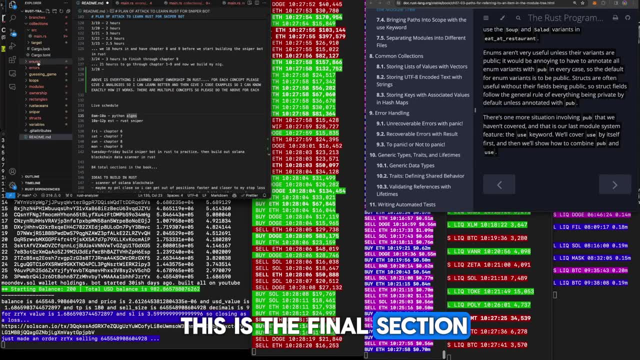 and i'll provide some tailored solutions. no, dude, we're good on that. we already did that. so we did our retest my collections. we just went through it, dude. and now error handling. this is the final section. so you see, we're flying through this. i like how we learned this. 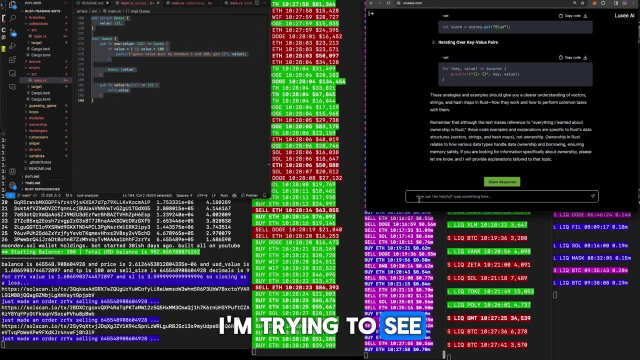 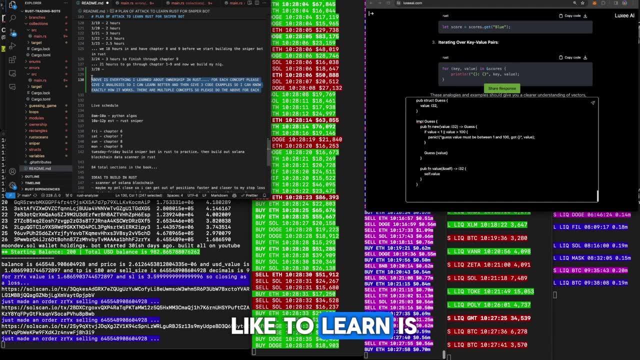 i know i'm going fast through this, but i'm challenging myself. i'm trying to see if i actually understand this and so far i do. there's a couple of things i'm not super solid on, but the way i like to learn is just read the book or watch the videos you know, like if i were to. 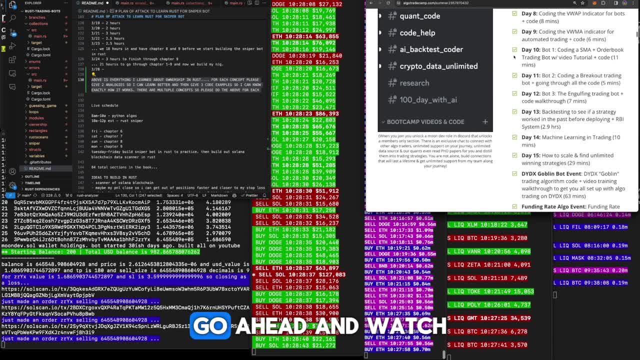 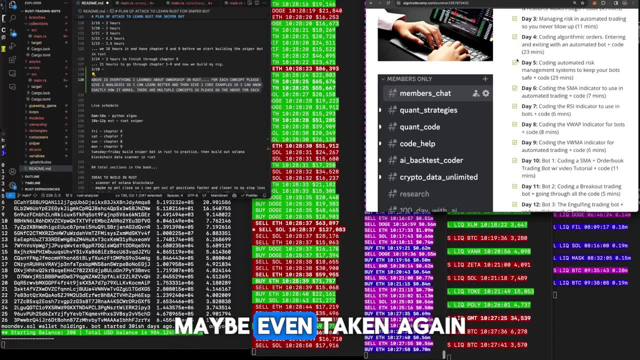 take my boot camp. i would watch all the videos one time through and then i would go ahead and and then type all the code, so just how I like to learn, and then I would see, maybe even taking again and see if I actually understand it. so everybody learns a. 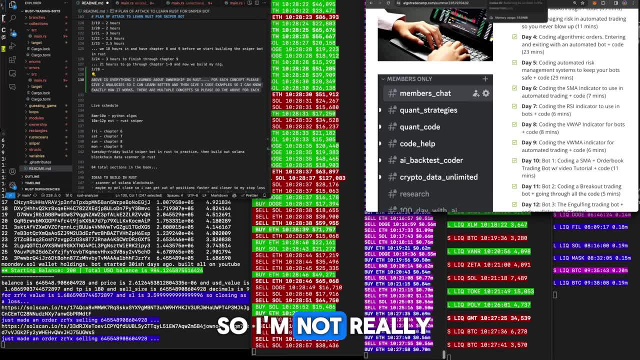 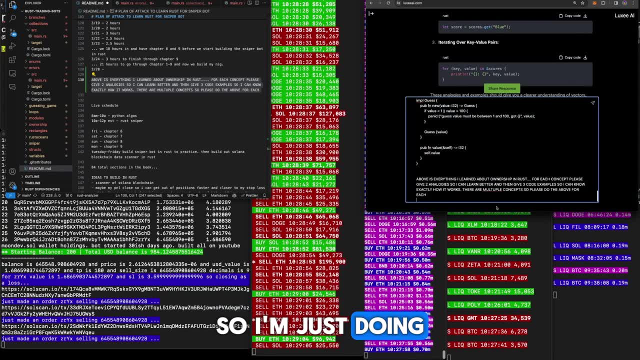 little bit differently. I'm a visual learner, so I'm not really a huge reading learner, but this is supposed to be the best way to learn Russ, so I'm just doing what we did. I can get you caught up to speed with me. everything I teach is in. 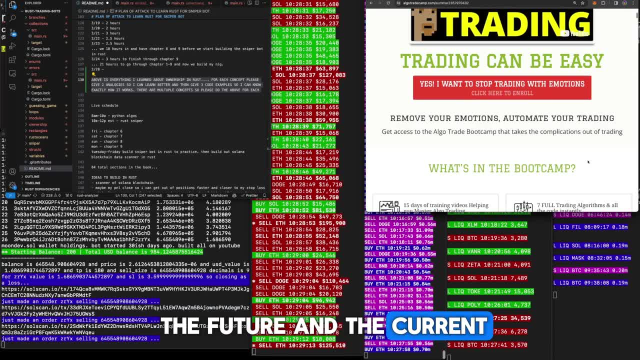 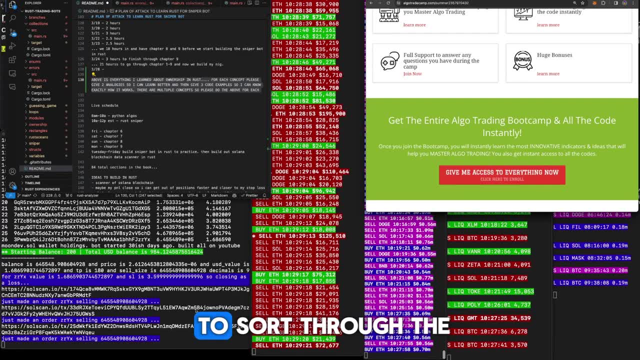 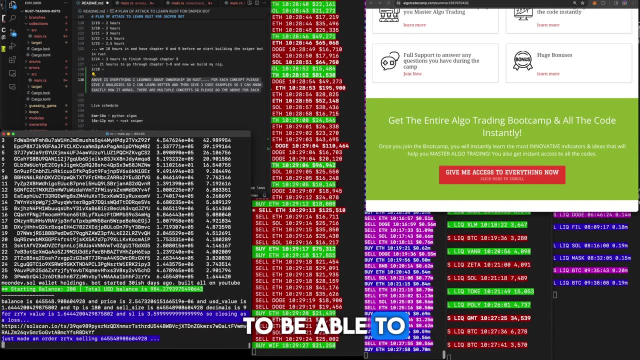 Python. I think Python is the future and the current and all you really need to automate your trading again. the reason I'm learning rust is because I want us. I want to be able to sort through the Solana blockchain, because I have this Solana sniper that's actually doing quite well, so I want to be able to take 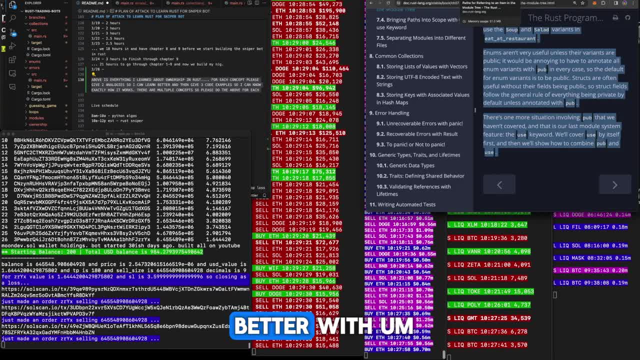 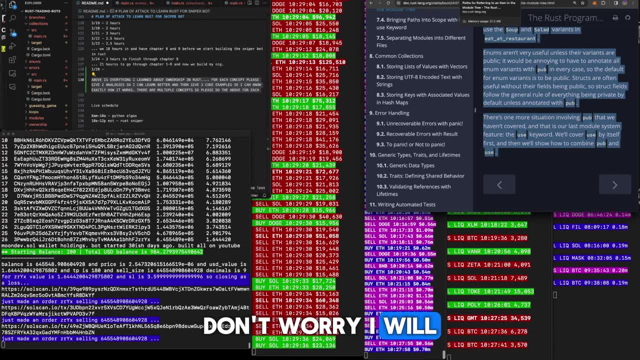 control of some of that and see if I can make it do better with grabbing stuff from the Solana blockchain. and if I do figure this out, don't worry, I will share all the api's with you. everybody in the discord will have free access to you. 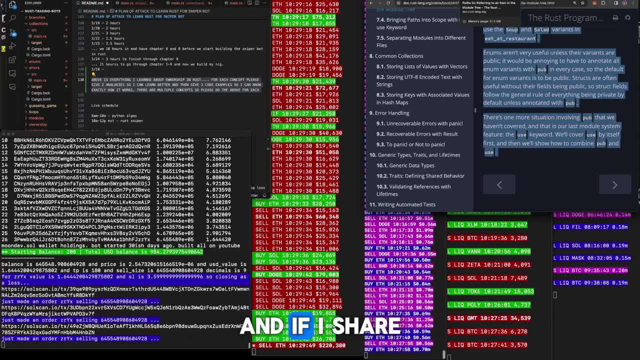 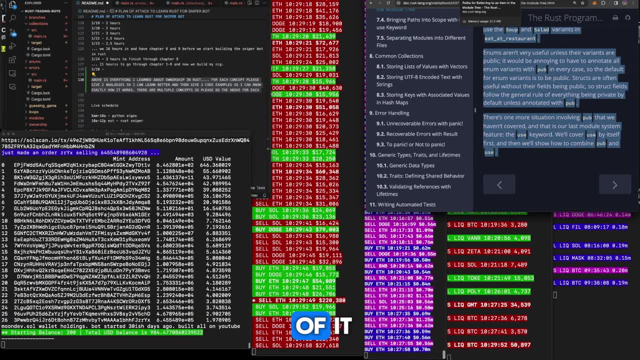 um, all the data that I have, because I believe code is a great equalizer and if I share absolutely everything I do, then essentially, hopefully somebody learns how to code based off of it. you know what I'm saying and I'm really starting to love this community. I know I talk about this so often, about how this is. 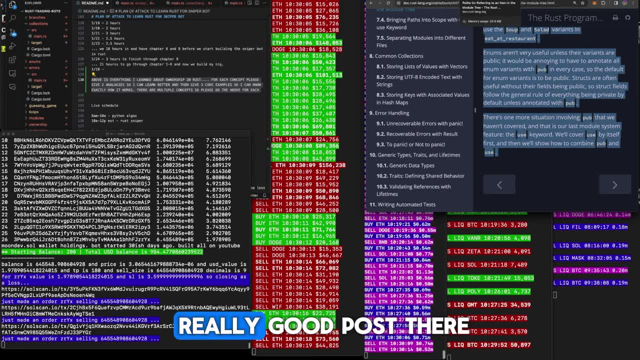 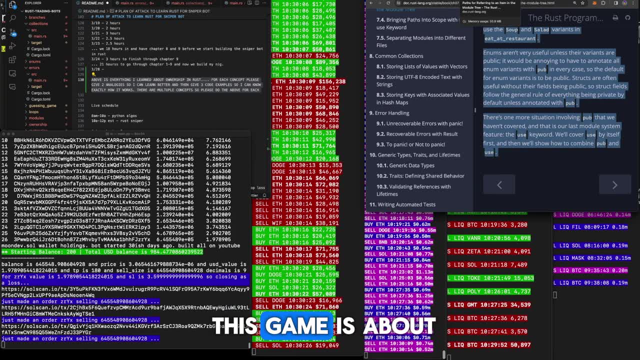 not a get rich quick, but I'm just looking at Discord right now and somebody made a really good post. there's really a few good posts here today. one guy said delayed gratification is that's what this game's about, and it's so true. so people are really starting to. 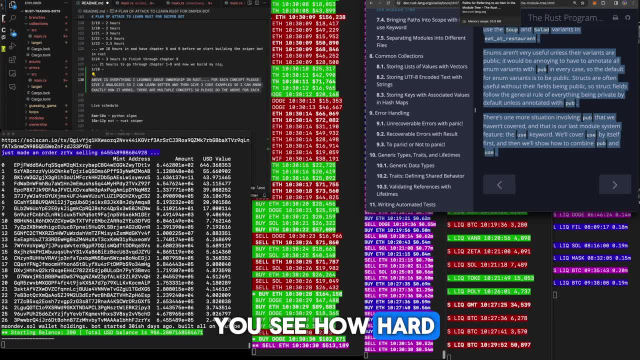 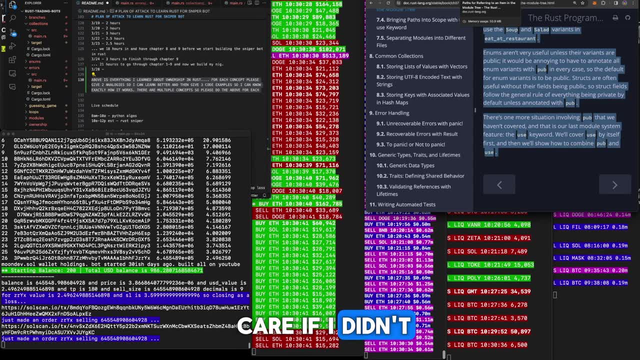 chain that this is not a get rich Quik, this is hard work. you see how hard I work, dude. you see how hard like I go every single day, no matter what, sick, tired, whatever, I don't care. if I still didn't sleep last night, I'm still going. 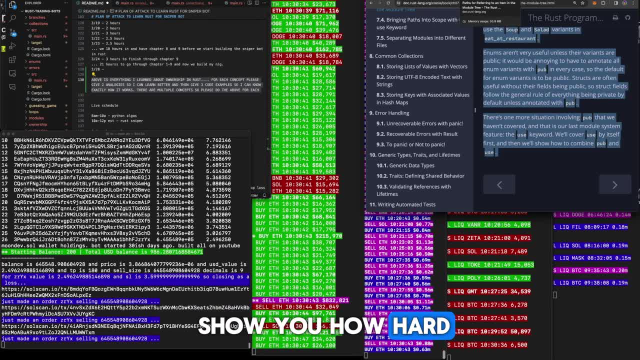 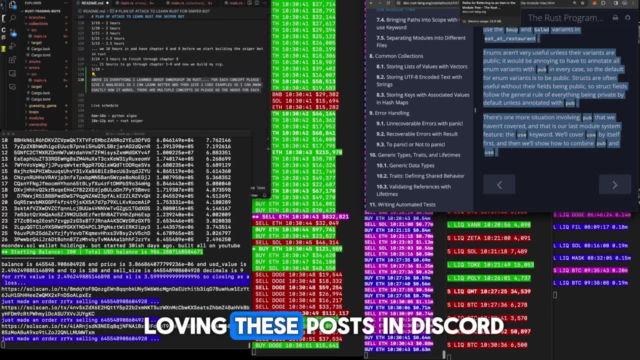 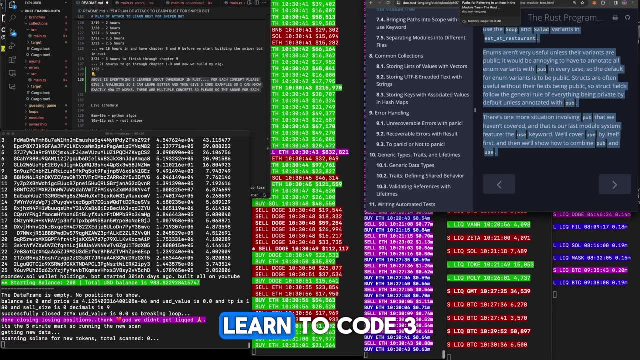 to be here because I want to show you how hard this is. I want to show you that algo training is not easy. it's not something you just plug and play. but I'm really loving these posts and Discord. somebody said there is no get rich quick strategy if you put in the work. 1: learn to trade. two: learn to code. 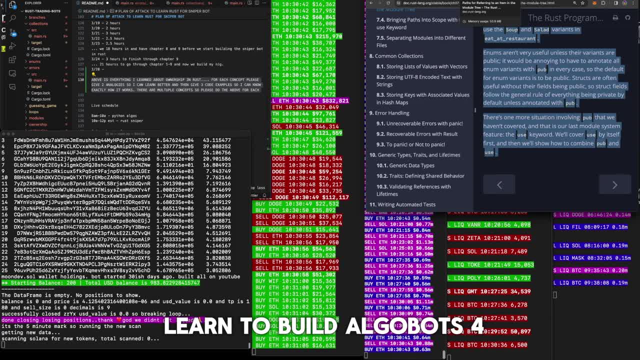 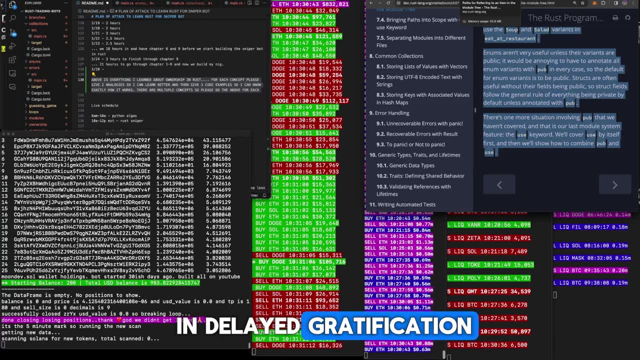 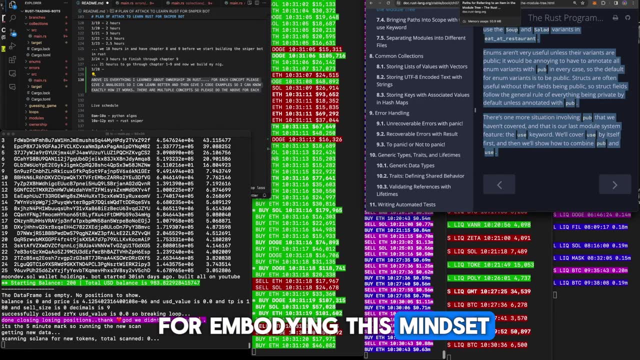 three: learn to build algo bots. four: learn to make strategies. five: learn to be patient. a whole lot of other learning will result in delayed gratification. that is so true. so i really uh, thank you guys, thank you so much for embodying this mindset of- hey, this is not like a givers. 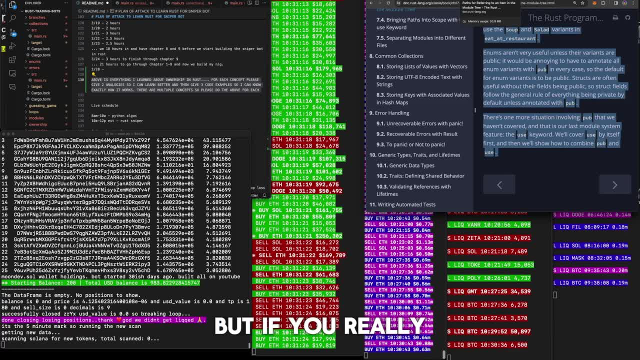 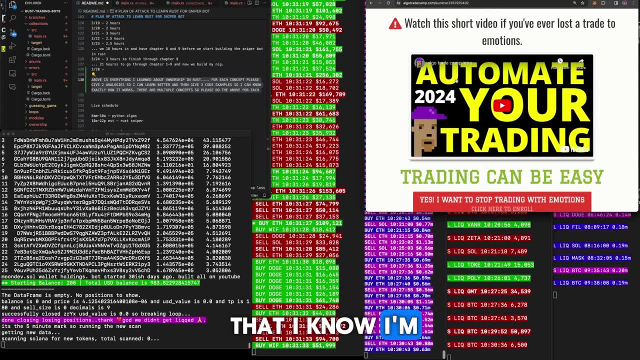 quick. it's not something super easy to do by any means, but if you really are struggling with emotions or you really want to just automate your trading, i show you everything that i know- and i'm not the best in the world, but i see nobody else sharing this information, so you know. 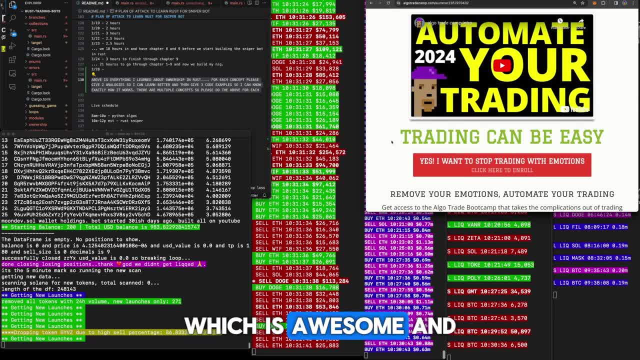 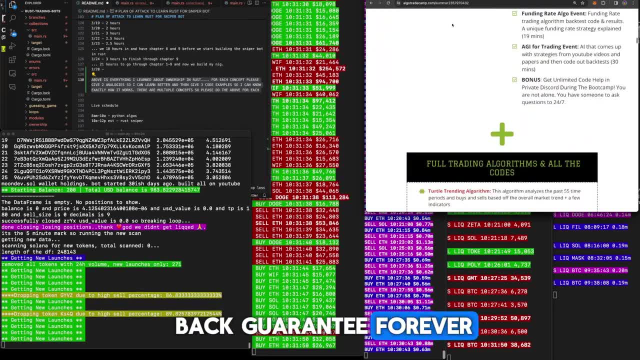 if you can get caught up to me, then you you could probably crush me, which is awesome, and that's what i try to do in the boot camp. i show you step by step how to do all of this in python, and there's 100 money back guarantee forever. so let's go ahead and finish this. one last thing and rust. 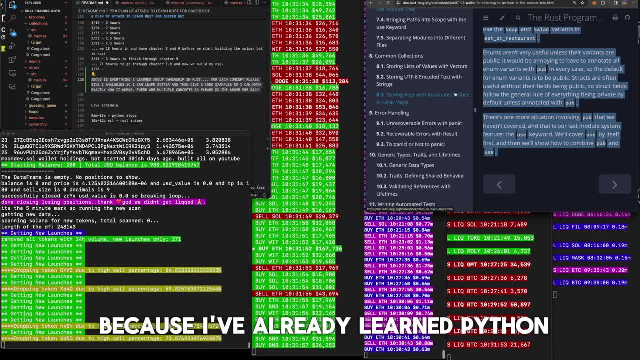 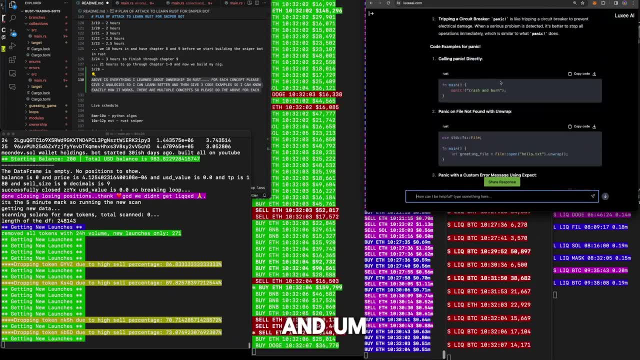 again. you don't need rust. i'm just learning it because i've already learned python and i've got good things going here, dude, so let's go ahead and see what she said about this here. and this is just error handling. i think a lot now that we have a good core and a base of. 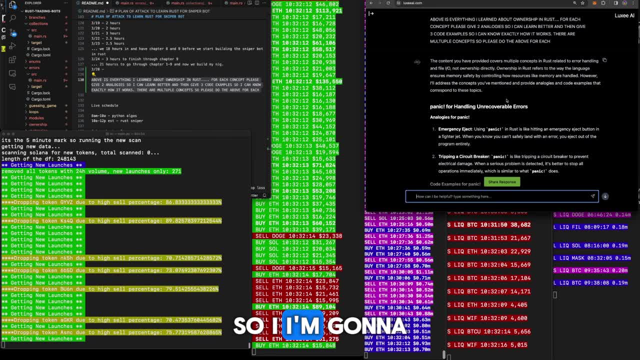 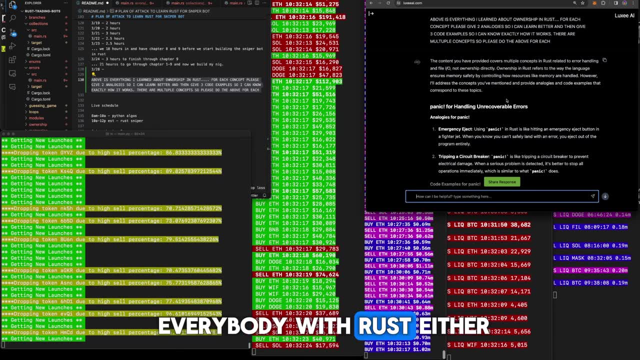 rust. now we can start building, so i'm gonna think of a project to build with you here in rust and i'll come back. i don't want to overload everybody with rust either, so that's why i'm not like doing too much here. the content you provided covers multiple concepts and rust. 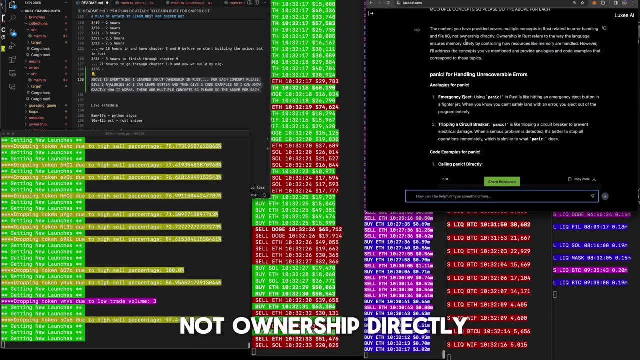 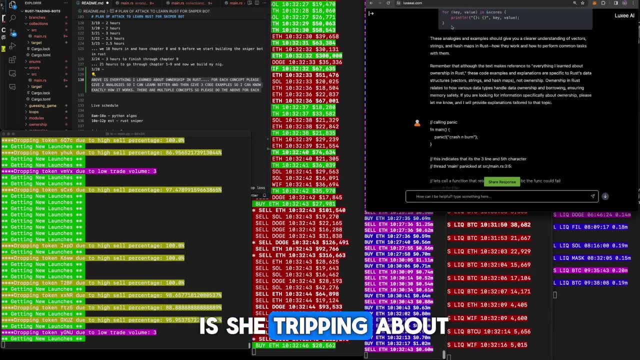 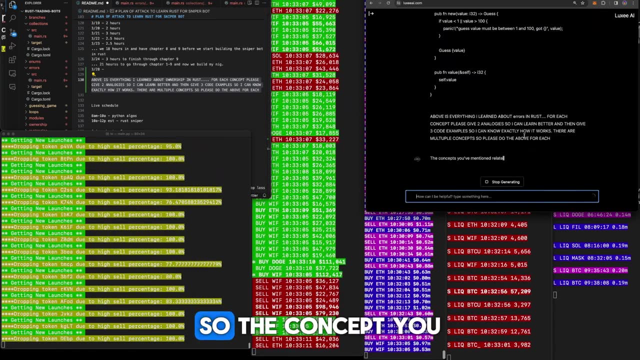 related to error handling the file io, not ownership directly. oh, my goodness, my bad. that's why i was like: what is she tripping about? why does she keep talking about ownership? it's because i said it in the freaking thing about all right, there we go. so the concepts. 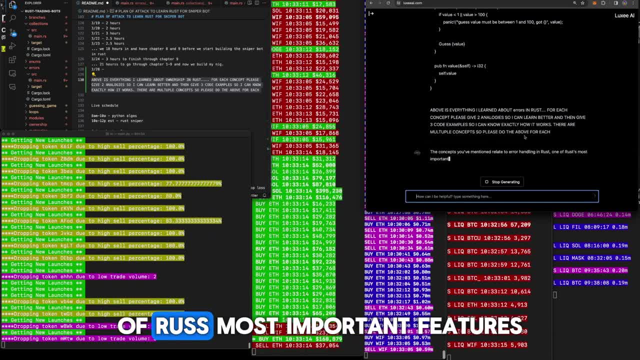 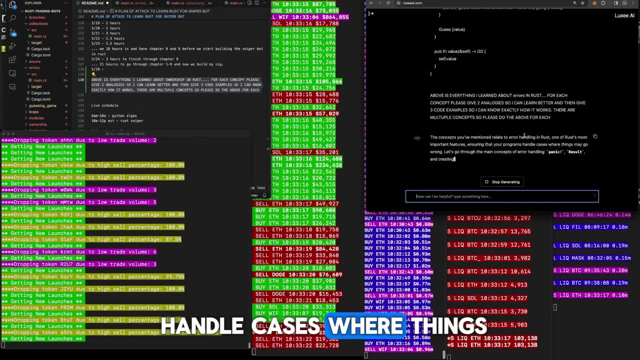 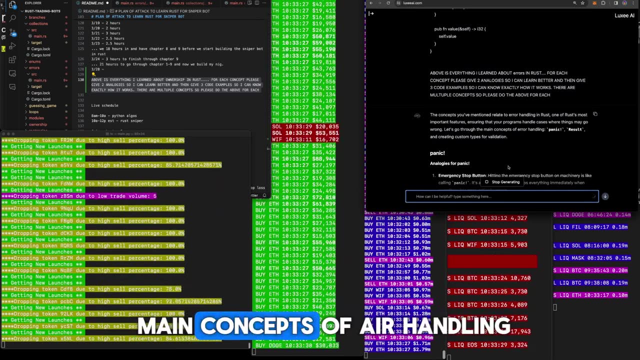 you mentioned relate to error handling and rust. one of rust's most important features. ensuring that your programs handle cases where things may go wrong, lets you may go wrong. let's go through the main concepts of error handling, which are the main concepts of error handling, which are: 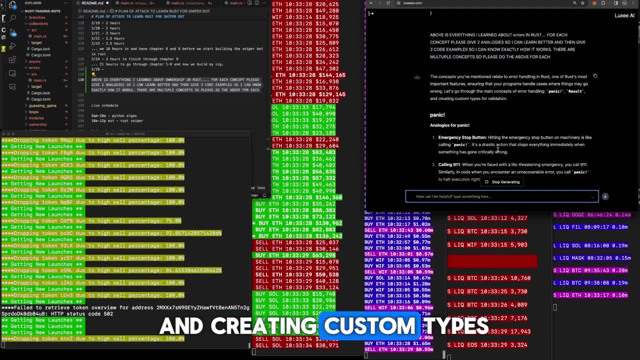 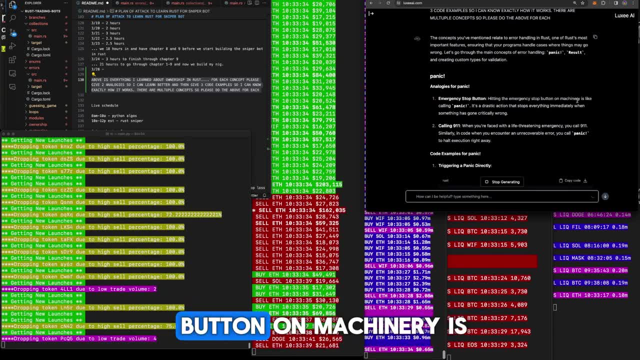 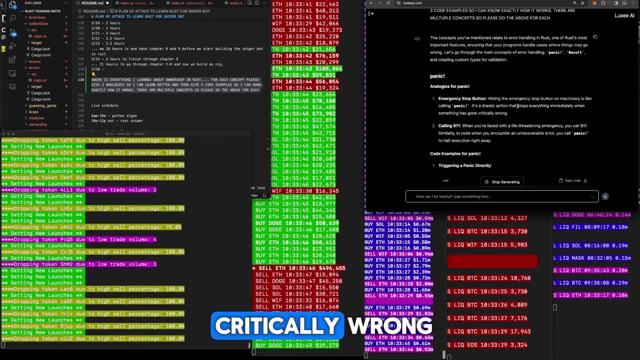 panic and result and creating custom types of for validation. so panic analogies for panic. emergency stop button: hitting the emergency stop button on machinery is like calling panic. it's a drastic action that stops everything immediately when something has gone critically wrong, calling 9-1-1. when you're faced with a life-threatening emergency, you call 9-1-1. 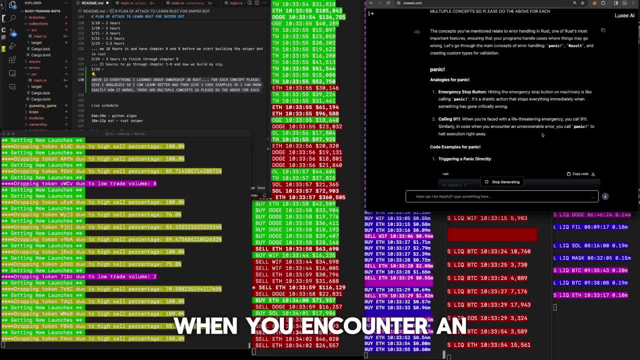 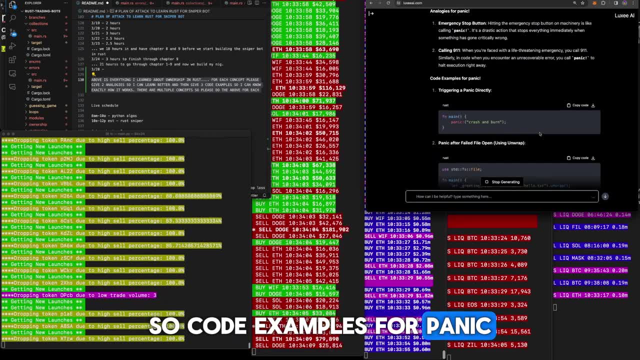 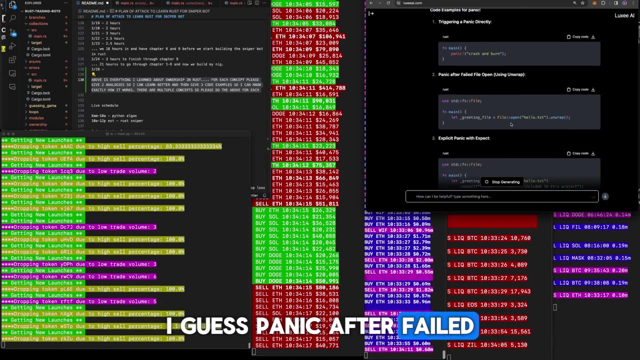 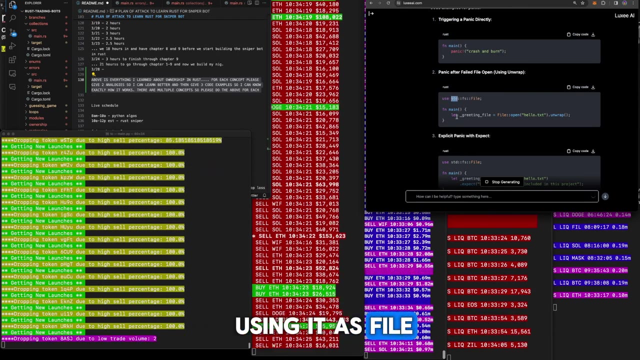 similarly in code: when you encounter an unrecoverable error you call panic to halt execution right away. so code examples for panic: triggering a panic directly so you can say you can just have a panic being triggered, i guess panic after failed file open using unwrap. so you can see, here we're importing, this is how you import stuff and we're using it as file and 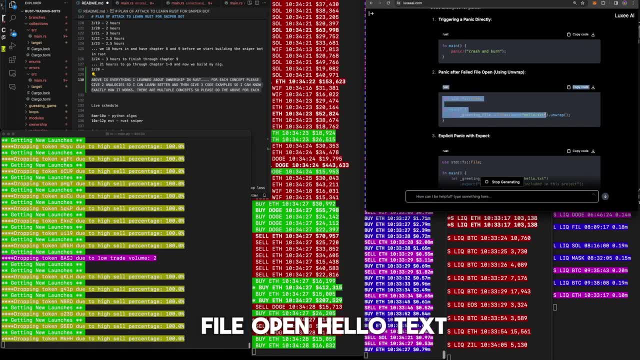 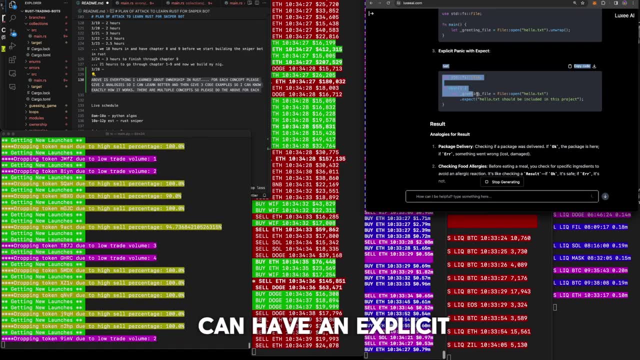 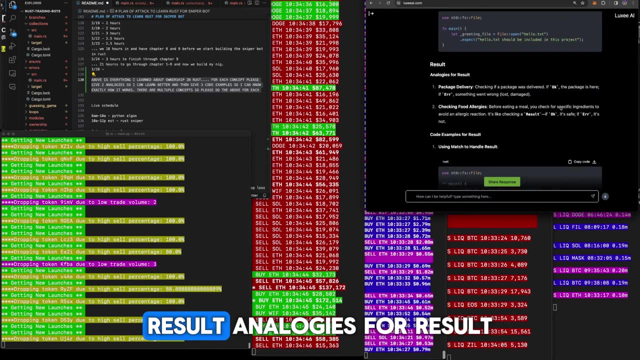 you can say like greeting, this is a function file, open hello text. if that fails then it will explicit panic with expect. so it looks like you can have an explicit panic here saying dot, expect. hello text should be included in this project. result analogies for result: package delivery: checking if a package was delivered. if, okay. 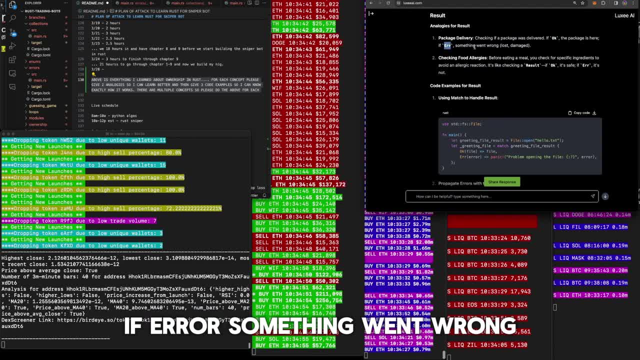 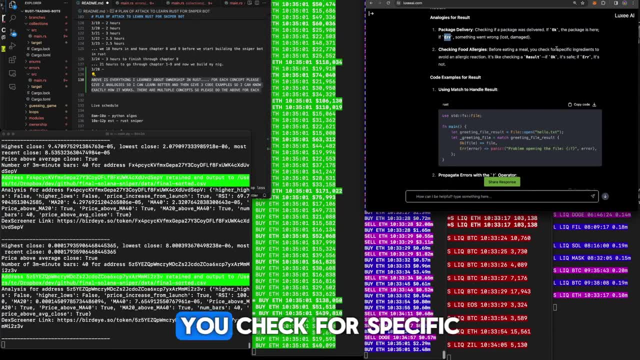 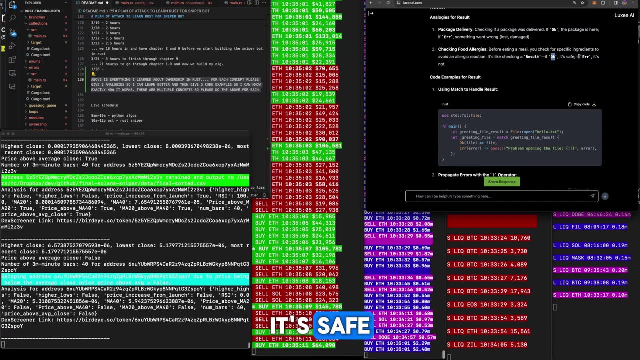 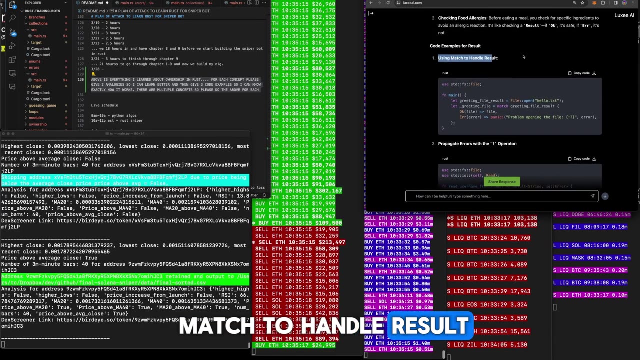 the package is here. if error, something went wrong, loss or damage. so checking food allergies is another analogy. before eating a meal you check for specific ingredients to avoid an allergic reaction. it's like checking a result: if, okay, it's safe. if it's not, code examples for rust using match to handle result so you can see we're bringing in file here. 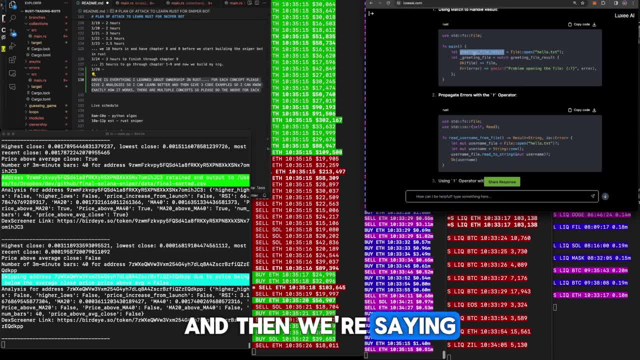 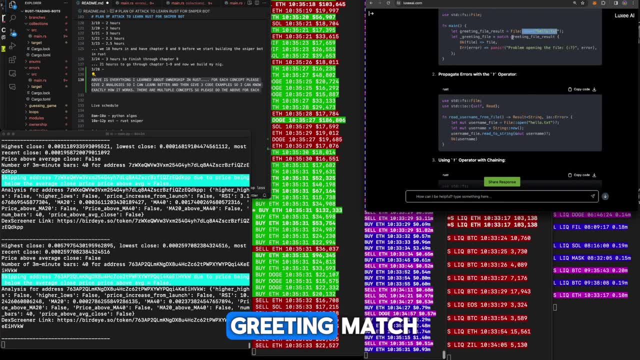 and we're naming it file and then we're saying a function here, and then we're saying a variable and saying file open. so using whatever this means, and it opens the file and then let greeting match. so we're checking: does it match? does it match? okay, then it's just file. if it matches the error, then 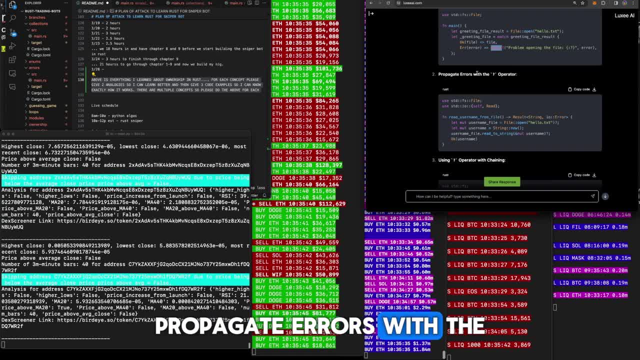 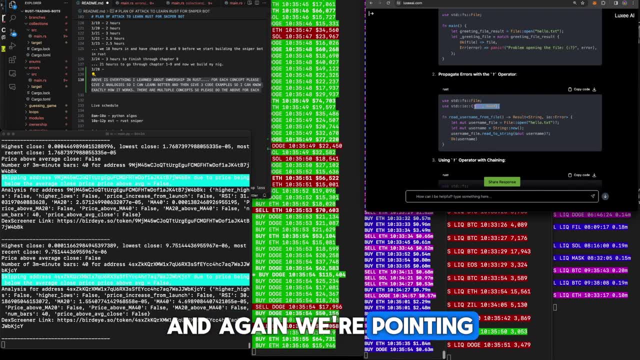 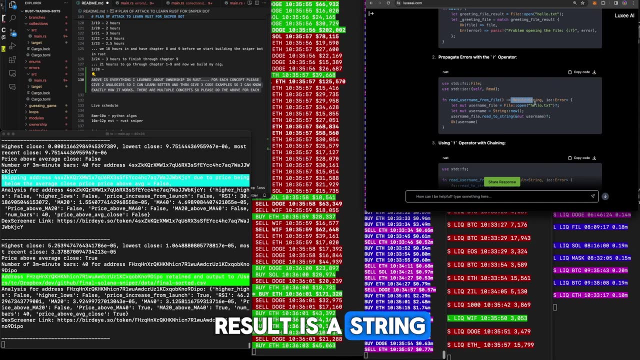 we're going to panic. problem opening the file propagate errors with the question mark. so we're using this package here as file and again we're pulling in something here self and read. so FN read username from file. result is a string and we're importing the error thing, so mutable. 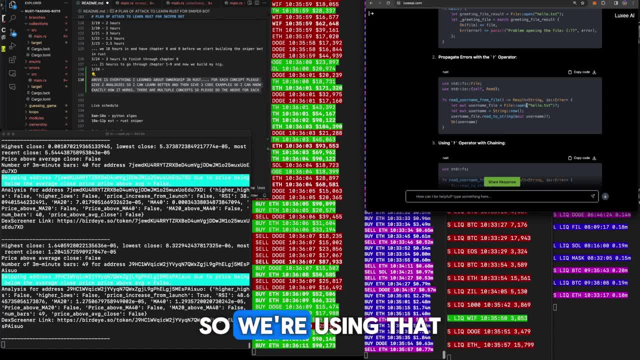 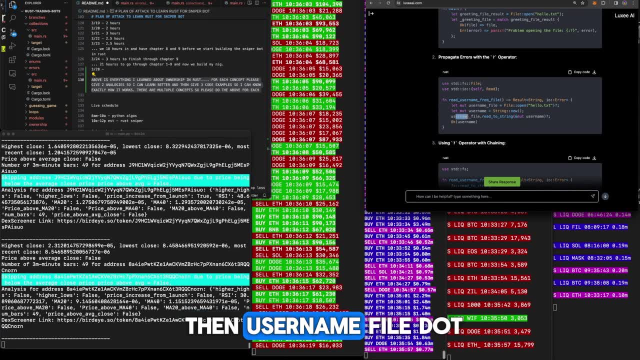 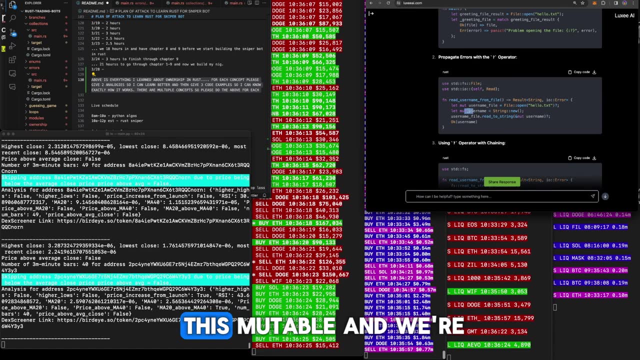 a changeable variable username file open. so we're using that file up here to open this hello text here and then we're saying the username is a string, a new string, and then username file and file read string and username. so we're passing in: there's mutable and we're borrowing it here and 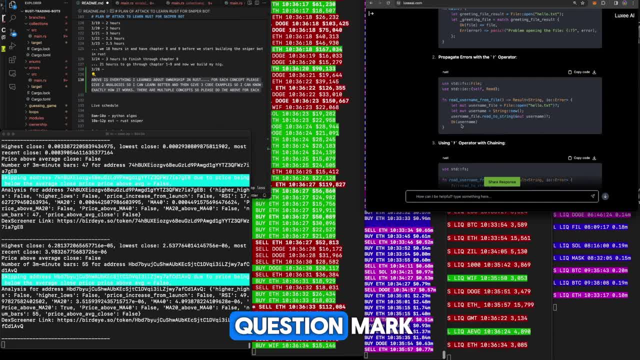 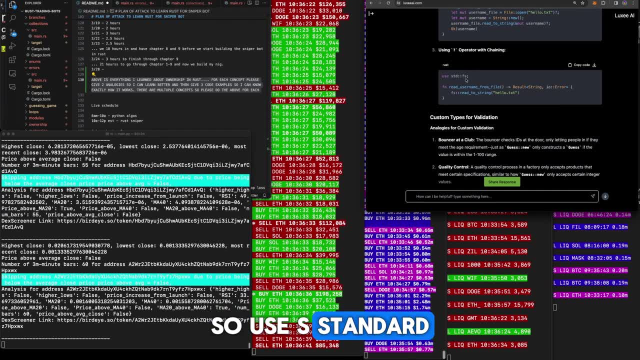 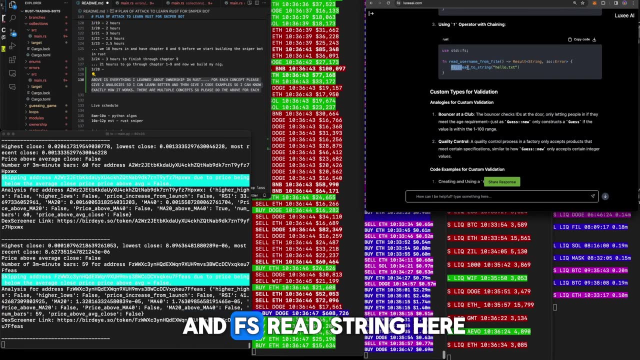 then the question mark means propagate errors. so if there's a question mark- I'm not quite sure about that- using Question mark operator with chaining. so use as standard FFs. FN is results of the string or an error and FS read string here. read to string: hello. 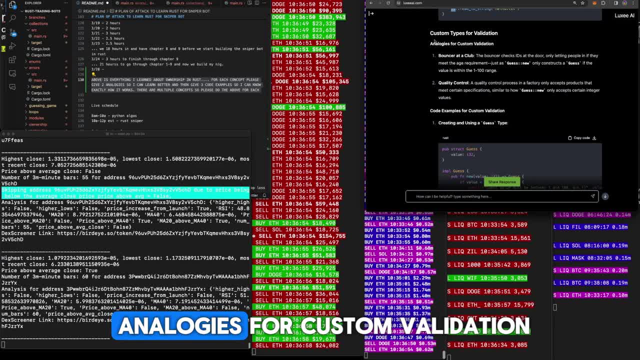 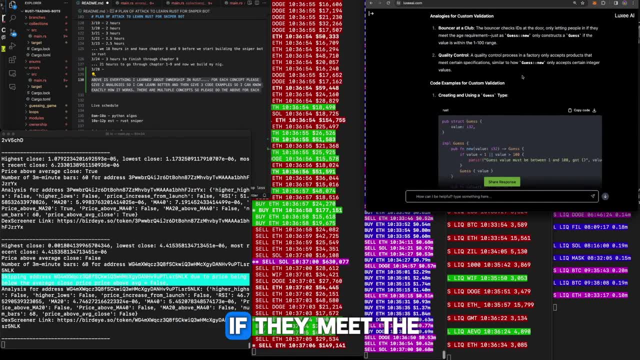 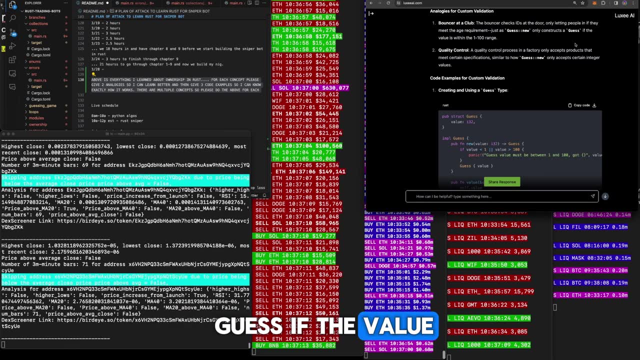 custom types for validation. analogies for custom validation: bouncer at a club. the bouncer checks ids at the door, only letting people in if they meet the age requirement, just as guest new only constructs a guess if the value is within one to a hundred. a quality control process in a factory: 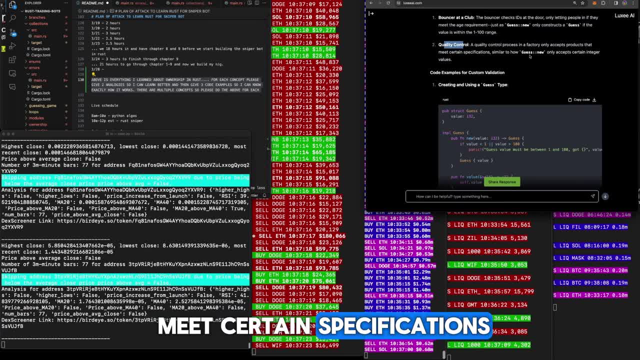 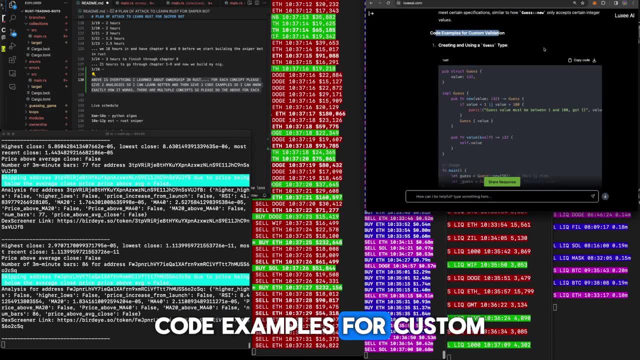 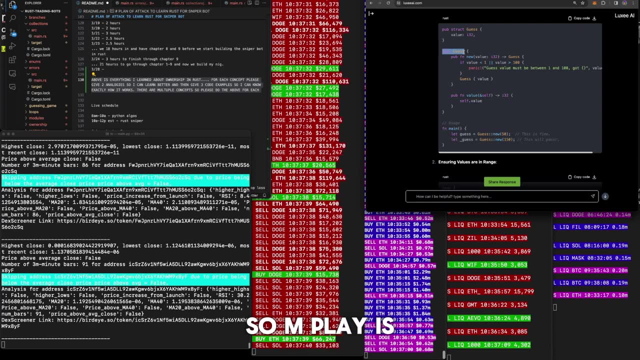 only accepts products that meet certain specifications, similar to how guests new only accepts certain integer values. code examples for custom validation here. so we're building a struck that I 32 called guests. so M play is how you do. the protest means pub new, we create a new funk. 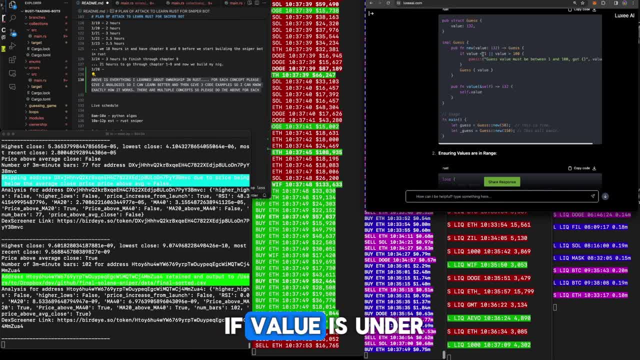 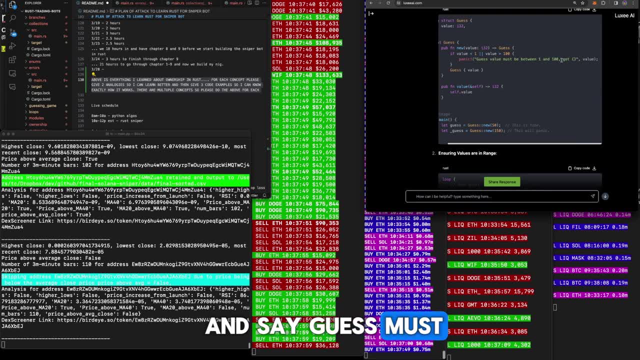 here, inside it here, and it outputs guests. if value is under one or values over a hundred, you can create a new funk here inside of here, and it outputs guess. if value is under one or values over a hundred, then it's gonna panic and say guess must be between one and a hundred and it got this value. so value is. 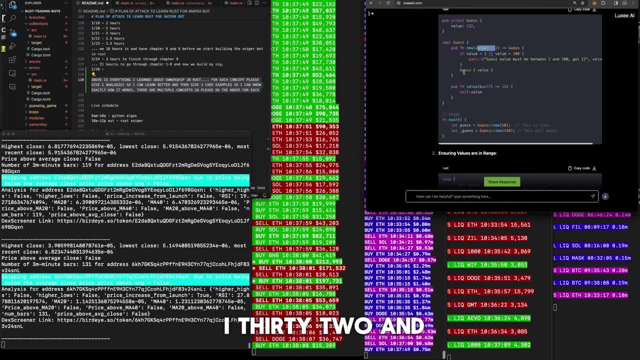 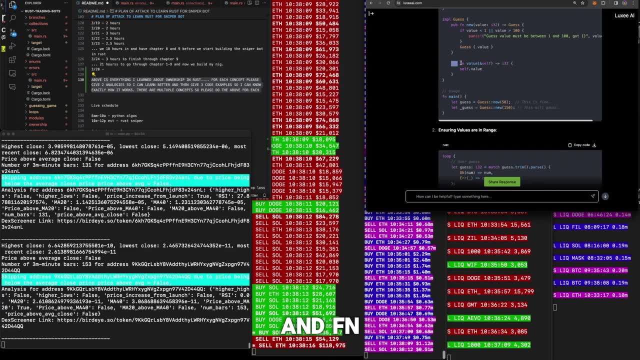 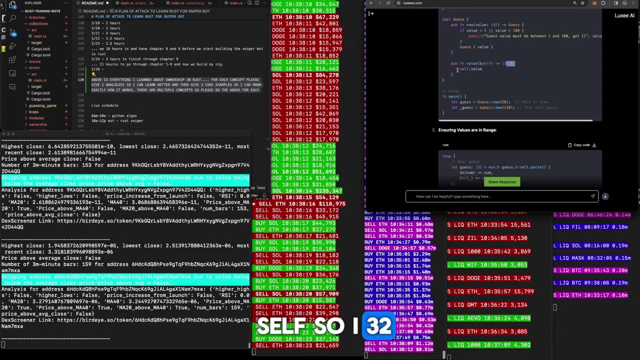 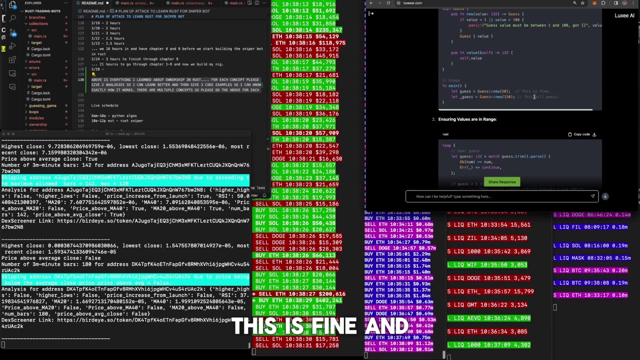 here values passed in as I 32 and then guess value. if that's not true, guess is value, so pub and FN, so value is here and s3 and self, so I 32 and then self dot value. so usage here is the FN like guess, equal, guess, new. this is fine and this will panic because 50 is in between one and a hundred. so 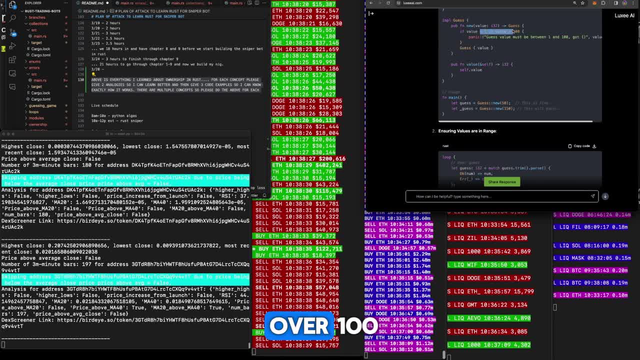 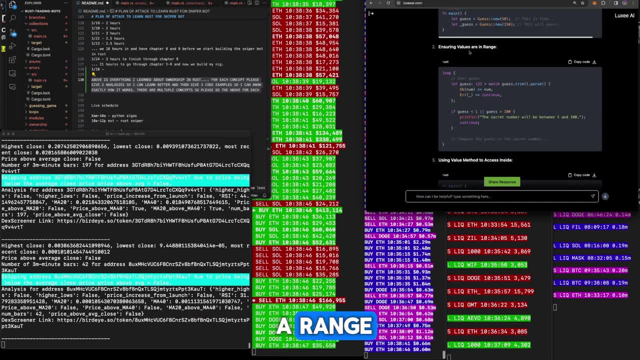 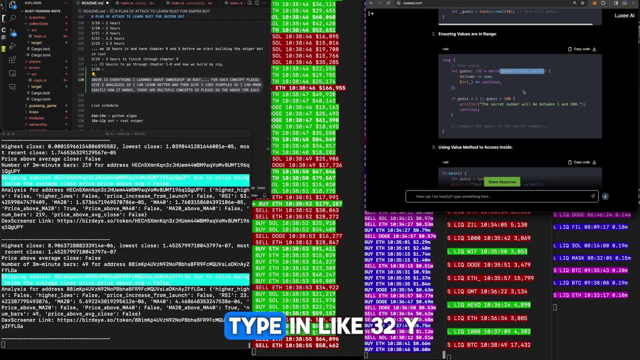 it's not going in there. but 150 is over a hundred so it's going to panic and panicking essentially just kills your program ensuring values are in a range. so we could say, let guess I 32 match. it's trimming it so it's taking away any numbers. if I were to type in, like 32, why it would take away the. 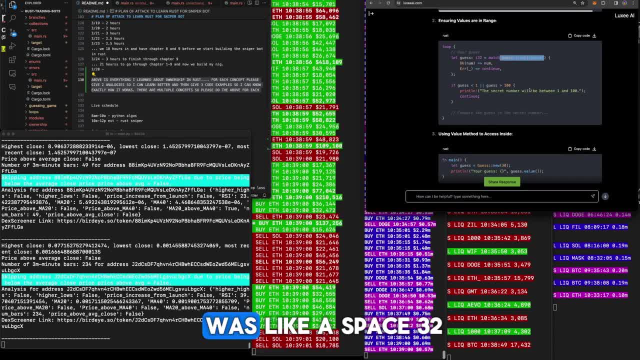 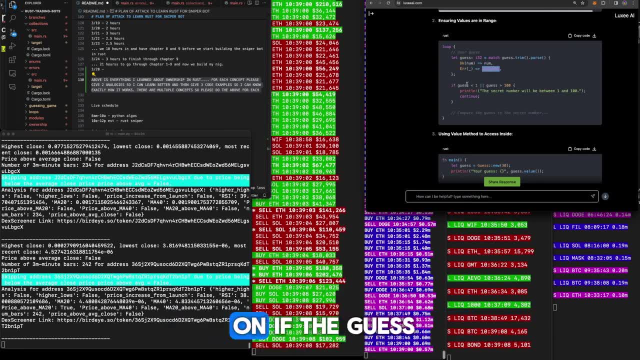 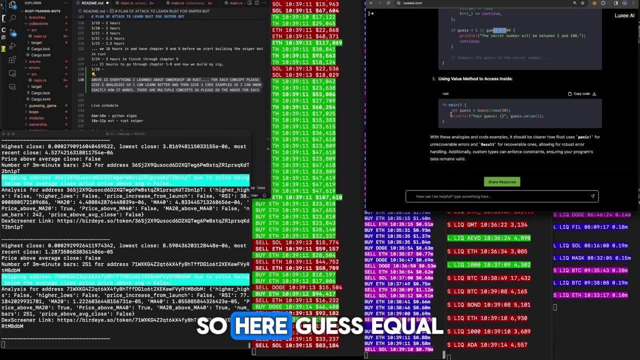 wire or whatever, or maybe if it was like a space, 32, and then it checks to see if it's a number. if it is, it returns a number, if not, it's just going to continue on if the guess is under one same thing here, so using value method to access inside. so here guess equal, guess new and pass into 30 and then 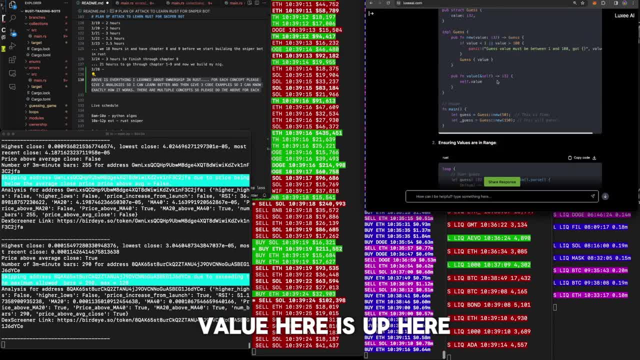 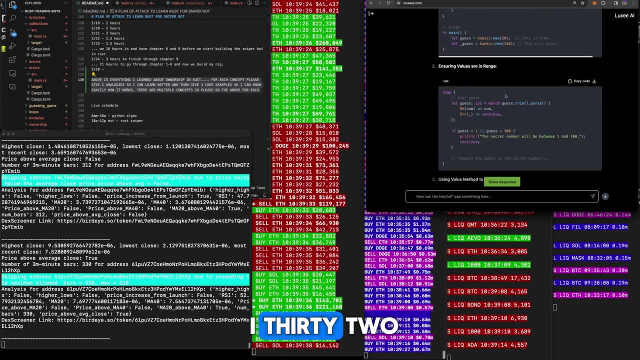 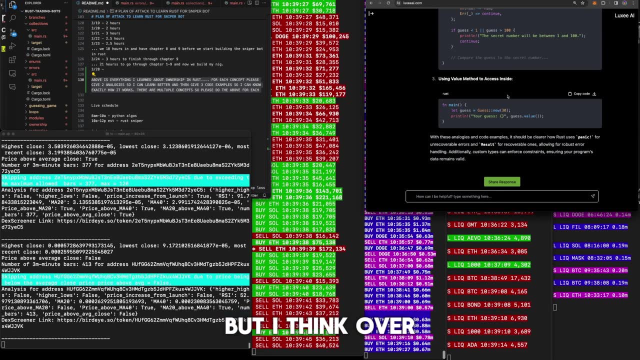 your guess is 30 and the guess value value here is up here and we're passing in value but we're not passing anything in but it's going to output I 32.. so this is tricky stuff and I honestly do not fully comprehend everything. but I think over. 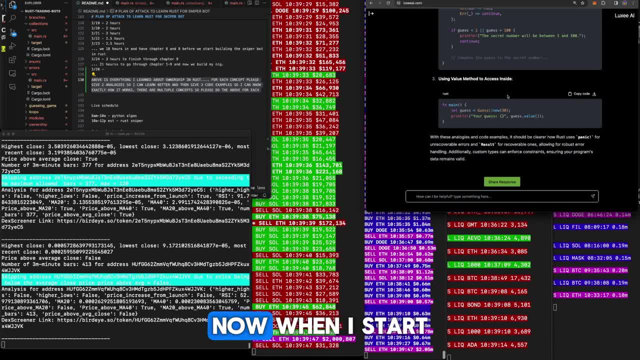 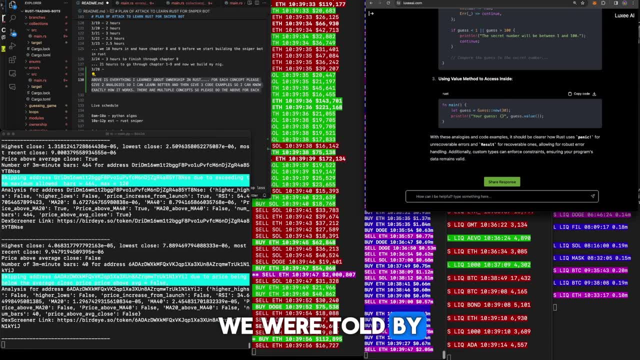 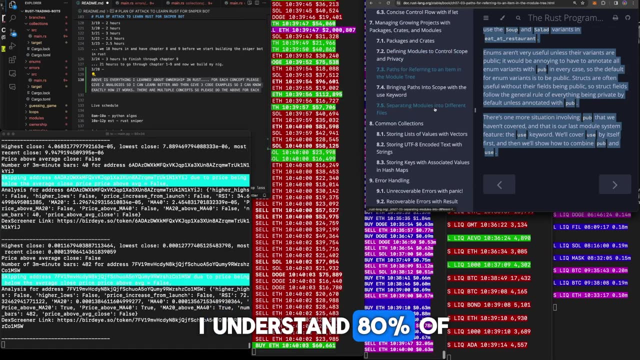 time, since we've now seen it two or three times. now, when I start implementing it, I'm really going to accelerate. I feel like from chapter one through nine, we were told by one of our homies here that that is, that's all we really need in order to start learning, and I would say I understand 80. 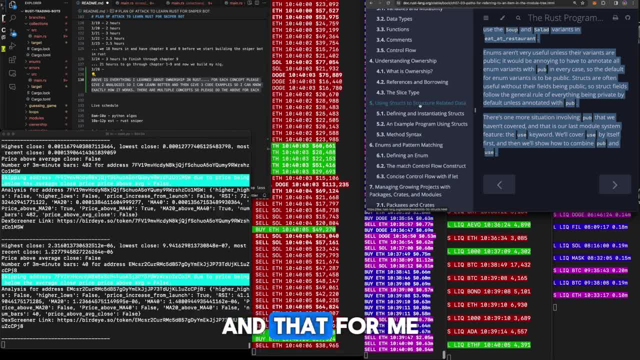 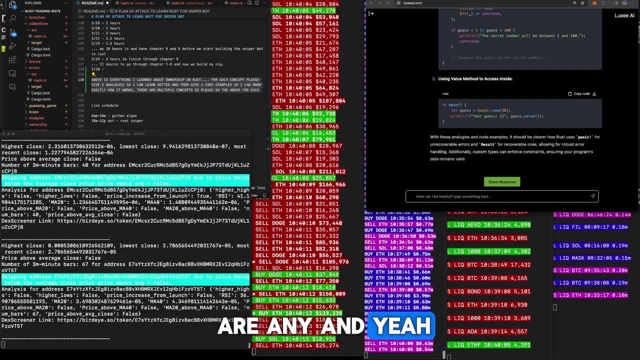 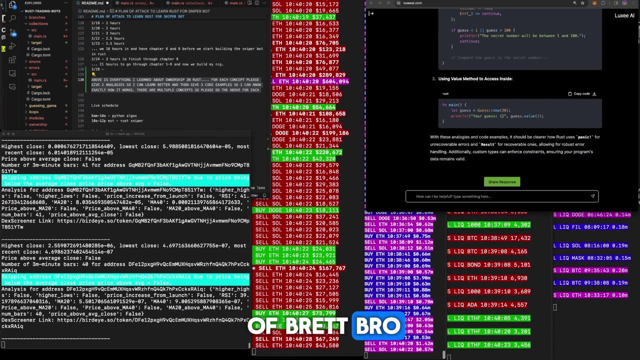 percent of the concepts in one through nine, and that for me is plenty to get going and start coding. so let me answer any questions, if there are any. and um, yeah, this has been good, so let's see here, let me answer any questions here. what do you think of Brett bro? uh, I think that's a. 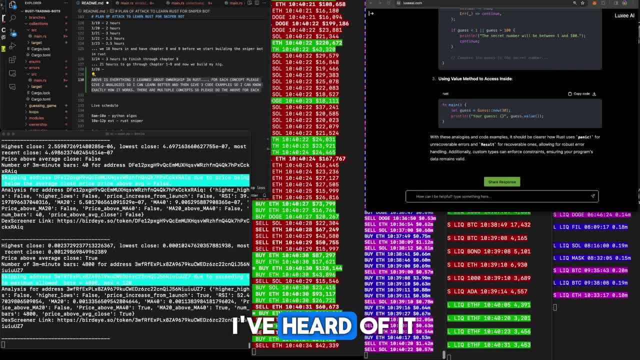 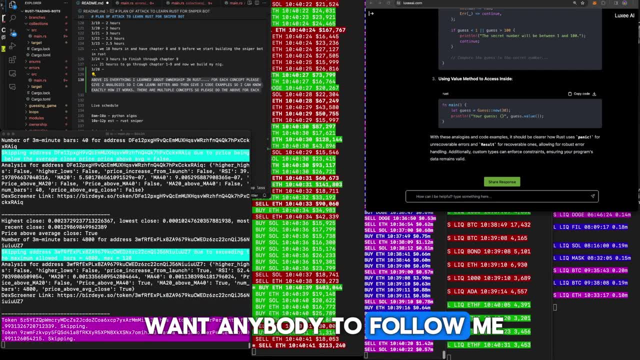 base token you're talking about? I have no idea, I've heard of it and seems cool, but I try not to give inputs on what I think about stuff, just because I don't want anybody to follow me. and so, um, Flippo says, don't want to say, but I do, like Mac. 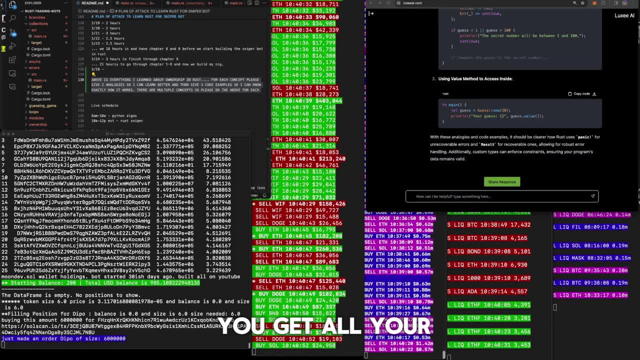 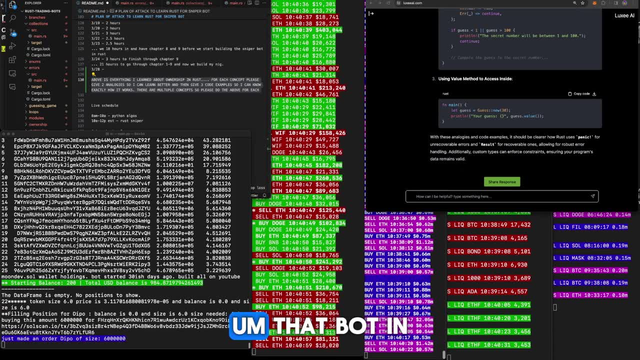 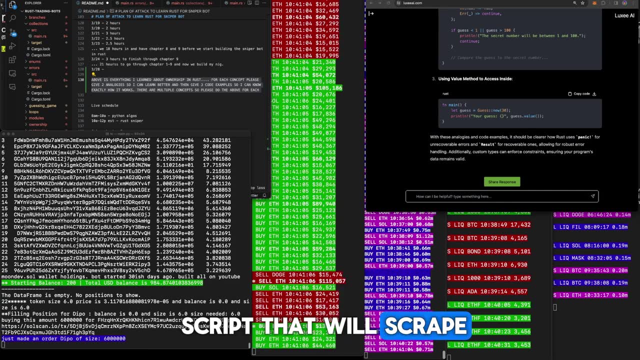 me too. dude I bear says: where do you get all your historical data from? I know there's a bot in Discord, but was wondering what other sources you use um that bot in Discord is what I use. um. if I can't find the token on that bot, I have a little script that will scrape hyper liquid. 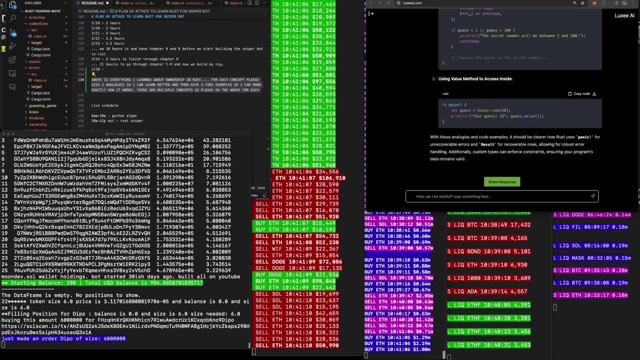 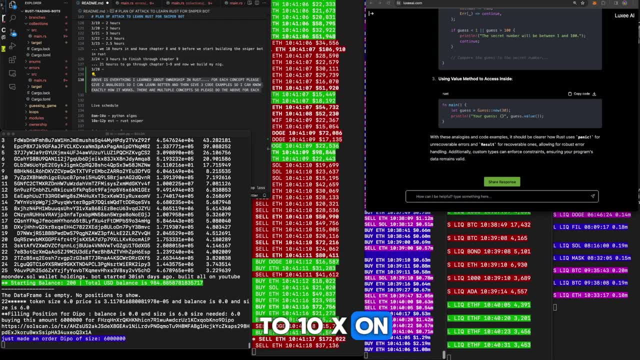 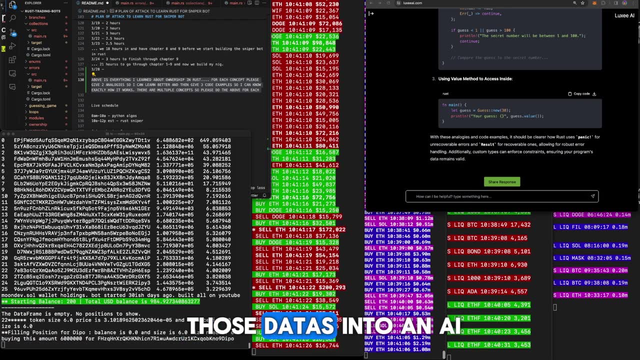 because they have more, uh, degenerate tokens. I guess awesome video says. here's an idea for me: how about one find all the previous winners that did five to 10x on those meme coins and feed those data- sentiment, vibe score, price movement, wallet ratio, Etc- feed those datas. 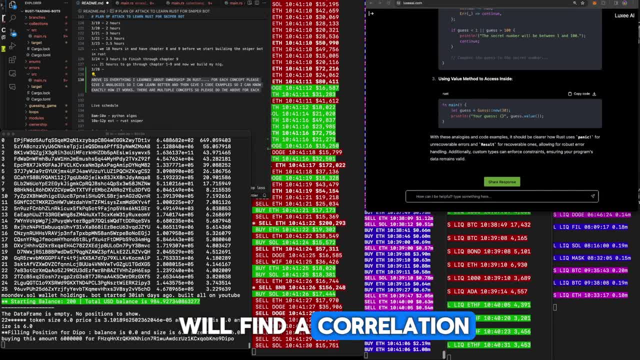 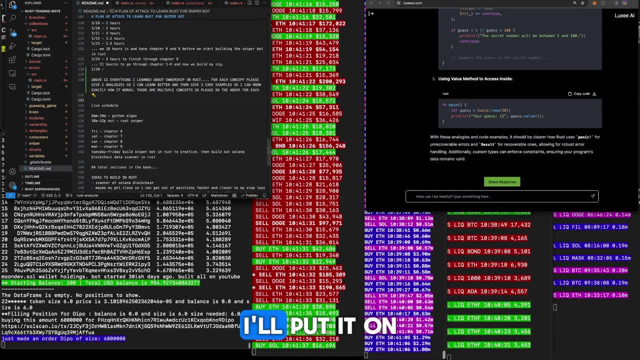 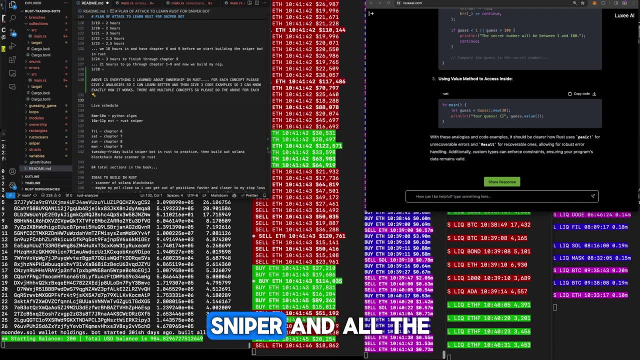 into an AI and let's see if it will find a correlation chip between winners and losers so we can use it as a filter. really good idea, dude. thank you for sharing that with me. I'll put it on my note sheet here at the bottom feed. and winners of Solana sniper and all the features. 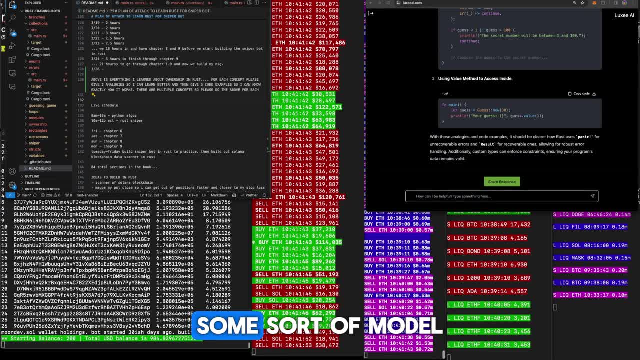 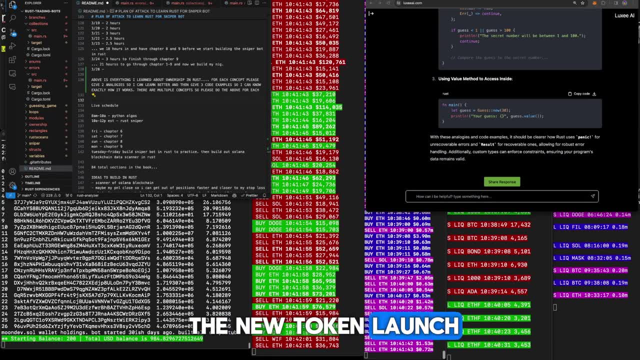 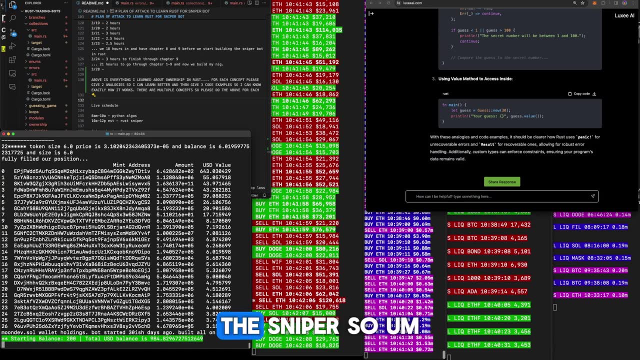 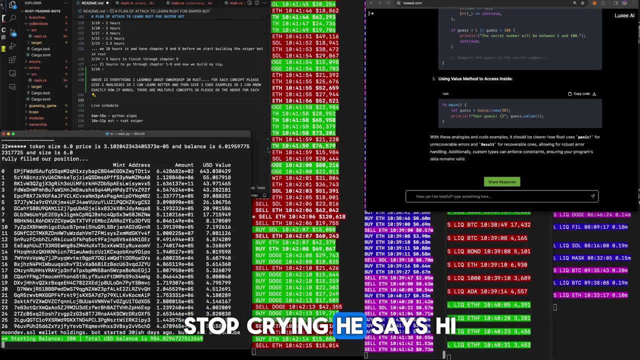 to ML and build some sort of model that can predict if the new token launch is legit. so the reason I'm learning rust is because this is doing well for me, the sniper. so, um, these ideas are welcome. thank you so much for sharing that with me. dude, stop Cron, he says hi how. 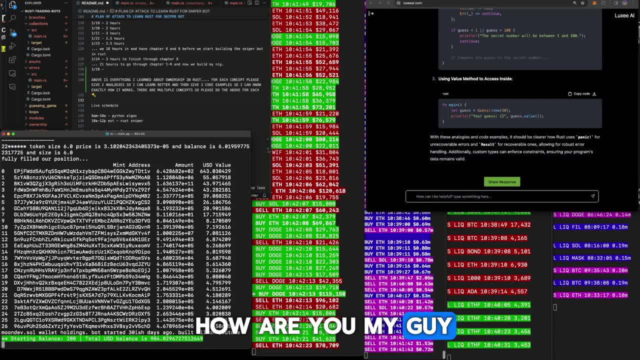 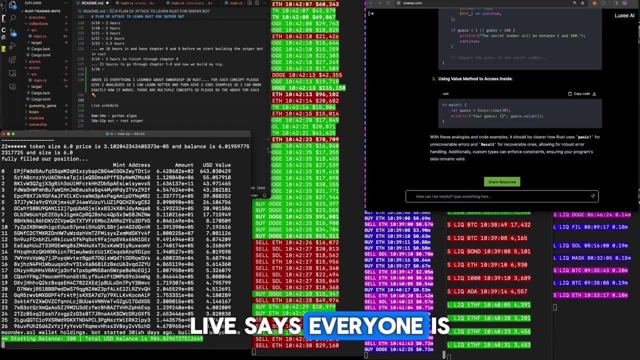 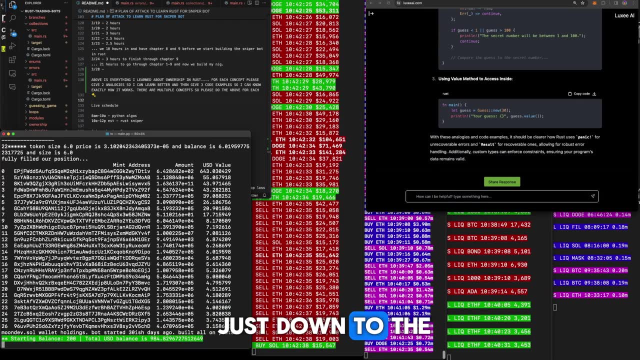 are you doing, mate? I'm doing good, bro. how are you, my guy? it's good to see you back. good to see you back every day at 8 am. live says everyone is looking at indicators and variables in the underlying data, but memes have Moon just down to the name. cat, for instance, with hat. yeah, it's tough. 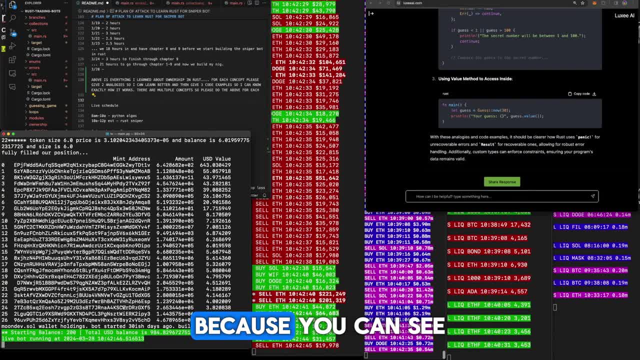 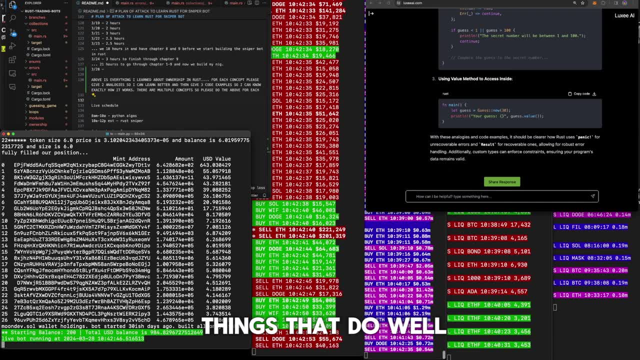 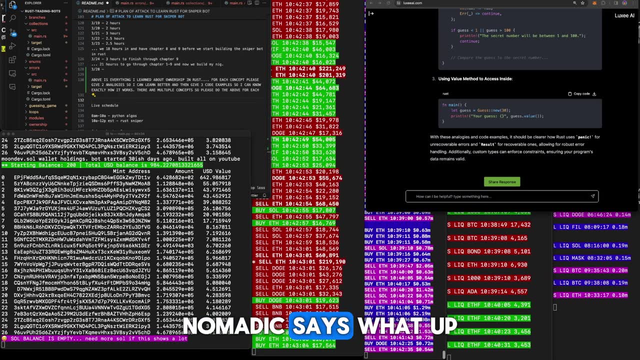 I mean, I think the looking at the numbers is good because you can see if it's trending upward and that gets rid of a lot of trash. but then you're right on man, a lot of the uh things that do well are just based off of the meme. so i just kind of call that the vibe check. nomadic says what up moon. 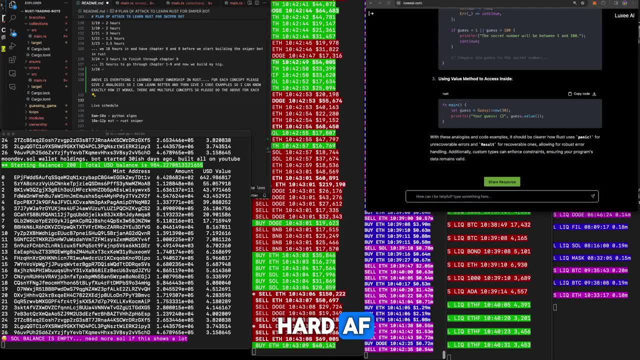 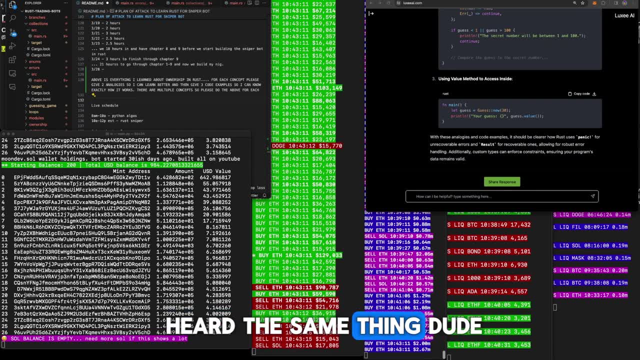 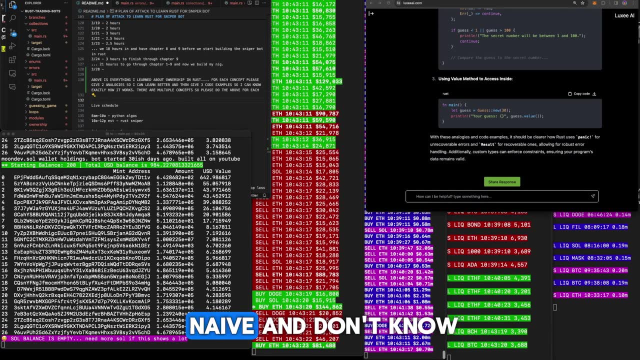 dev, i heard rust was hard af. yes, sir, it is hard, but it's actually not nearly as hard as um i thought it was going to be, because i heard the same thing dude: everybody's saying how hard rust is and how hard it is to understand the concepts. maybe i'm still just naive and don't know what's coming for. 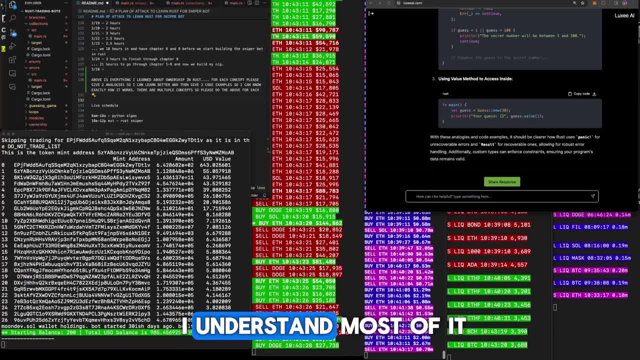 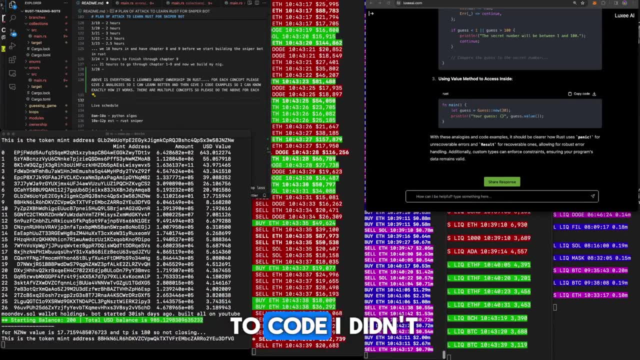 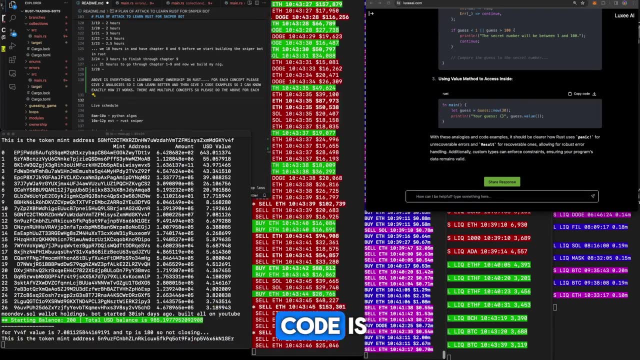 me. but uh, i read chapters one through nine and i understand most of it. market bull says: can i really learn this? absolutely, dude. i didn't know how to code. i didn't know how to do any of this stuff. i was just a dgen, like a lot of people, and, uh, the only reason i didn't know how to code is 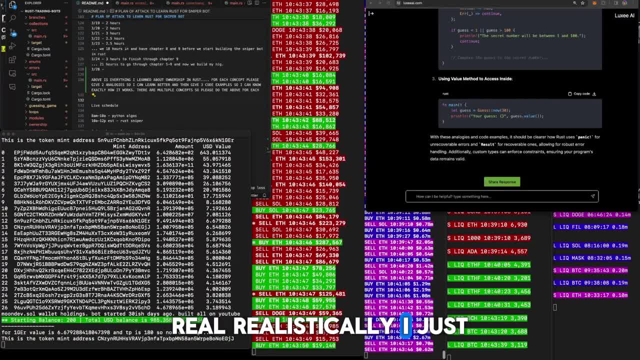 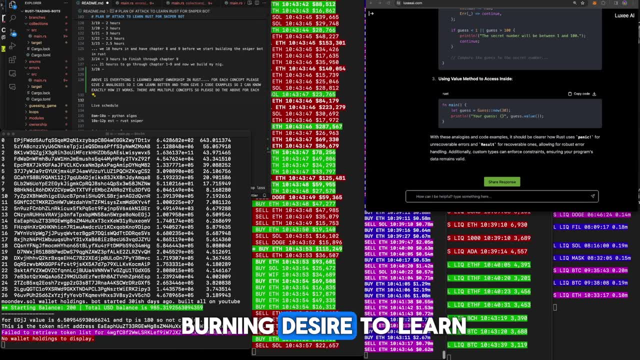 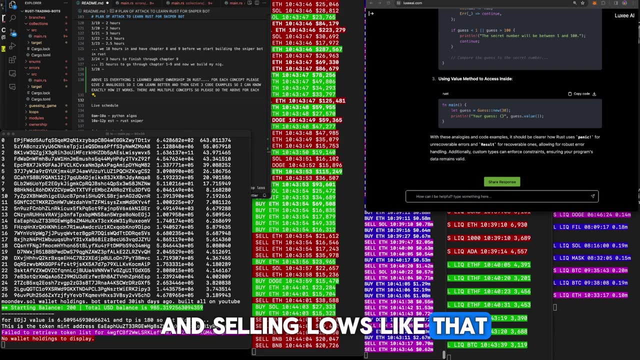 because it was a limiting belief, real, realistically, i just was like, oh, i can't code because i had to go to school for that. but once i had a burning reason, a burning desire to learn how to code, i was trading emotionally. i was chasing highs and selling lows. like that, i'll kill your account. 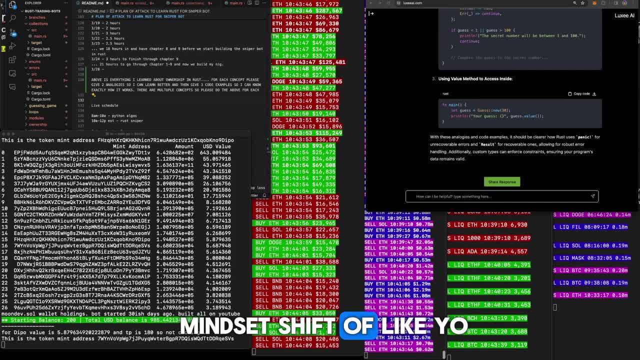 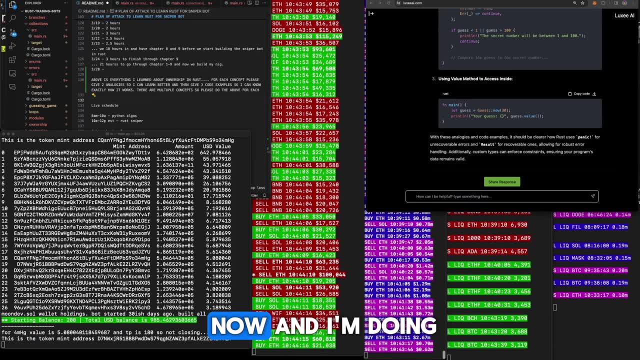 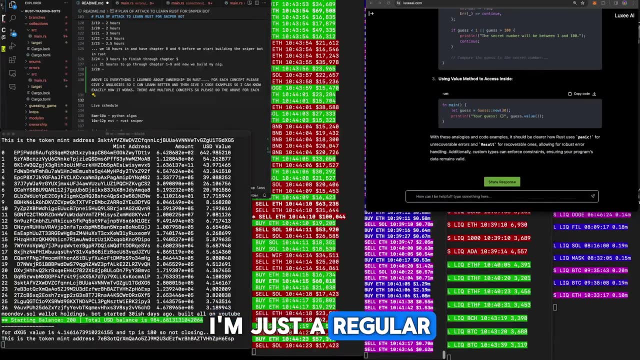 quick. so, um, once i made that mindset shift of, like yo, i can actually do this. it took me meeting somebody to have that mindset shift, but you met me now and i'm doing it and you can hear me trying to, trying to read and stuff and i trip up over words. i'm just a regular and i'll show you how. 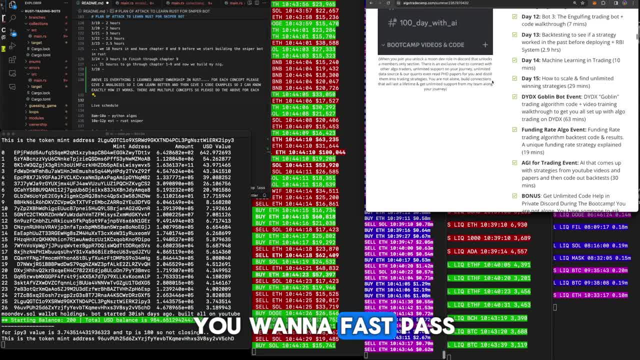 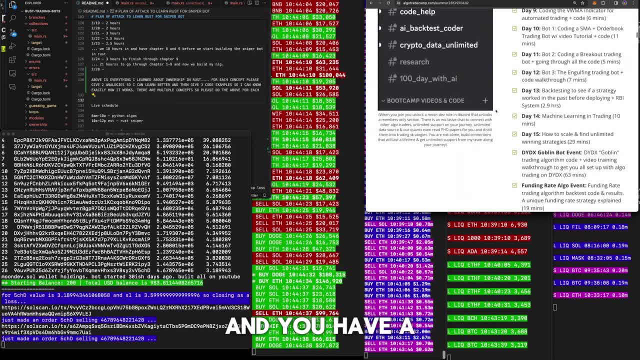 to do it here on this channel for free, or, if you want to, you want to fast pass, i can show you everything in the bootcamp. the bootcamp has everything laid out step by step, all of my code, and you have a community of us all doing this stuff here: automating our trading, backtesting, making sure things are. 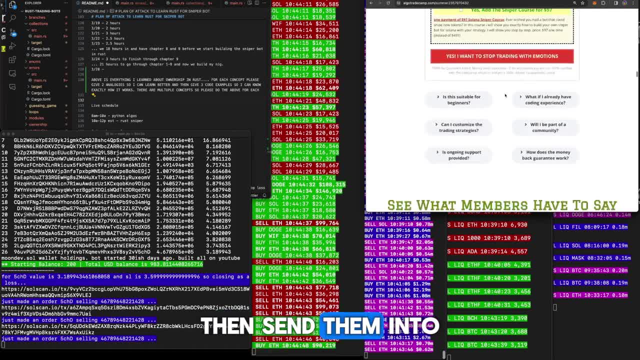 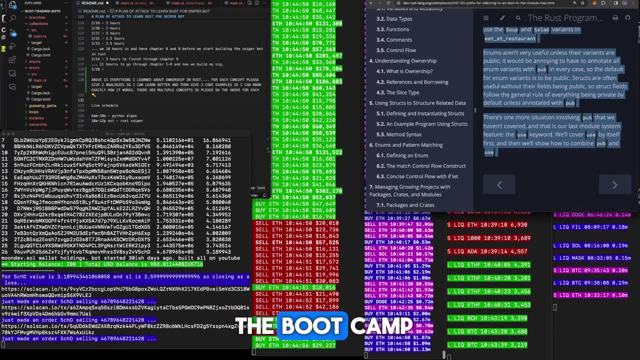 profitable in the past. that they're profitable in the past, then send them into bots. so you're going to save a lot of time and a lot of money if you join the bootcamp. but at the same time, i don't really care. if you join the bootcamp, i'm there for you pretty much 12 hours a day, if you. 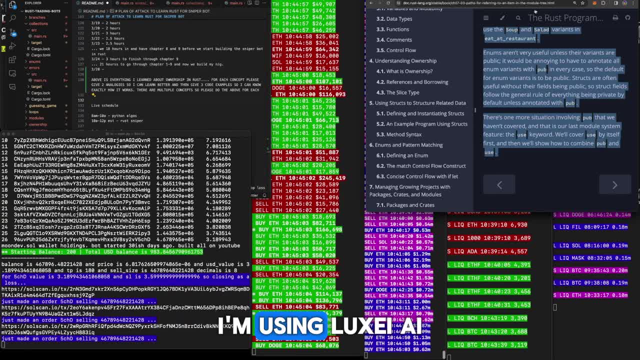 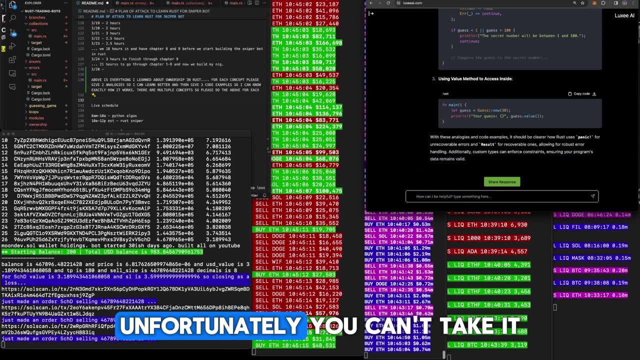 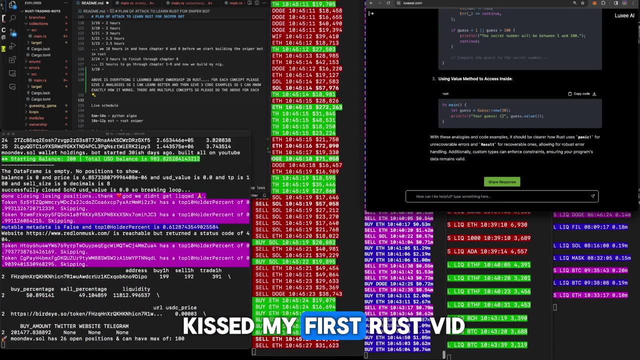 have any questions. what ai am i using? i'm going to be using the bootcamp. i'm going to be using the. i'm using luxi ai. b7r says i need this bot. how can i take it? um, unfortunately you can't take it. i'll teach you how to build your own. though ibear says he kissed my first rust vid, i think you meant. 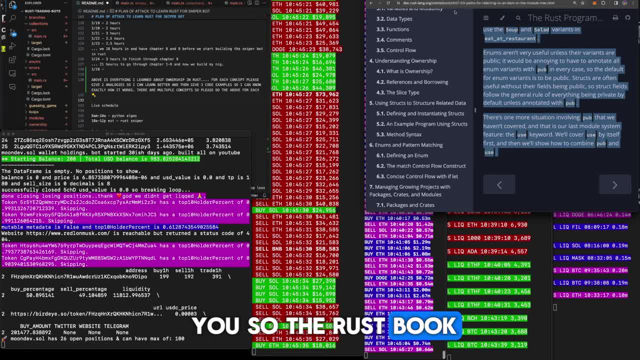 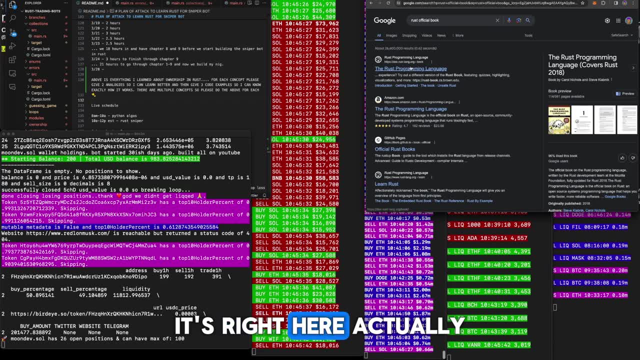 miss, but i got you, uh, so the rust book. i think you could probably just google it: rust official book. i haven't done that yet. yeah, it's right here actually. so this is the rust book that i went through. i went through choppy and i'm going to show you how to build your own bot. i'm going to 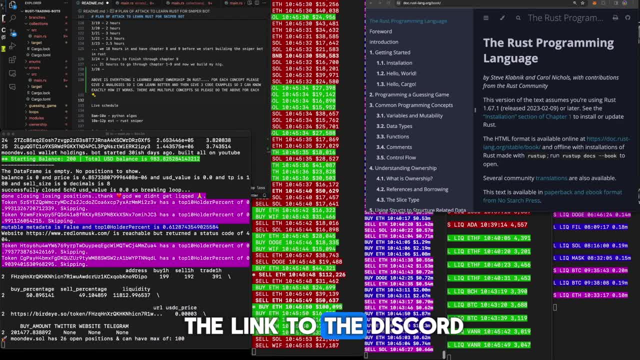 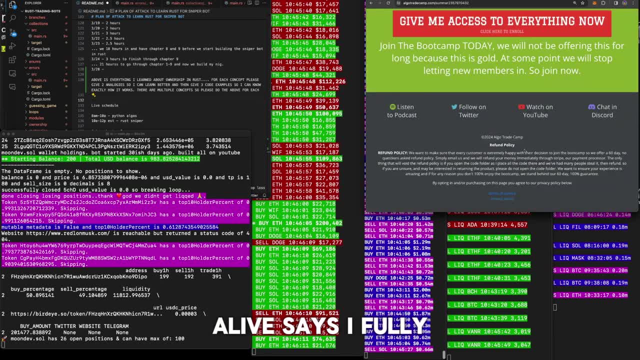 show you how to build your own bot. i'm going to show you how to build your own bot. muhammad says he wants the link to the discord. it's on the it's in the description at the very bottom of this page. here. alive says i fully respect anyone who has learned code in the past. 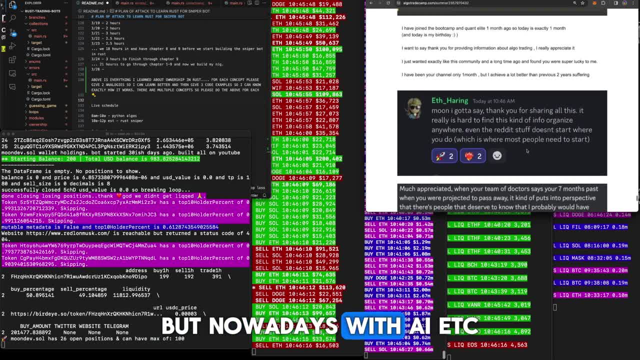 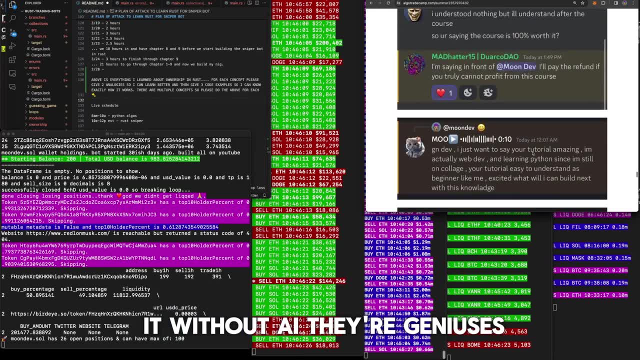 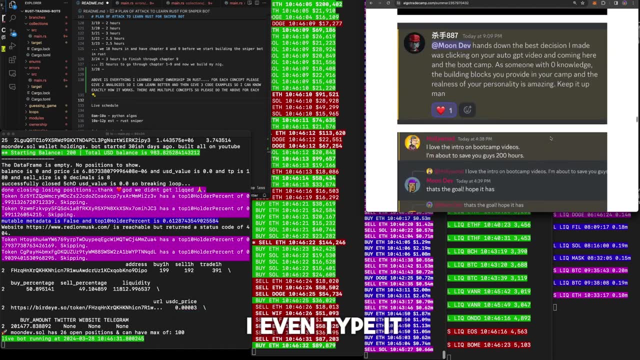 i left school with no qualification, but nowadays, with ai, etc. a different game made it much simpler to learn. it's crazy, right, those guys that learned it without ai. they're geniuses. i guess i learned it without ai, but, like now, i lean on ai a lot, because why would i even type it? you know, um guys, get your questions and get your last. 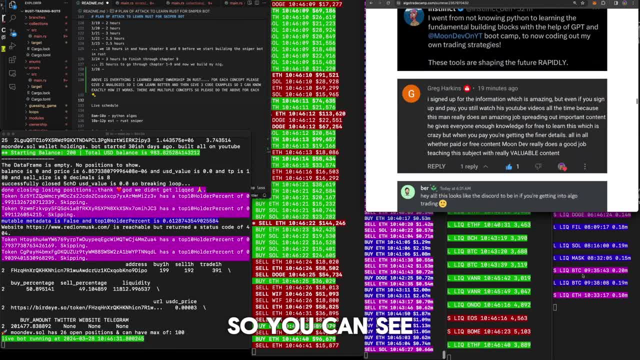 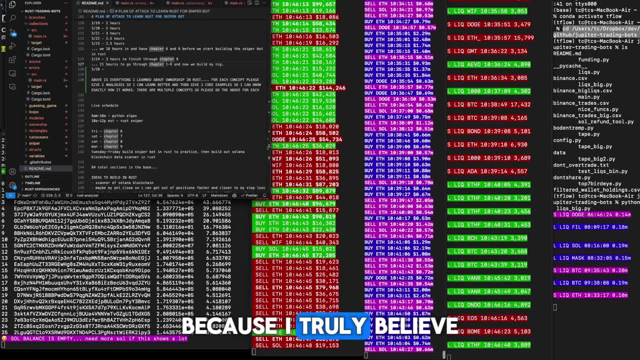 questions, and i'm gonna let the stream go for the rest of the day so you can uh see all this data. this data is super interesting to me and it's what i'm watching all day. that's why i stream it, because i truly believe if i just show you everything that i'm i'm looking at, then you know. 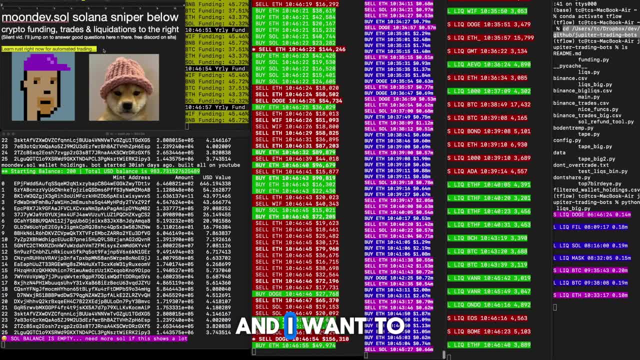 you'll be able to come up with new ideas, and i want to just really share everything along this journey, like i think it's super interesting to me and i'm going to show you how to build your own stream and see how it works. and i'm going to show you how to build your own stream and i'm going to 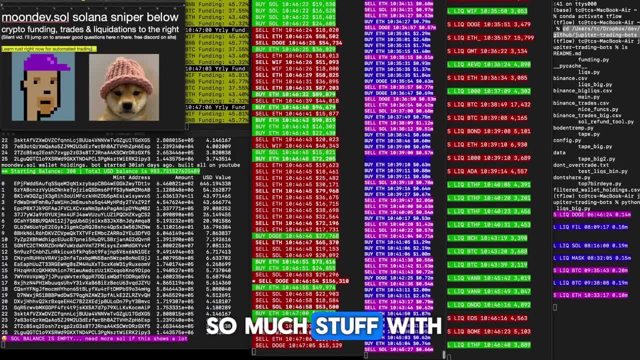 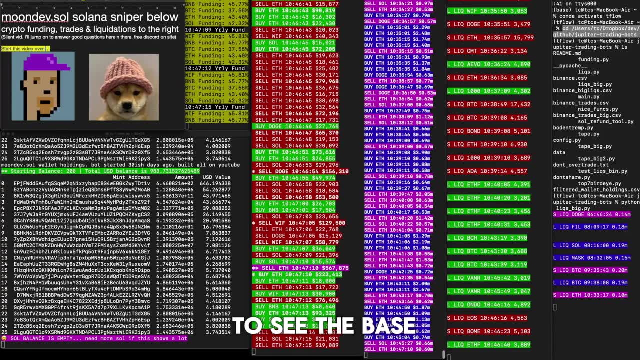 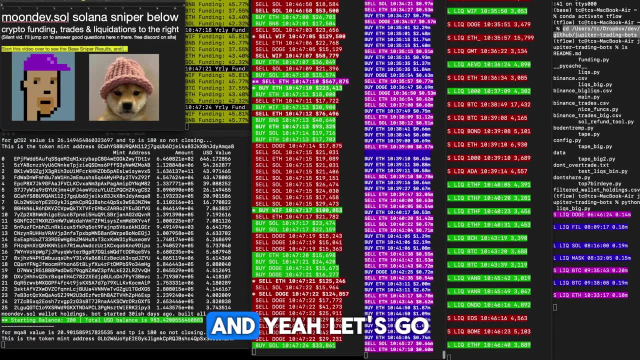 show you how to build your own stream. and i'm going to show you how to build your own stream. i love sharing it because you guys share so much stuff with me too and it's just awesome. so i'm gonna say: start this video over to see the base sniper results and 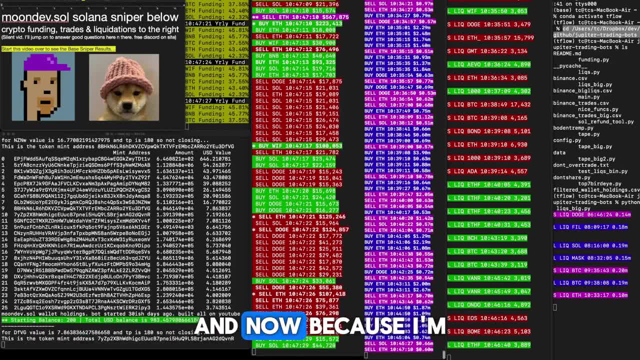 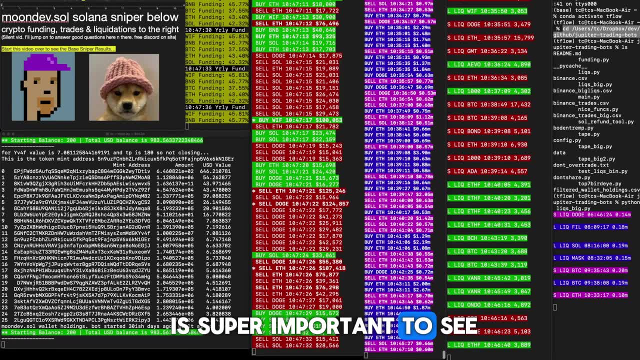 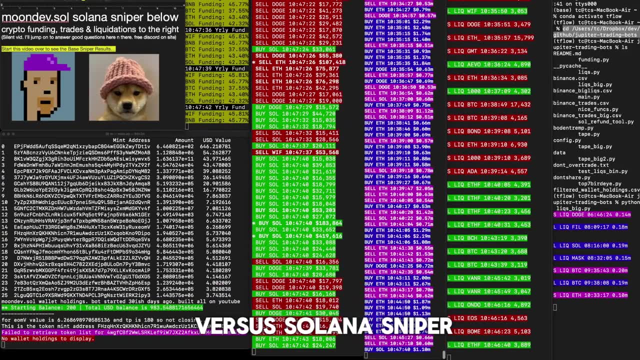 yeah, let's go ahead and switch this back. get your questions in now, because i'm about to go work out, but i'll keep the stream going because i think this is super important to see. let's say i'm changing the name base sniper versus solana sniper, and then i'm gonna change. 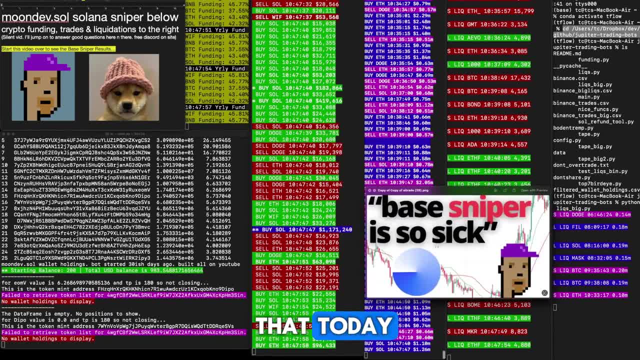 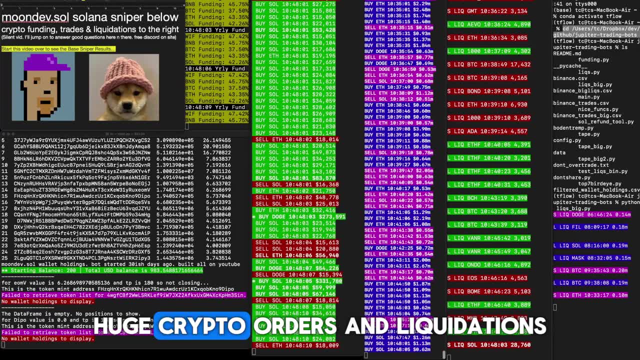 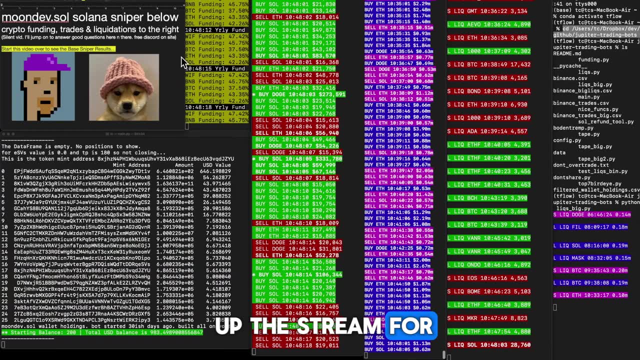 out this thumbnail again. we didn't get to that today. that's it, so i'm gonna change it back. plus, uh, huge crypto orders and liquidations. so i'm just setting up the stream for the rest of the day because i'll just let this go all day. i'll probably